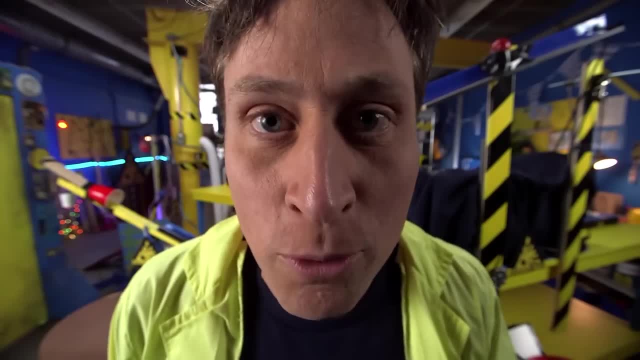 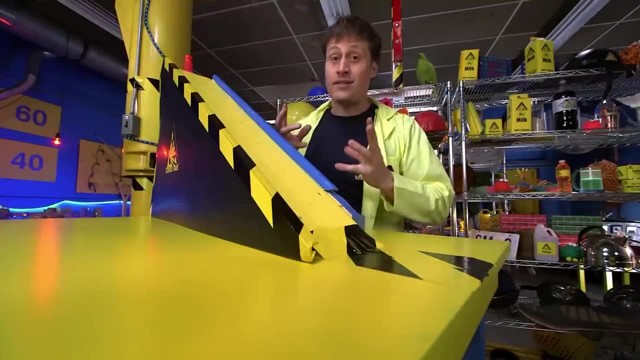 Rube Goldberg machines. Rube Goldberg machines, Rube Goldberg, you heard me say Rube Goldberg machine. Okay, we got that part, Okay, good, Rube Goldberg was a cartoon, A cartoonist who came up with the idea of having a simple task done by a machine. 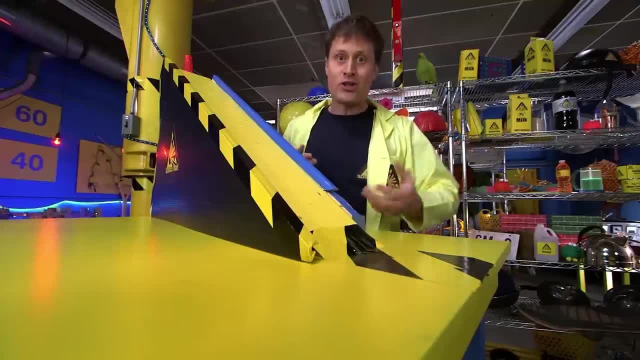 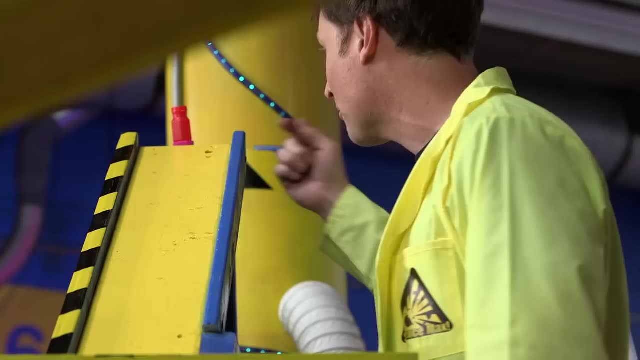 that was extremely complicated. There are Rube Goldberg competitions all over the world and there's only a few rules. First, a human can only touch it once by starting the whole thing off, and then the machine has to work all on its own. 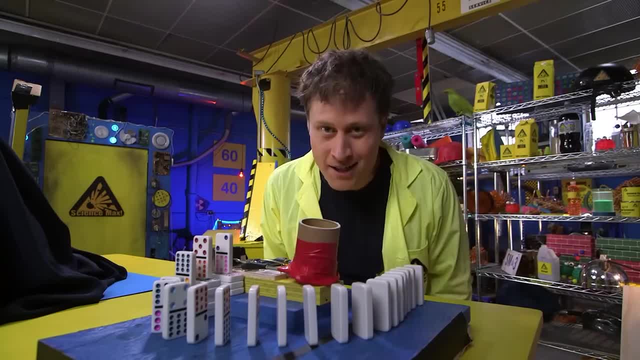 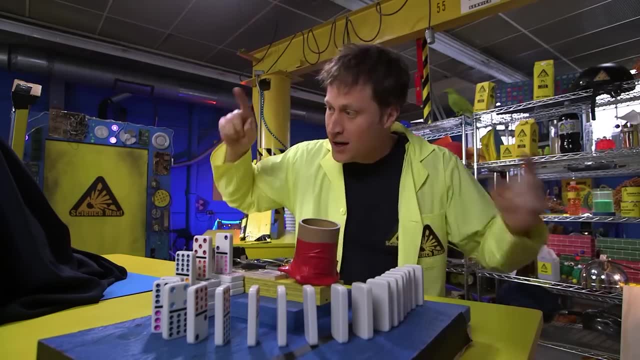 I know what you're thinking. You're thinking, Phil, what's the science behind a Rube Goldberg machine? Well, it's all about changing energy. Remember, you start the whole thing off with just a little push, but if you want the machine to keep going and going, 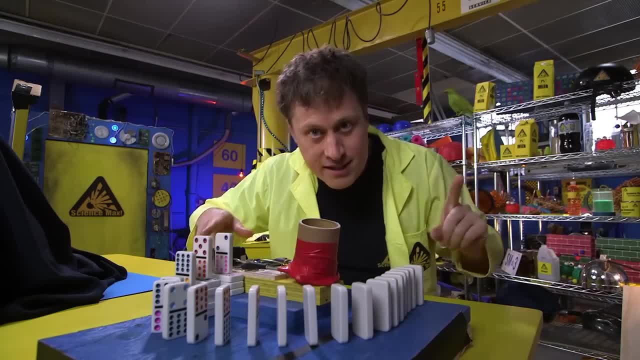 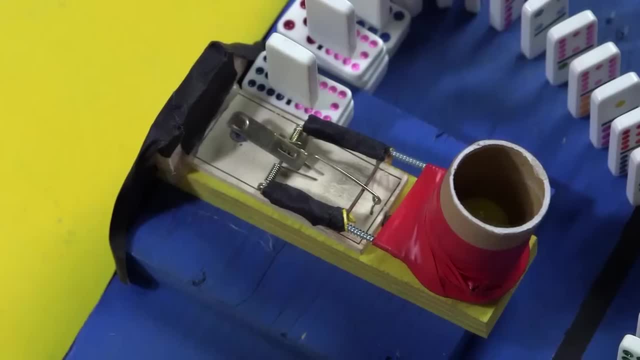 you have to come up with clever ways to add more energy to the system. so you've got more energy to keep the machine going. So check this out: A bunch of stacked dominoes, which will start a chain reaction that leads to this mousetrap. 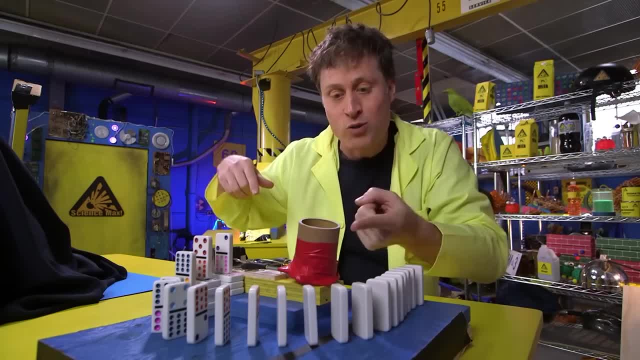 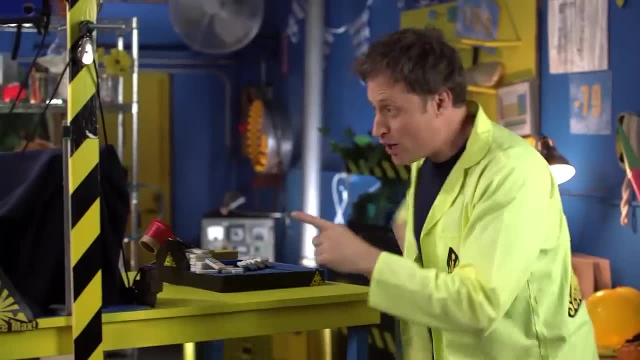 which has all of its energy stored in this spring tension which will release the ball Boing. Check this one out. It's a bunch of pulleys and there's a rope that goes up and down and up, attached to this lever where there's a ball. 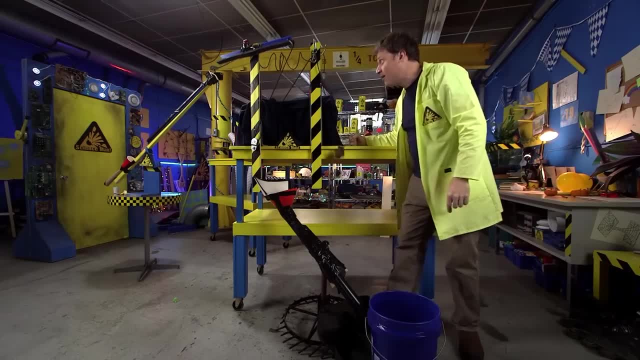 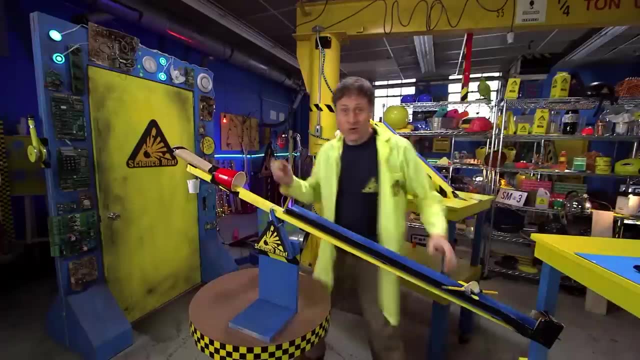 and there's a big heavy weight here, And when the weight gets knocked off the table, the ball falls into the hole and then goes down the tube and so on. Check this one out. Here's a great way to change the direction of something. 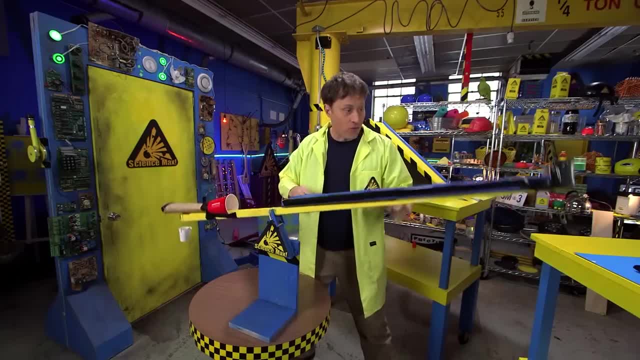 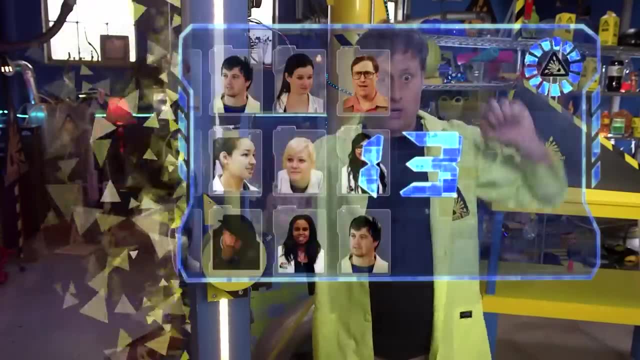 Say, the ball falls on this lever. Well, it's weighted on this end, but then the weight falls off and the ball goes this way: Ha ha And uh-oh, uh, the portal turned on. Uh, I gotta pick an expert. 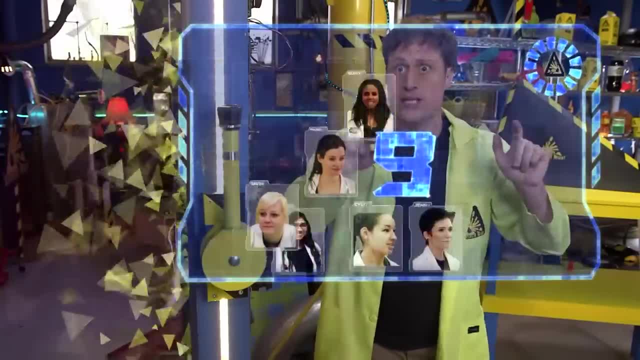 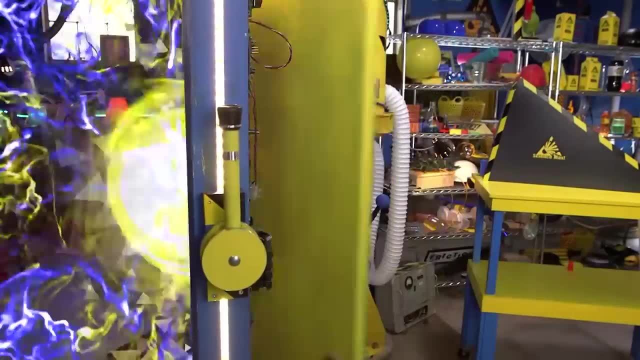 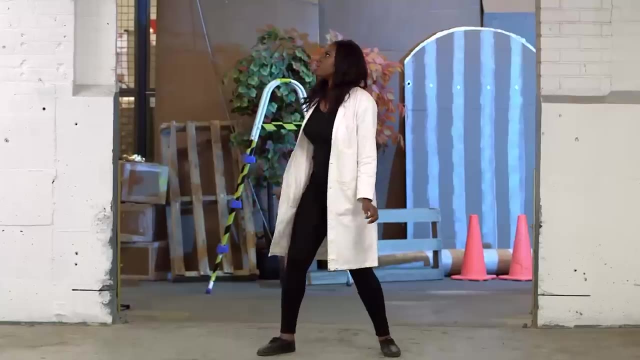 Okay, hold on a second 10 seconds before the portal resets. Ah, Sonya from the Ontario Science Center. Perfect, and there we go. Tons of time. Three, two, one Sonya. Hey, I whirled in three blocks away. 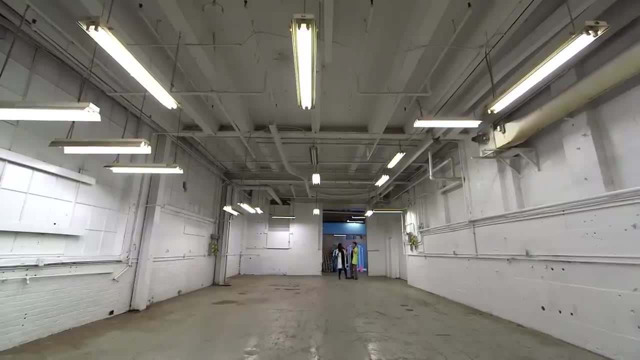 I had to run here. Okay, You're here now. Yeah, I didn't put the coordinates in when I left. anyway, It's okay. it's okay, Sonya from the Ontario Science Center. I'm glad you're here, Nice. 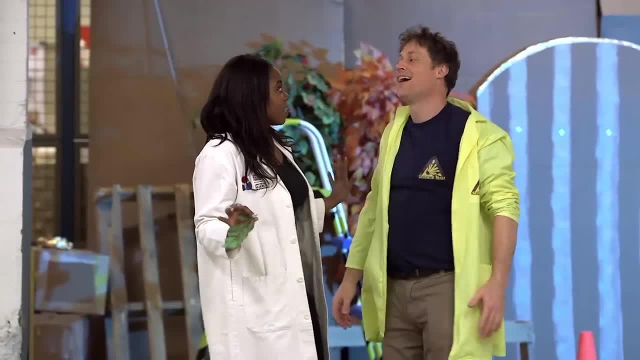 Because we are gonna build a Rube Goldberg machine. Really, Yeah, Oh my gosh, I'm so excited. Yeah, Yeah, I am excited too. Check it out. We're in a giant room. I've never done anything with it. 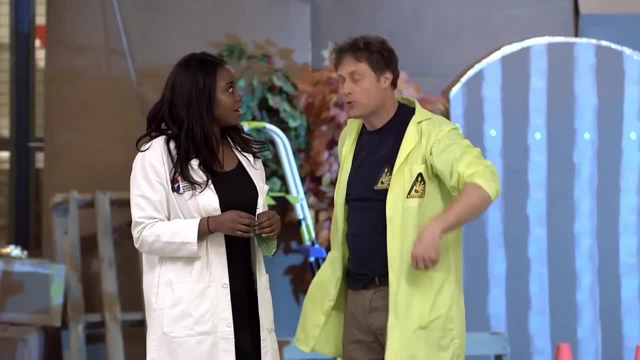 so why don't we build a giant machine in here? Why not? Okay, so here's the rules. The Rube Goldberg machine has to start with one simple thing, right? Yep, So we're gonna start with this marble and we send it on its way. 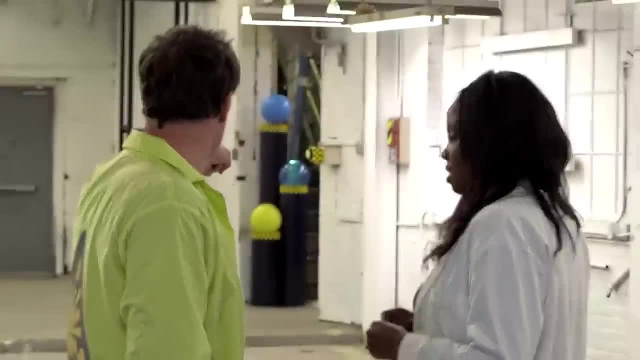 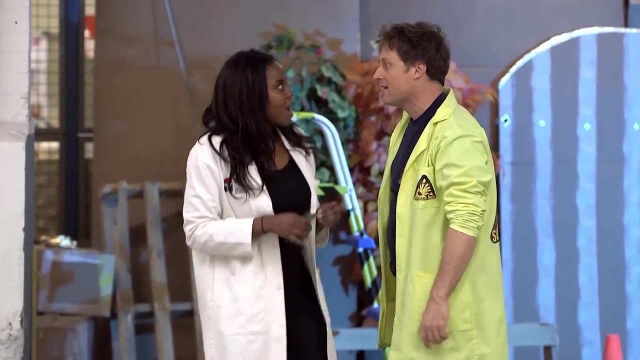 and then a whole bunch of stuff happens and at the end we press that button. That button- Yeah, What does it do? I've never used it before, but when we hit that button, we get cake Cake. A cake will portal in and we'll have cake. 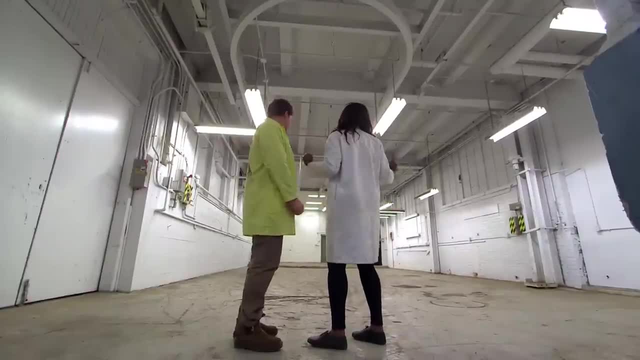 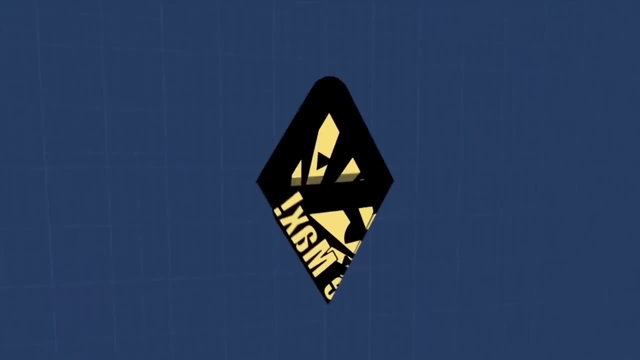 Oh, my goodness, can we get chocolate cake? We can totally have chocolate cake. All right, Now I'm really really excited. Okay, so can I start? Absolutely Great, because I saw some stuff over here. Okay, This is a pendulum. 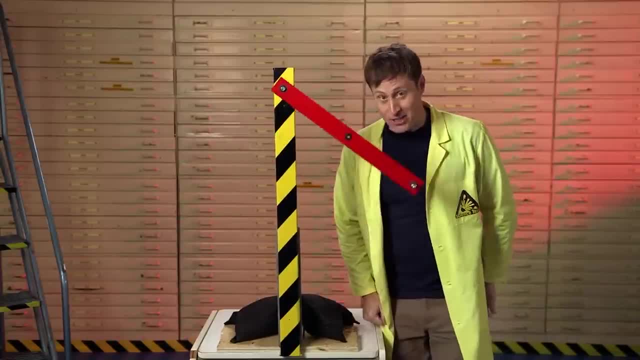 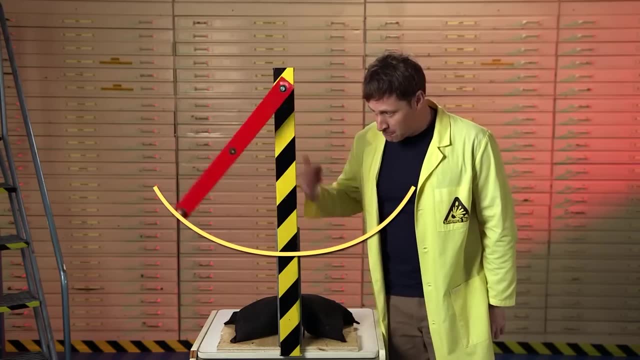 It's a weight that swings. It swings back and forth. Pendulums are pretty simple. It swings back and forth. Predicting the path of a pendulum: Pretty simple. It's gonna swing back and forth. But wait, As I make it so much more complex. 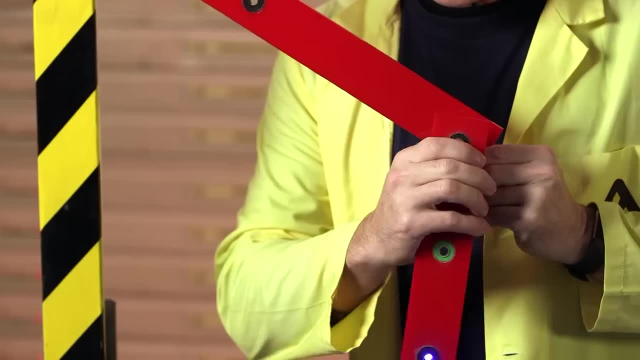 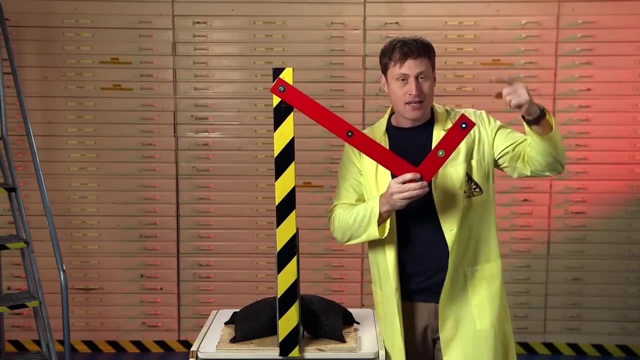 by adding more and more stuff, I end up adding a pendulum. Now I've got a pendulum down here and that one swings back and forth, and I've got a pendulum up here that swings back and forth. What will happen to this part of the pendulum? 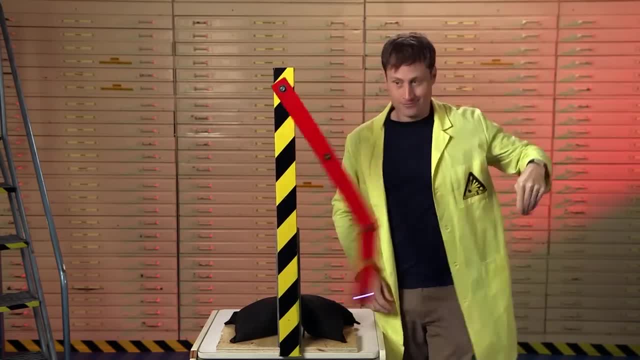 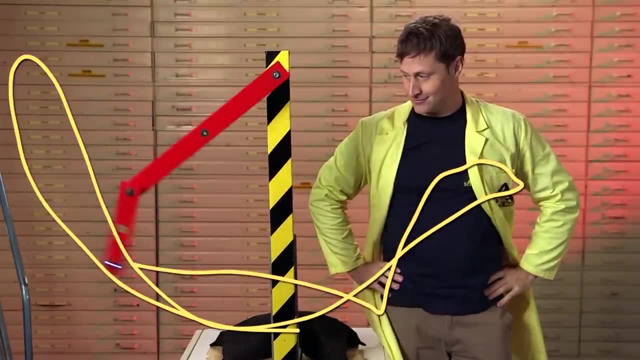 when I let it go. Can you predict? Let's find out. This is a double pendulum, and predicting the path of a double pendulum is really difficult. It's still simple physics, but because there's a moving part attached to a moving part. 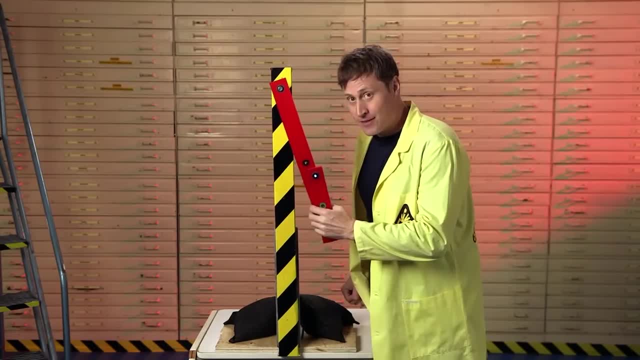 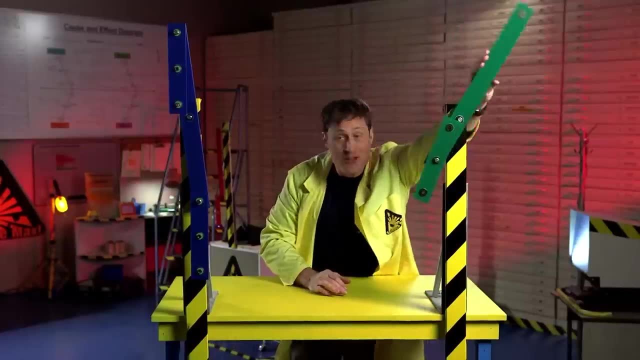 it makes it way more complex. So the question is: can we max it out even more? Of course you can. These are chaos pendulums. This one's a lever and it's got another lever on the end- Whoa. 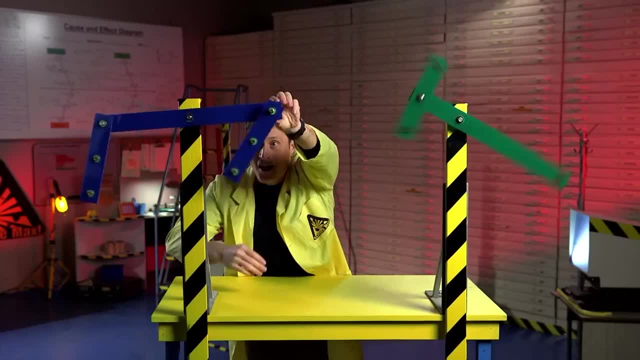 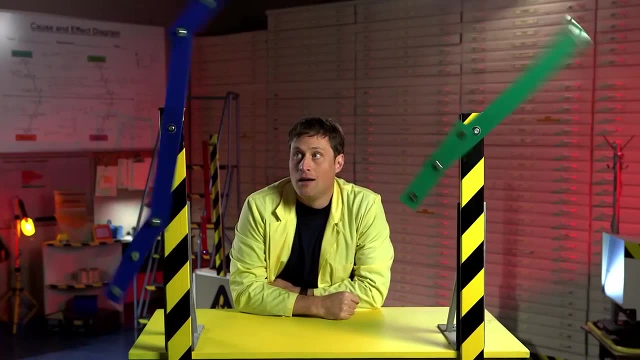 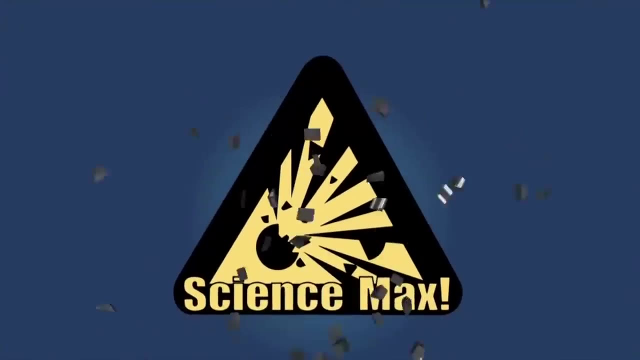 And this one here is a perfectly balanced lever and it's got a pendulum on either side. Whoa, Scientists and engineers have always said that the more moving parts something has, the more complex they are. Science, Sonya and I are taking turns building. 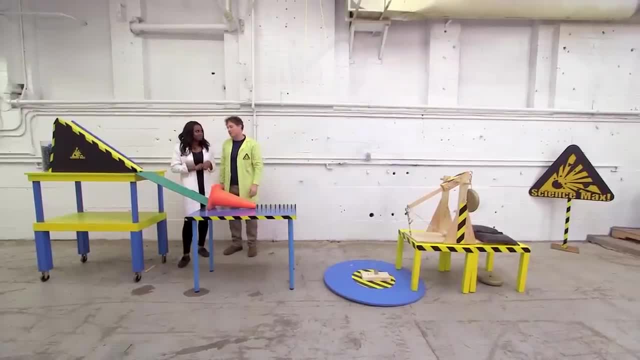 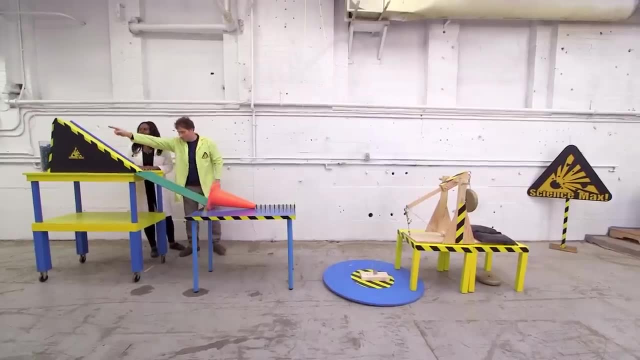 our Rube Goldberg machine. The first section was my turn and I explained it to Sonya Right. here we have what is known as a ramp. Ooh yeah, I know you know that, Nancy Right. So we put a marble on the ramp that rolls along this thing. 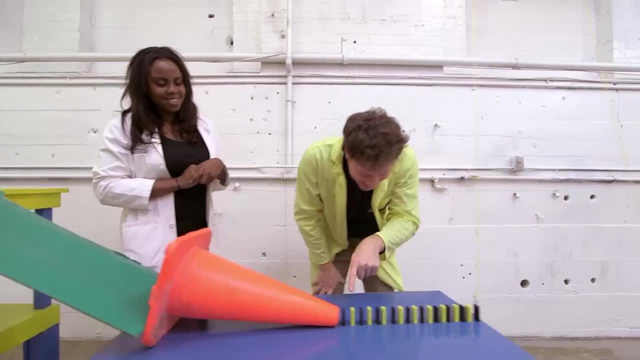 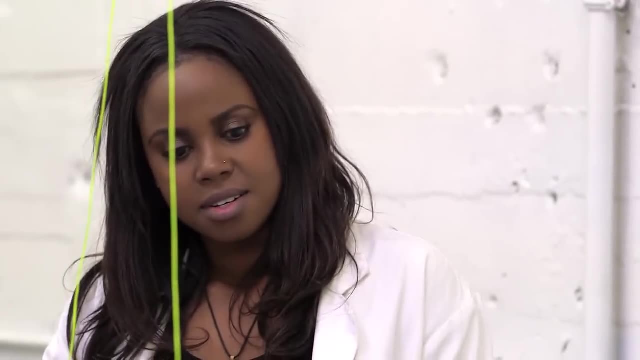 into what is known as a pylon, And then we've got these guys right here which are dominoes, And when that falls off the table, it'll pull on the string and then it's attached to this. Now, this is the release mechanism. 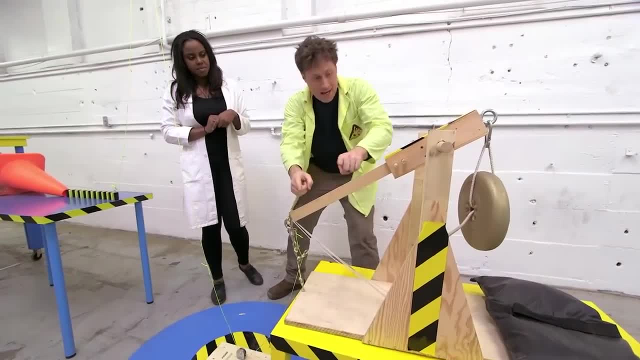 so when that string gets pulled, it's going to pull Mm-hmm, It will let go and it will fire this, which is a trebuchet. All right, should we test it out? Absolutely, Do you want to try it? 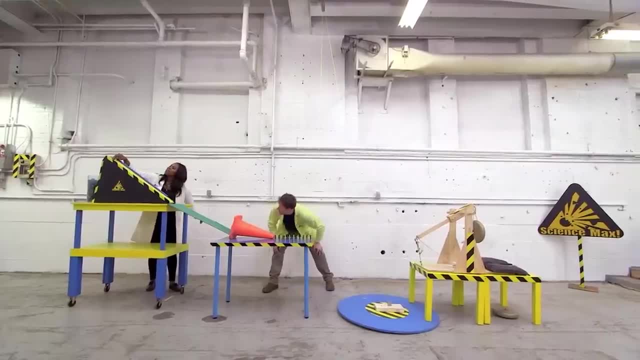 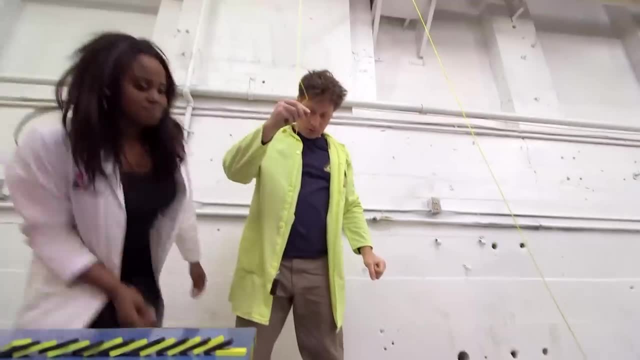 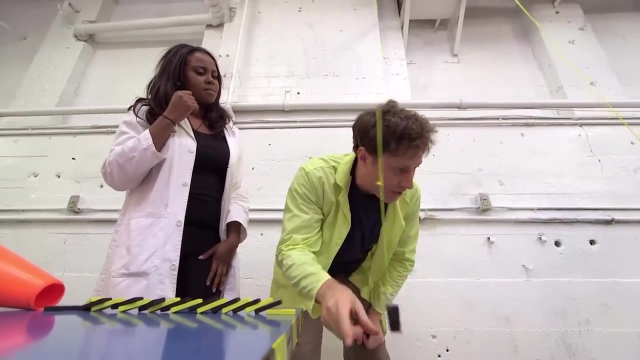 Can I try it? Yeah, Please, OK, OK, Three, two, one, Ah, Ah, Huh, Wait, Hm, Hm Didn't go, Why didn't? Well, the domino doesn't seem to be heavy enough. 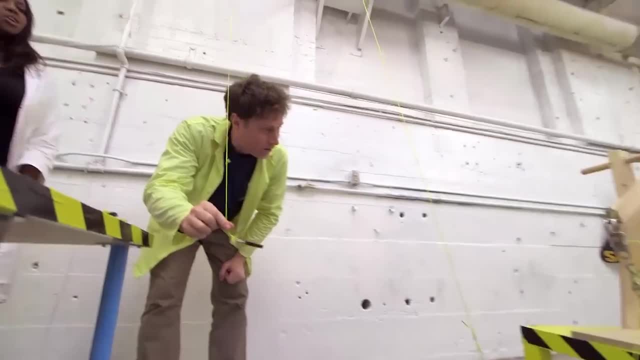 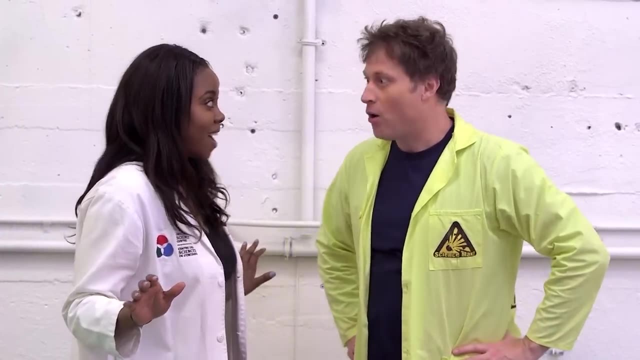 to make this contraption fire. You know what, Phil? What? I have an idea, Oh yeah, Maxed-out dominoes, Maxed-out dominoes. I love that idea. Why are they maxed out? Do they glow in the dark? 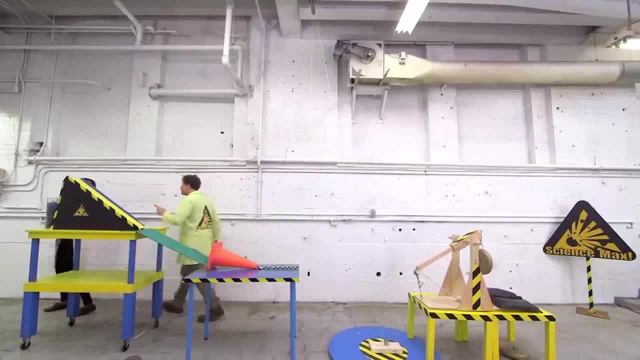 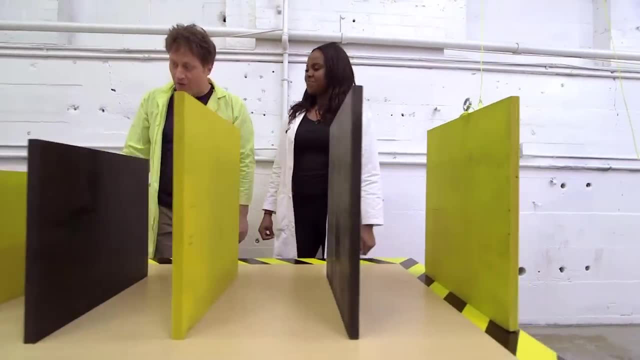 We'll see. Do they produce electricity? We'll see. Do they talk to animals? We will see. Do they dissolve in water? Whoa, maxed-out dominoes. That's what I'm talking about. These are very maxed out. 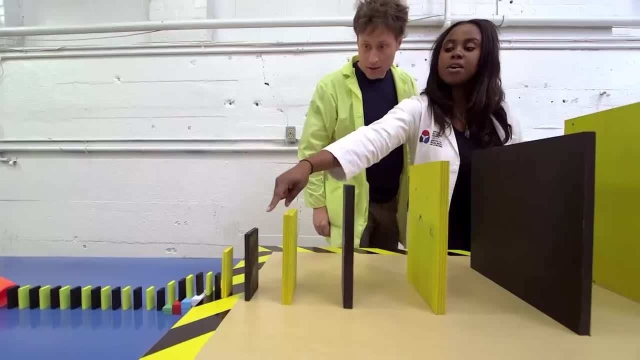 OK, so now, yeah, So we started off with this domino, Uh-huh. Then we went bigger, Yeah, Bigger, bigger, bigger, bigger, bigger, bigger, And we went to the biggest Right, And this is where we're going to get the most weight. which? 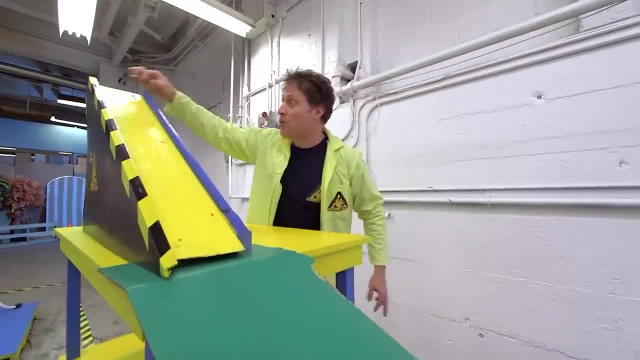 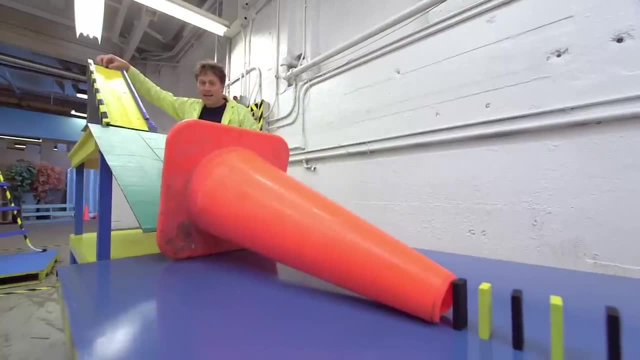 is going to trigger it and release Ha-ha, Here we go. Three, two, one, Here we go. The one thing to remember about Rube Goldberg machines is they never work perfectly. every time. Didn't, didn't, didn't go. 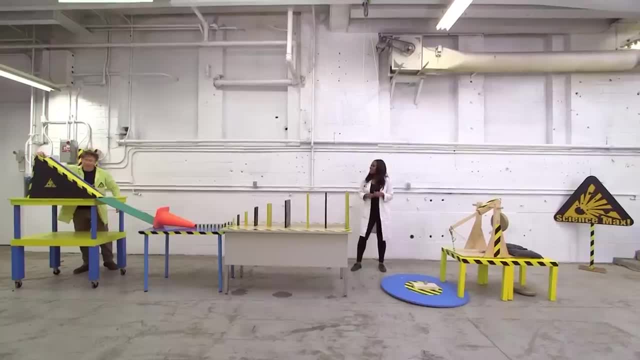 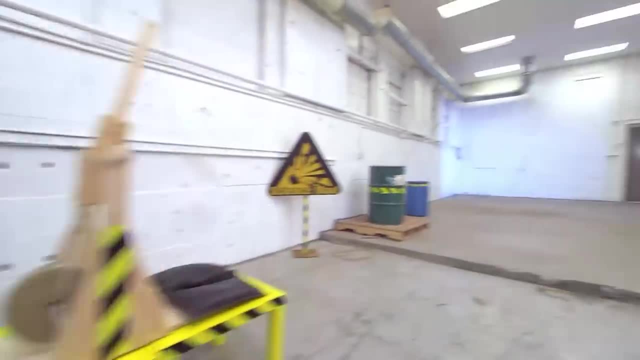 But we tweaked it and adjusted things, And then Here we go: Three, two, one, Whoa Nice, Oh, Oh, Oh Oh, That was pretty far. Yeah, check this out. Whoa, Whoa. 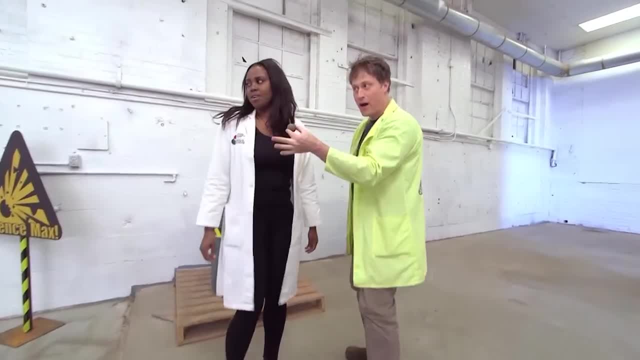 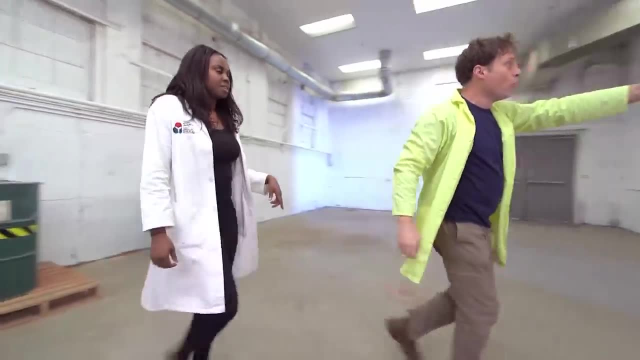 Whoa. OK, So now, Nice, Now that we've got the trebuchet firing, Yep, The ball is going over there. We need to get the ball going over here. Yeah, To the cake button, Cake button. I can't wait for the cake. 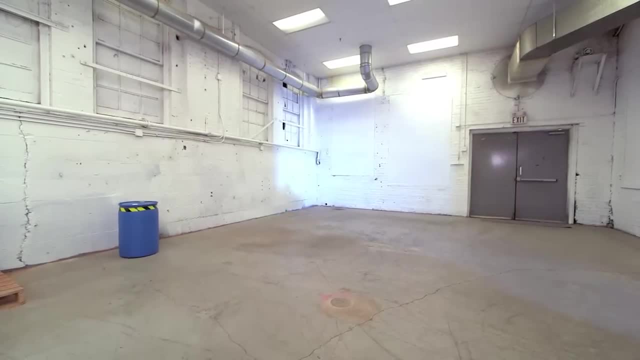 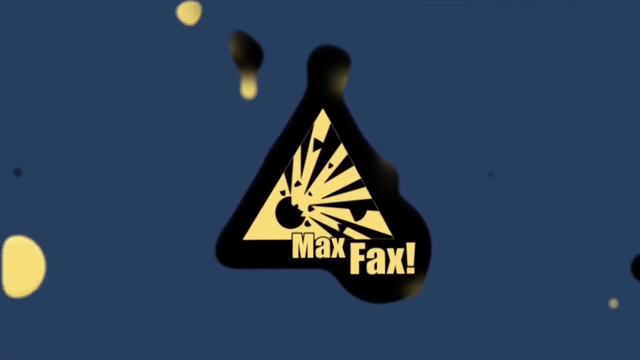 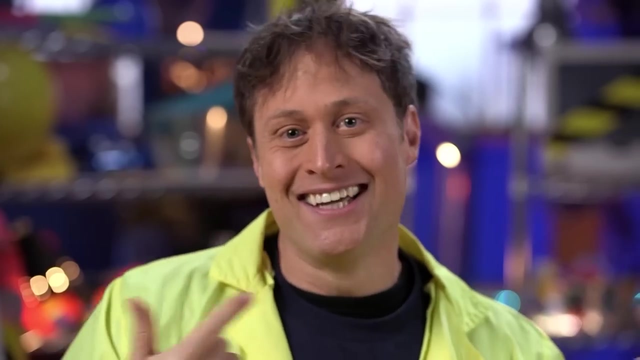 So I have an idea. Come on, OK. No wait, Changing direction, stuff is on the run. OK, Now we're going to talk about tension. What's tension? One more than nine-shin? Get it, Because tension and nine-shin, that's OK. 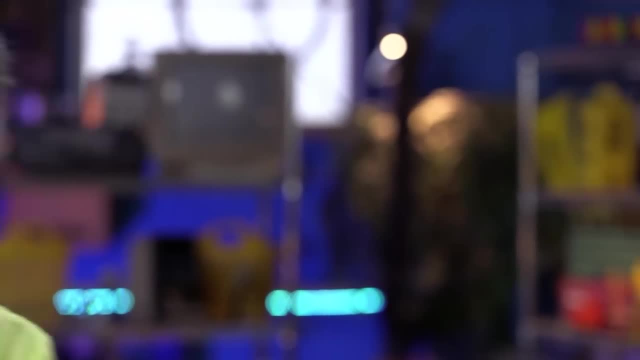 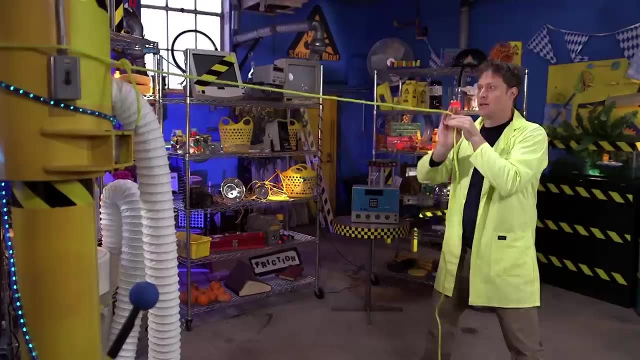 I'll um, because I tension is the force that we usually talk about when we think about pulling a rope or a chain or something like that, Because you know the old expression, you can't push a rope. But today we are going to push a rope. 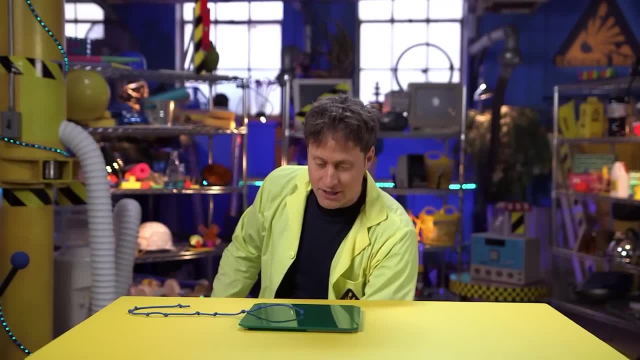 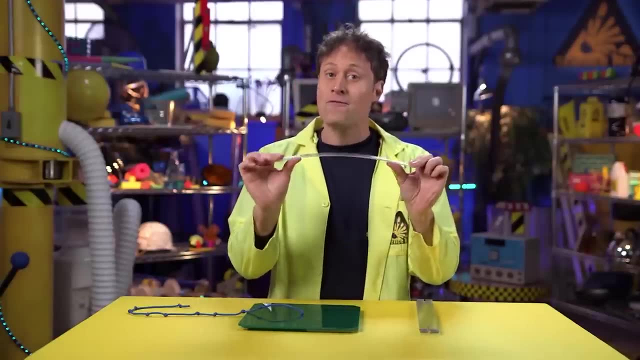 I have a rope right here And I'm going to push it using another force called flexion. I've got some pieces of plastic. I've got some pieces of plastic here And they bend or flex, And when they do, they want to spring back. 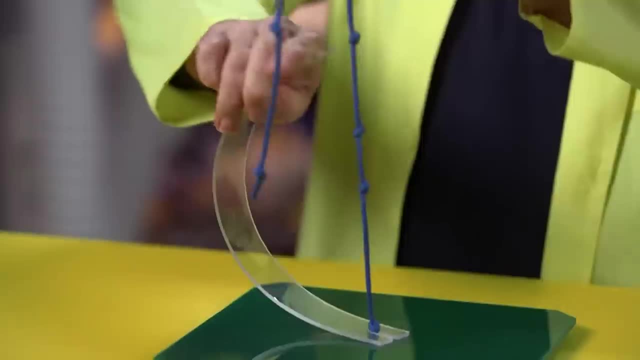 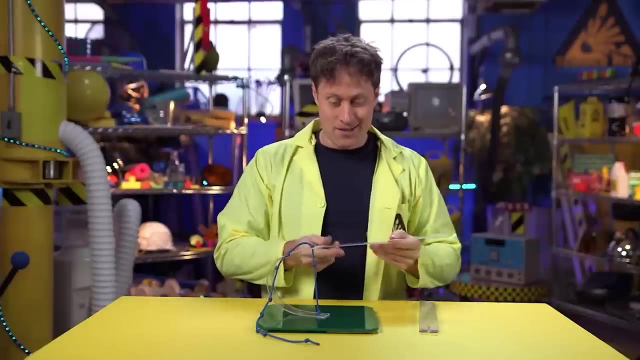 But I'm going to prevent them from springing back by putting them in between these knots. And look, The rope now stays up And I take another piece and I stick it on this knot And then I bend it all the way. This is not terrifying. 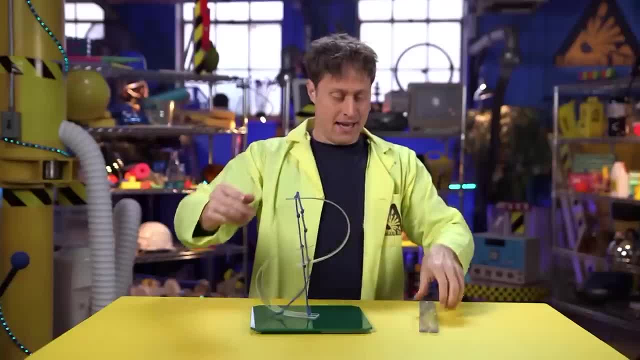 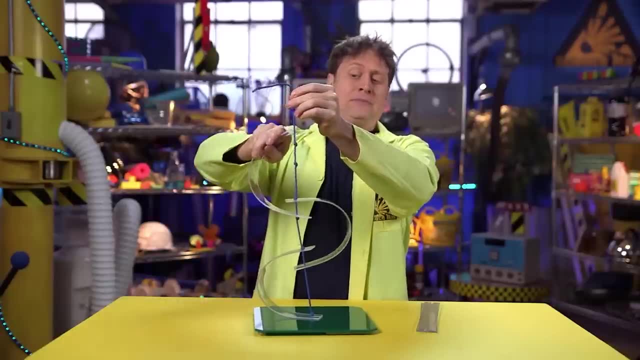 Really it's not terrifying at all. OK, good, And then I take this piece And I put it here And I bend it around, And so now we have a rope that's being pushed And we're defying gravity. 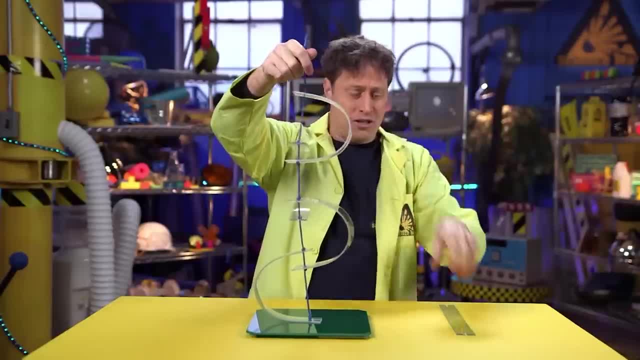 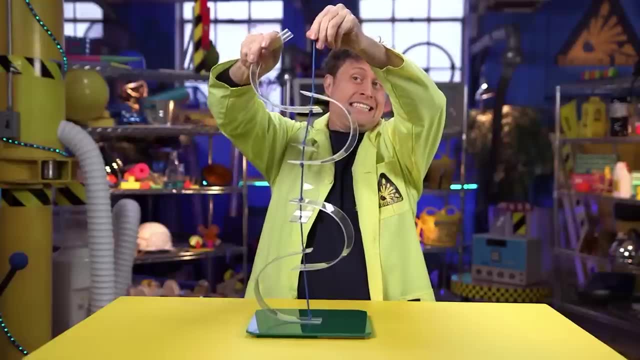 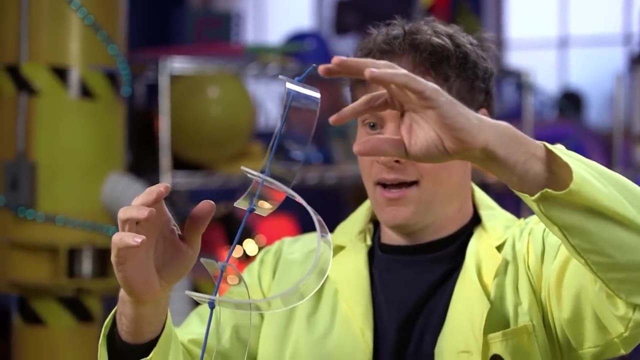 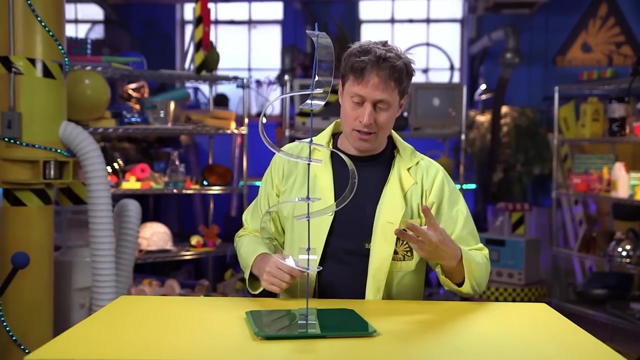 And we're making a cool art sculpture. All right, one more here. OK, here we go And flexing, And whoa Ha-ha, There you go. I've pushed a rope, defied gravity and made a cool art sculpture. 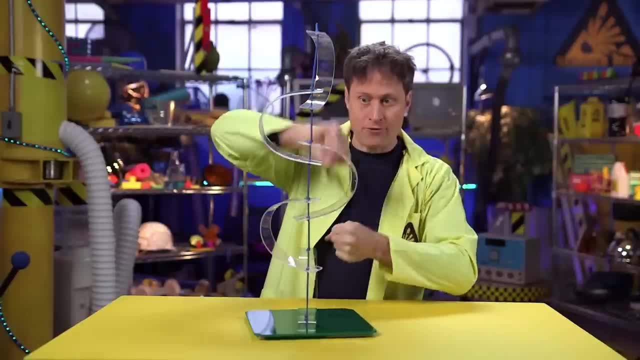 OK. well, I guess technically I haven't really pushed the rope, because we're still pulling from each knot, And I guess I haven't really defied gravity, because that one's sitting on the table and all the others are sitting on top of that. 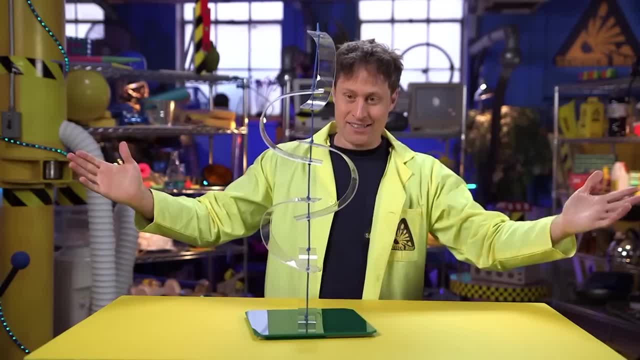 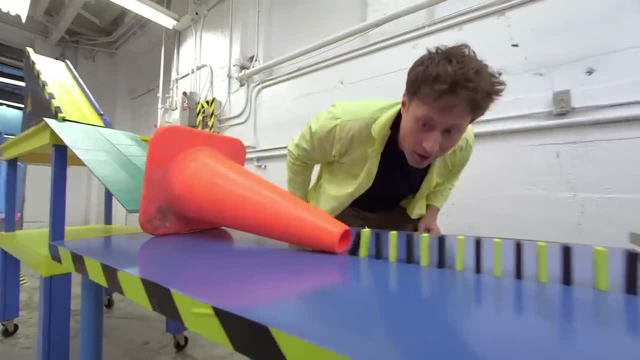 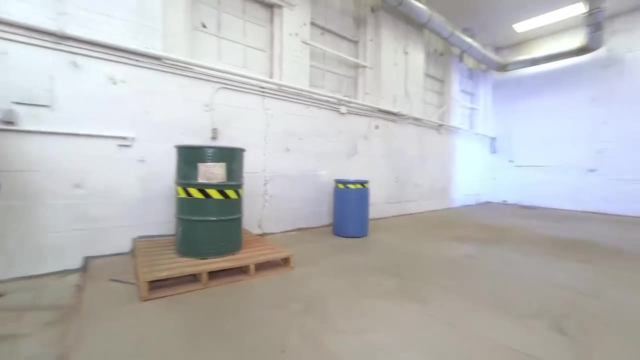 But you can't argue that I made a cool art sculpture. Ha-ha Art, I mean science. Sonia and I are maxing out a Rube Goldberg machine. Whoa. The first part worked pretty well And now we need to change the ball's direction. 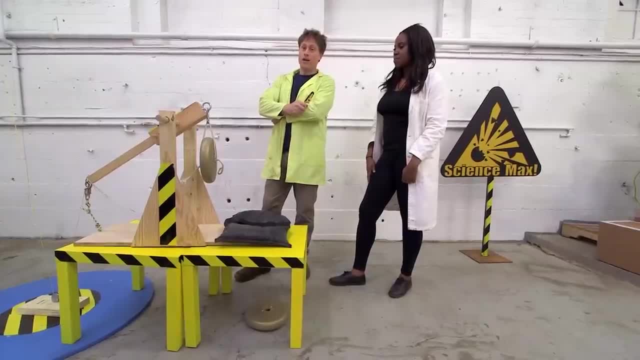 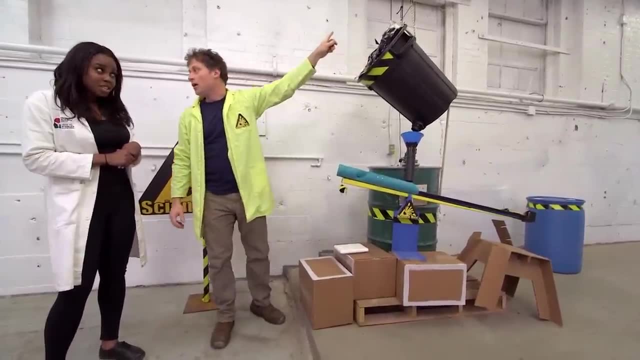 So this is trebuchet. Trebuchet fires the ball, right, Yeah, Right. now I want to tell you the story of the ball. First it goes through this fancy film of tin foil: Uh, aluminum foil, Right, aluminum foil. 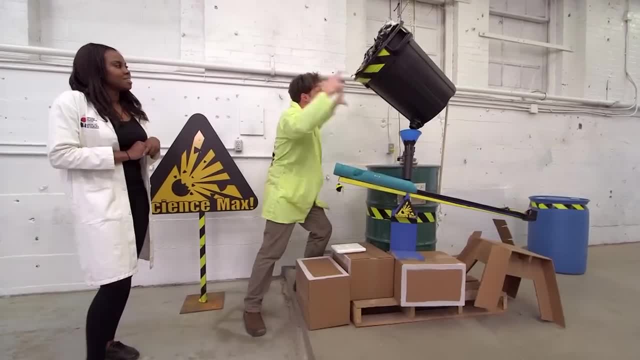 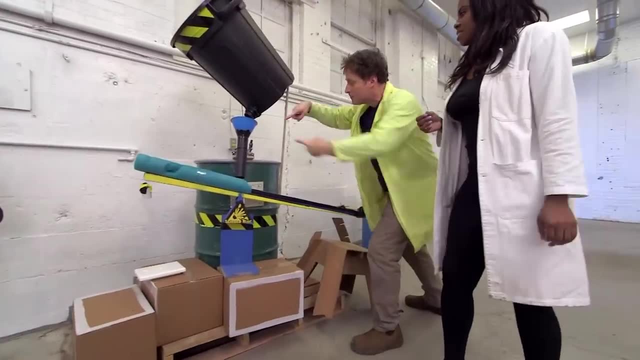 Because it's- yeah, you're right, it's made of aluminum. It enters this large receptacle- Uh, a garbage can You also could be called a garbage can It falls into this conular, conular um device. 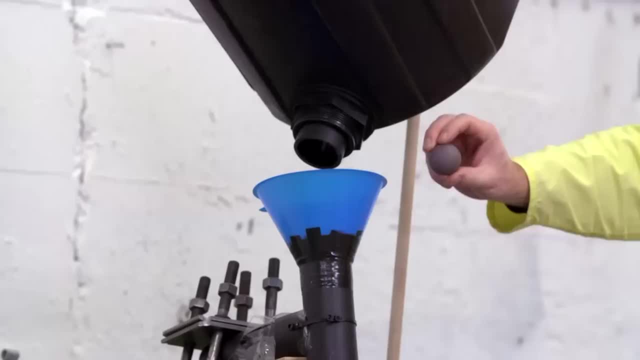 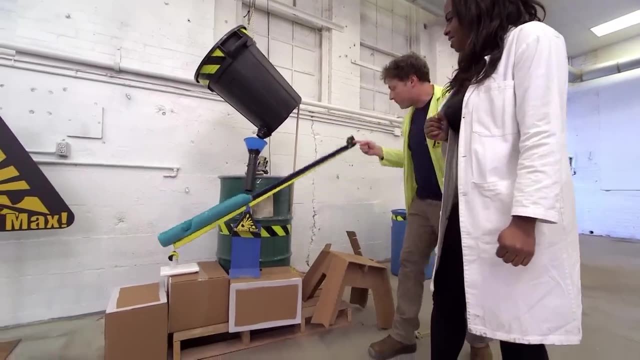 A funnel. A funnel- yes, You could call it a funnel- And then it enters the change-o-direction-o-matic. All right, Which is a lever. There's a weight on that end, Then it falls off. Then the ball goes this way: 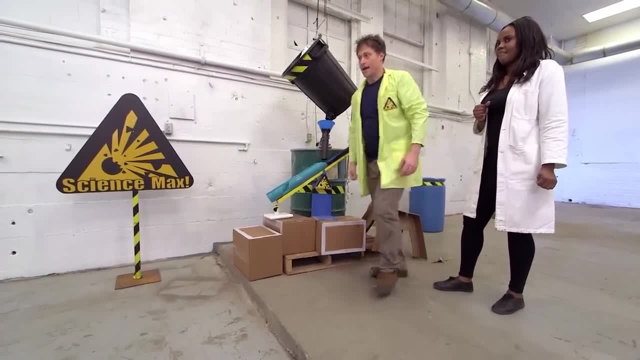 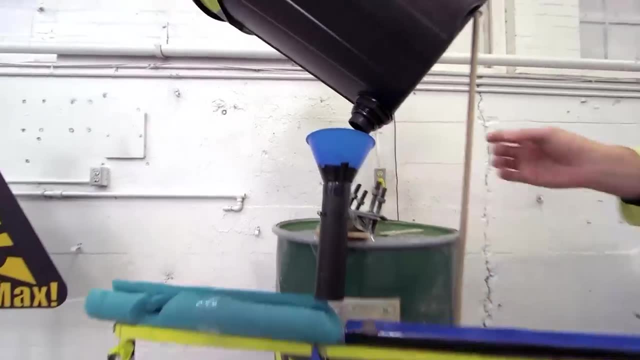 Uh, nope, Or that way. The one thing you need most of all when making a Rube Goldberg machine is patience. Ball goes in the funnel, Knocks that off, Changes direction, And then it goes this way. Okay, And that's all I got so far. 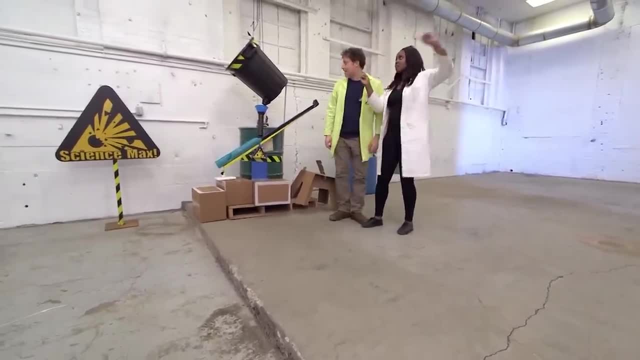 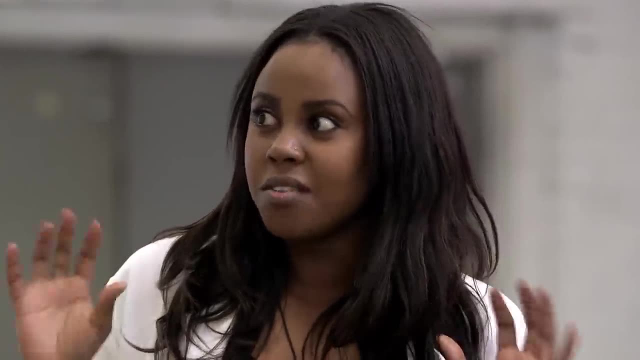 So not bad, Yeah, But we really want to get closer to that way, Right, because that's the button that gives us cake. How about we use some chemical energy for this? Ooh, chemical energy. I have an idea for this one. 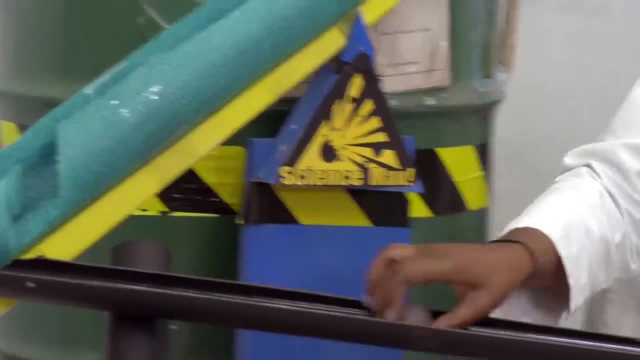 Let me go get it. Go for it. This is my idea. Okay, Ball's actually gonna roll down the tube. Oh yeah, because this is a rat trap, right Yeah, Which is like bigger than a mouse trap. 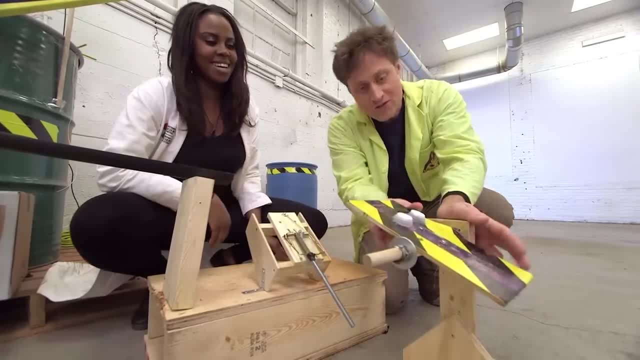 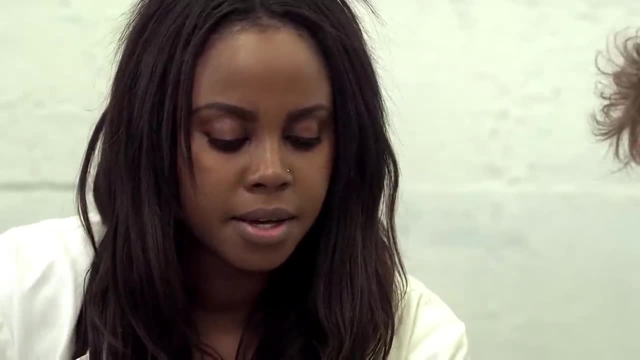 And then it's gonna hit it. Yes, Nice, Ooh. so this flips around. Exactly. And what's this? That is something called an antacid tablet, Some water, Exactly, And the antacid and the water react. Oh, 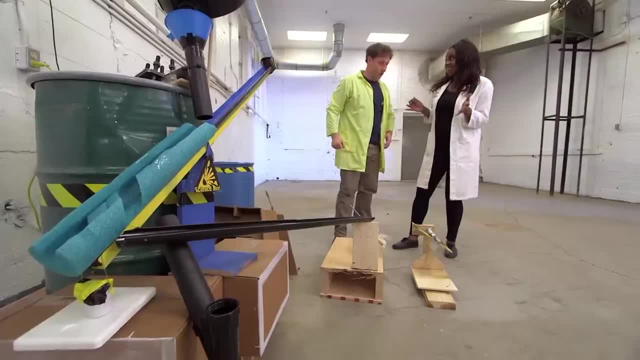 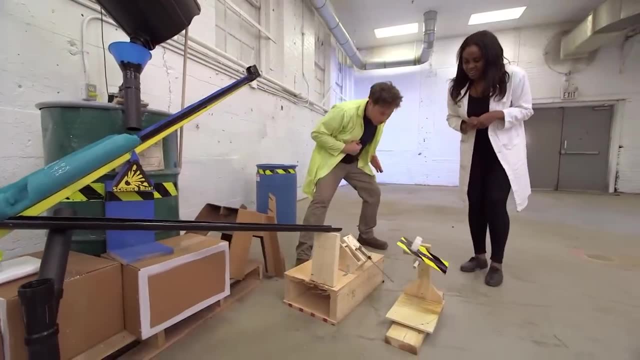 It blew. Do you want to test it out? Sure Can I. Okay, Okay, Ball comes through, this Goes down, there Comes out of this And on the ramp Onto the trap, Ooh And Ah. 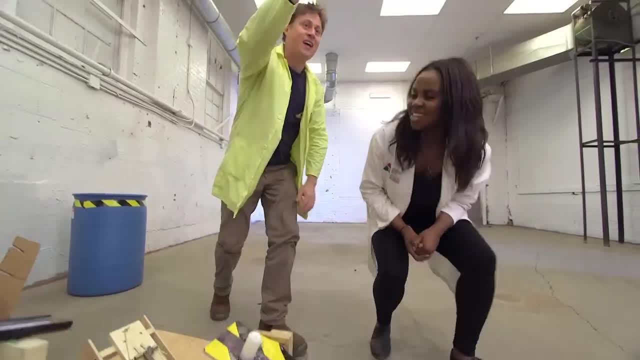 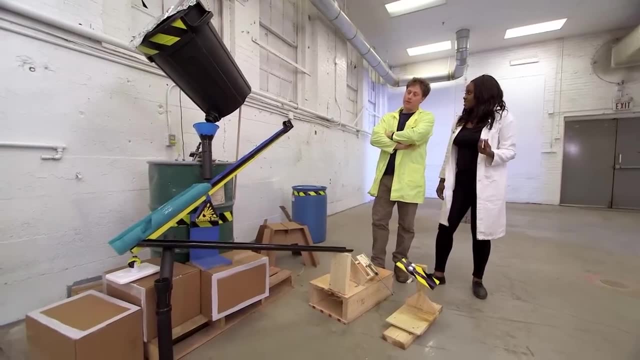 So then it Nice, Fires up, Yep, And hits something else, Yeah, And something, something, something, button cake, Hmm. So we got a lot of different energies, But you know what? What's missing? What Is electrical energy. 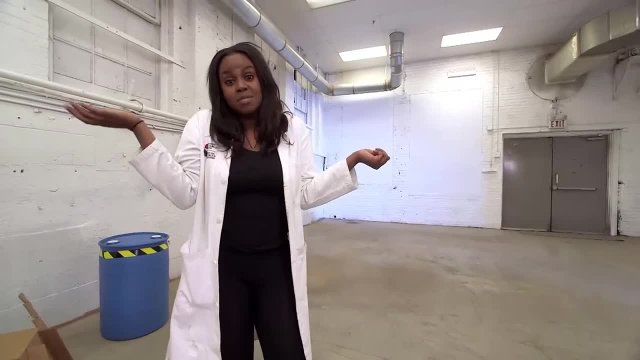 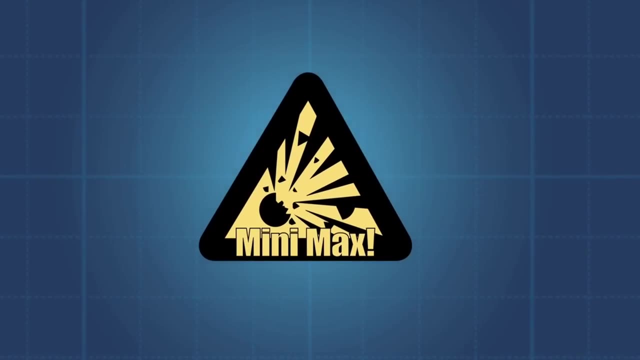 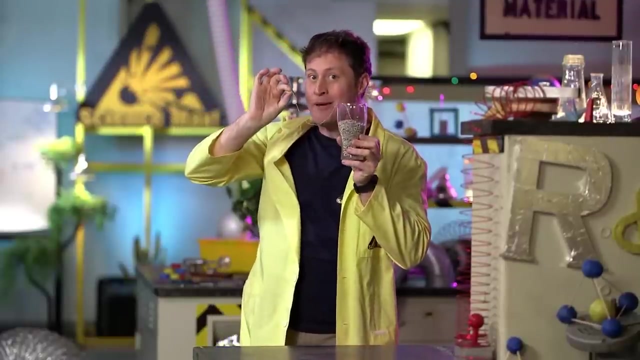 Yeah, You're actually right. I've got a great idea. Hold on, Hold on. All right, Let's see what he comes up with. This is a chain of beads And this is a glass. Now, if I was to drop the chain of beads, what'll happen? 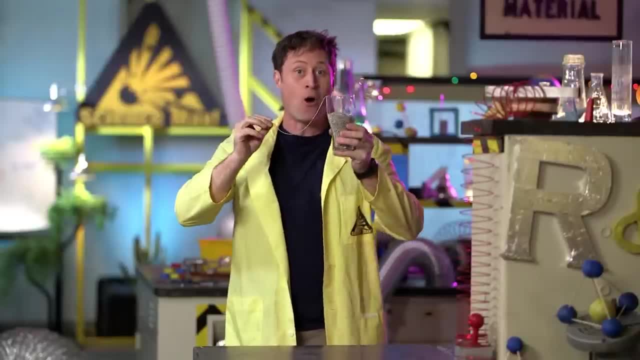 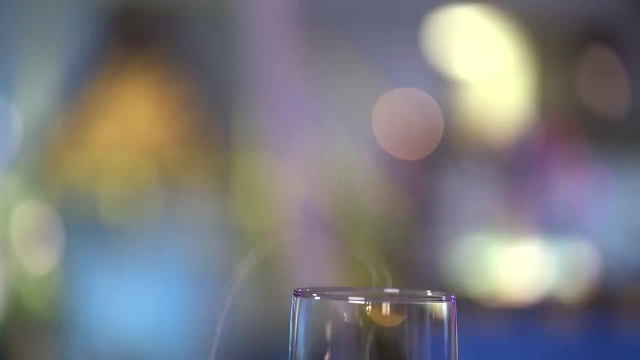 It will fall. Yes, That's right, It'll fall because of gravity. But watch this: This side goes up. Why? Because of gravity. Wait a minute. Wait a minute. Why does one side go up because of gravity? Well, it gets a little complicated, but I can explain. 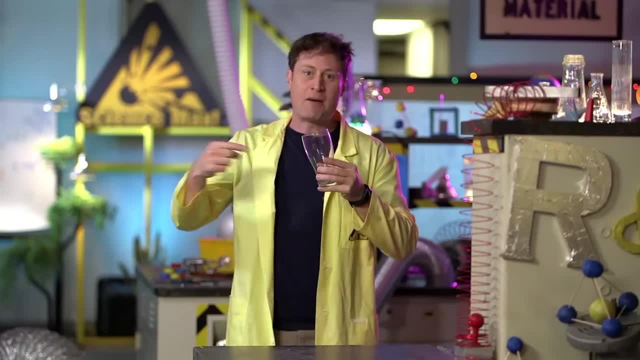 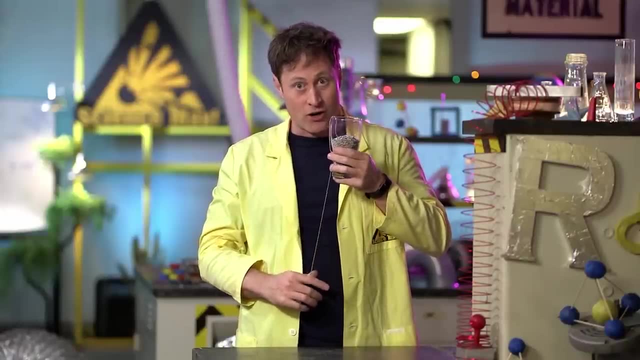 Um, but I think I should. I have to put the beads back in the glass, Okay, So what's going on? Well, when this part of the chain starts falling out, it gets longer and longer and it has more mass than this side of the chain. 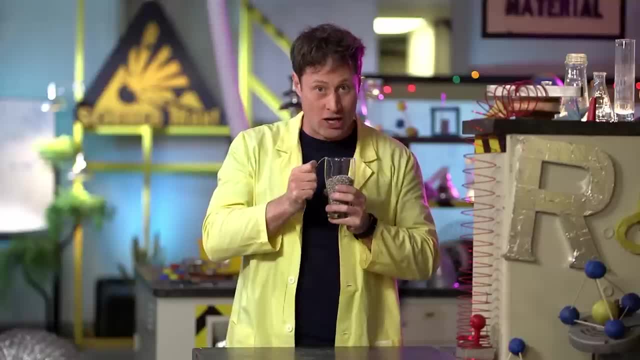 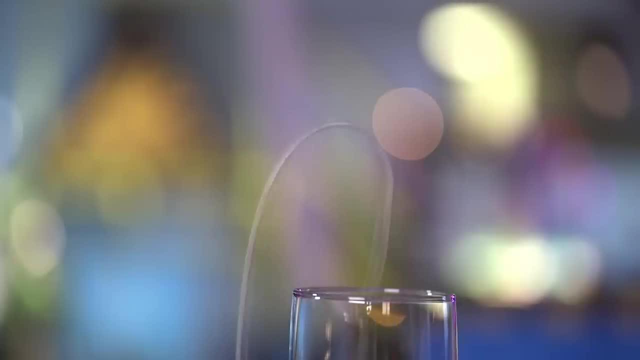 And if it has more mass then it has more inertia. And when it starts yanking out very hard, this side of the chain gets yanked up Out of the glass very quickly. When it gets yanked up hard, it flies into the air. 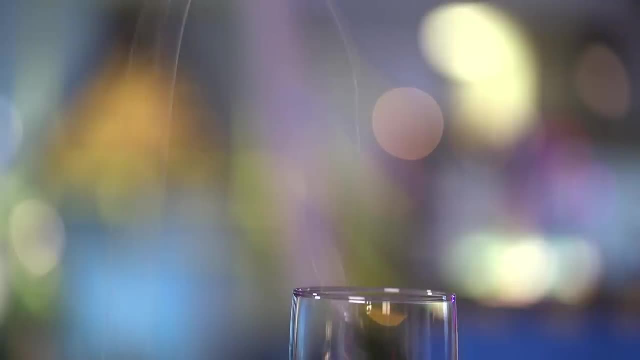 But then of course, the direction has to change. so it goes around a curve and then goes back down. Because of the speed that it's going, that curve starts lifting up over the top of the glass, And that's how it works. 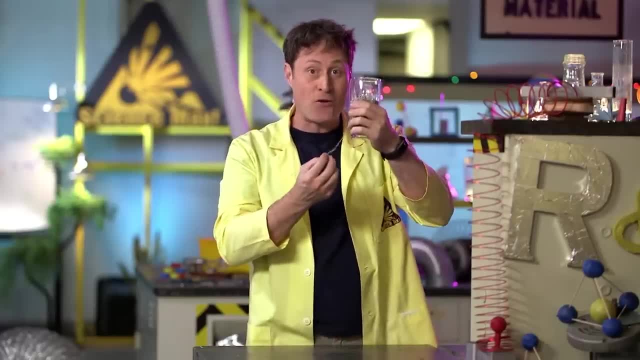 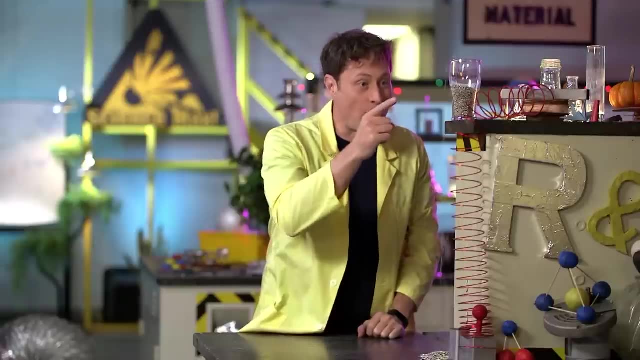 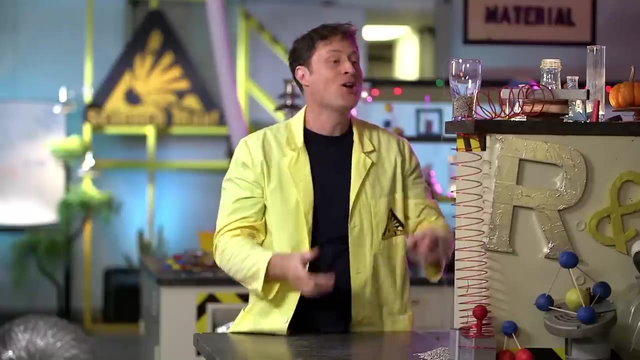 There's a big difference in energy because this chain falls far. I try it from here and it doesn't work as well. Why? Because the drop from here to here isn't as big. You want lots of force acting on the falling chain, which means the higher you do it from. 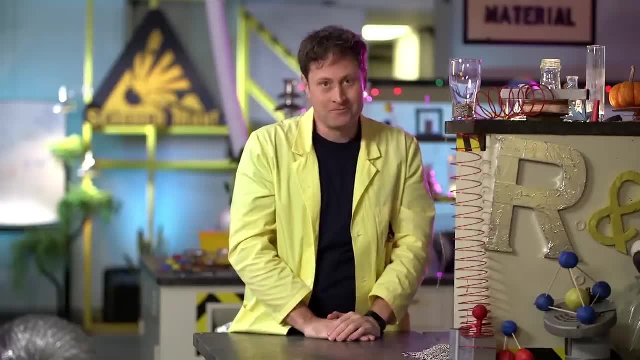 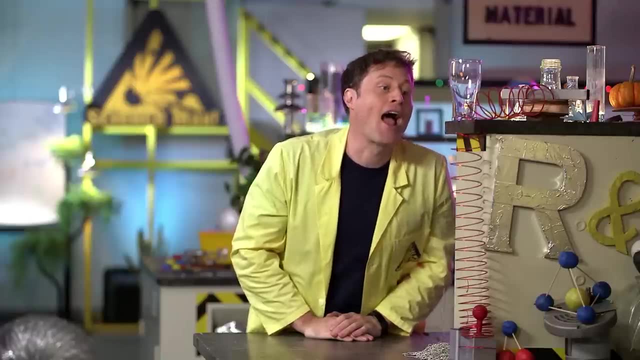 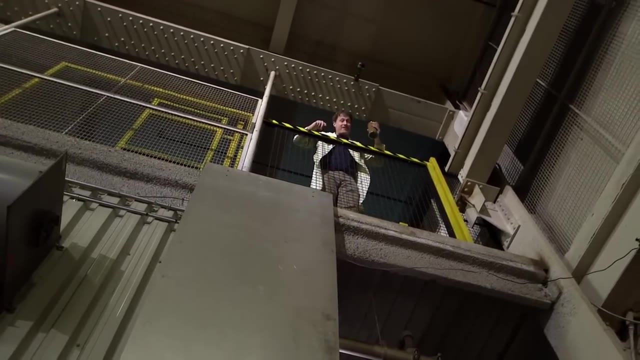 the better it works. So maybe we should max it out. Yeah, We should wait for it to stop, And now let's max it out. This is a really long chain and this is a really long drop. Let's see what happens. 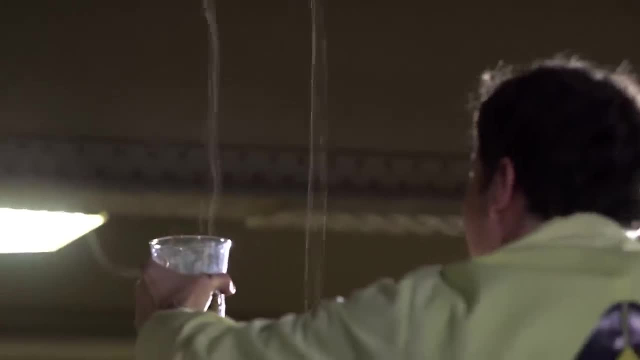 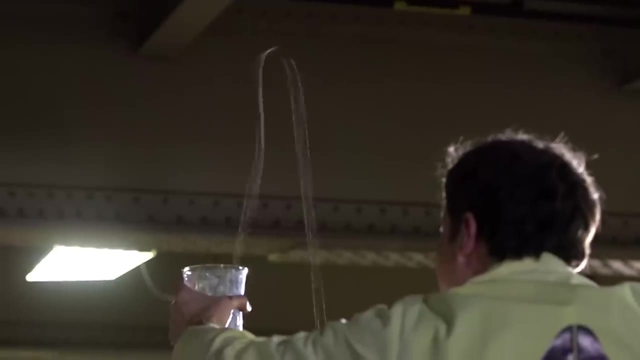 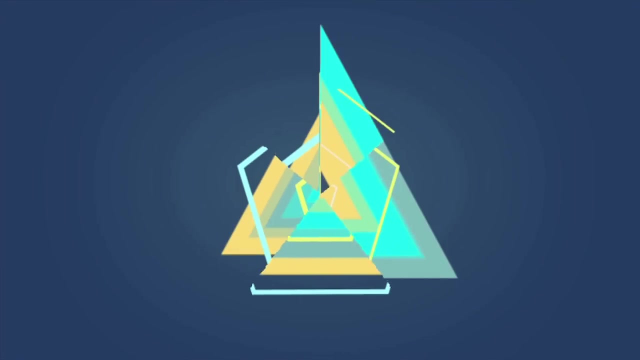 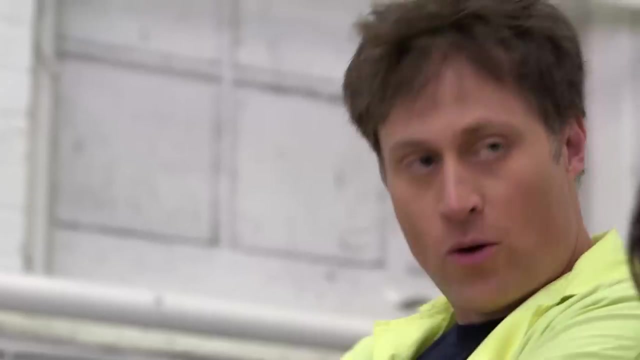 Whoa, Look at that. Whoa Super maxed out Science. Sconee and I have used potential energy, the lever and chemical energy, But you know what one we're missing? What Is electrical energy? Electromagnetism. 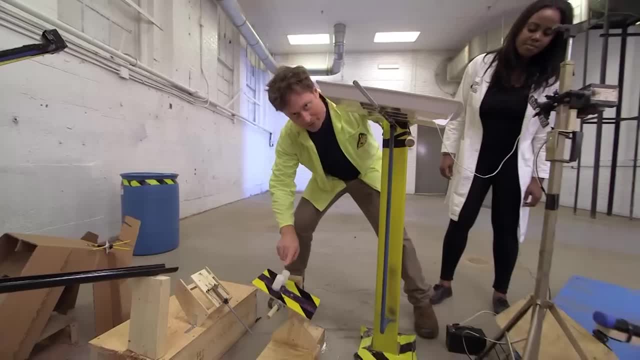 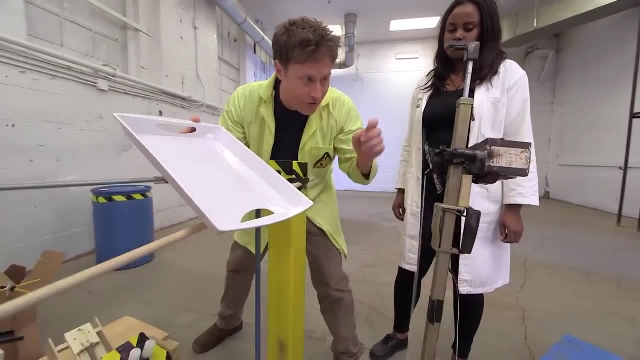 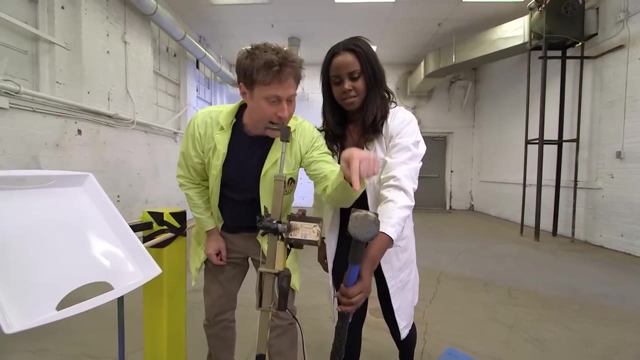 So watch, So watch the chemical rockets which we've had from before. they'll fire up, they'll hit the underside of this tray. The marbles will fall and flick this switch. See that sledgehammer. This is an electromagnet and it will attract. 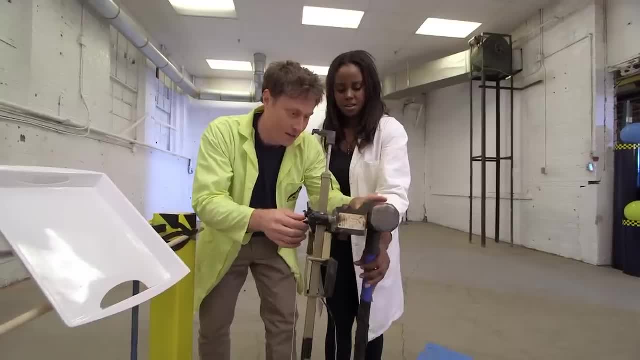 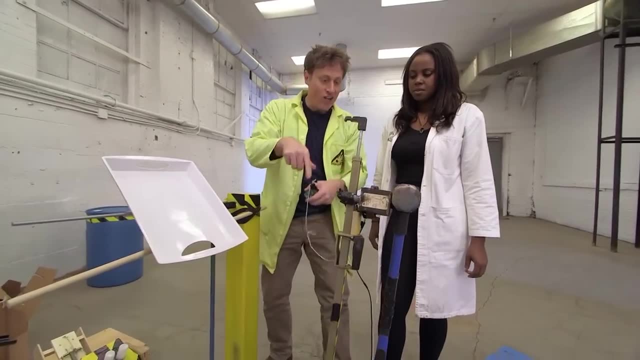 the metal in the sledgehammer. Watch this ready There: magnetized electromagnetism. Now, when the marbles fall, it'll turn the electromagnet off and the hammer will fall. Oh, that's pretty cool actually. 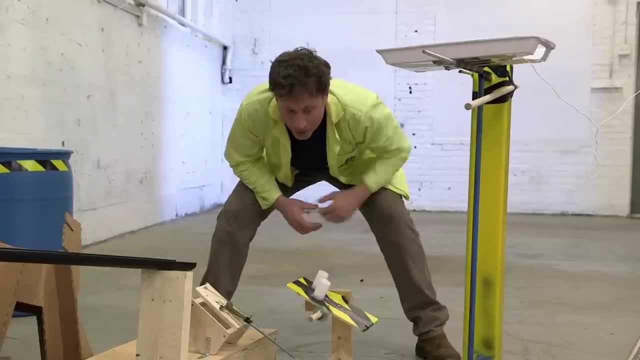 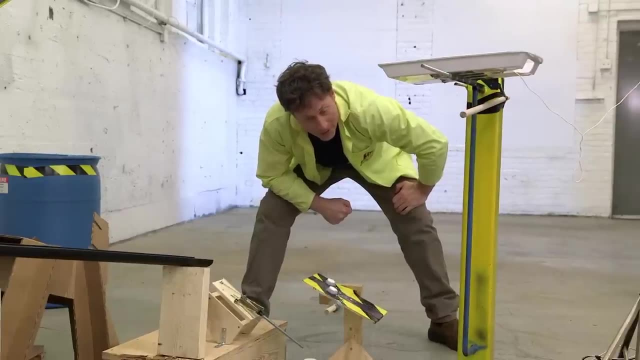 Right, Can we try this? So let's try it. Here's something we didn't know: Predicting the flight path of an antacid rocket canister is almost impossible. We had them aim the same way every time, But we stuck with it, and being patient is key. 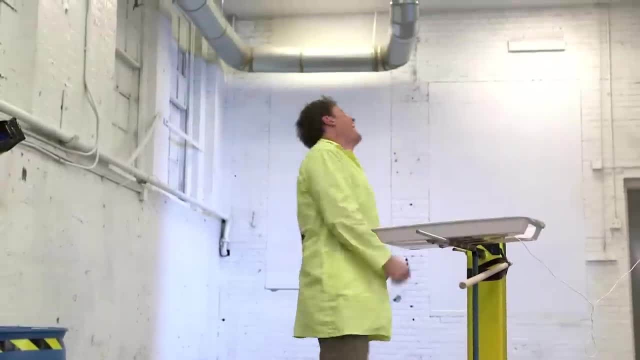 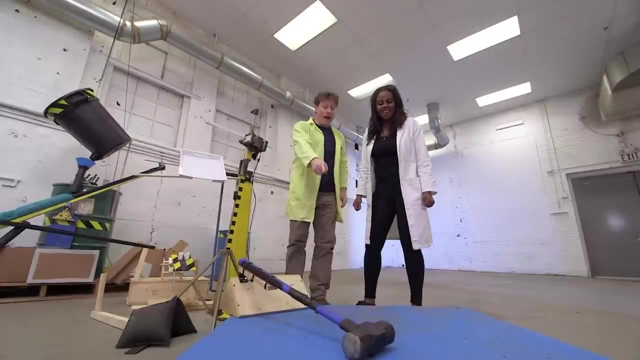 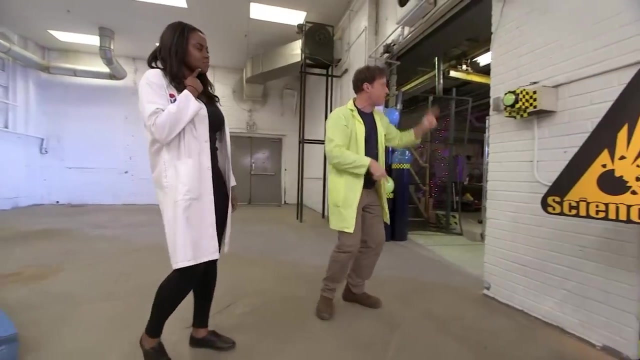 and eventually, eventually it worked. The chemical rockets fire and they hit the trays. All right, That's pretty cool, Yeah, so now we just need hammer hit something and then something, something, something, button cake. I have an idea. 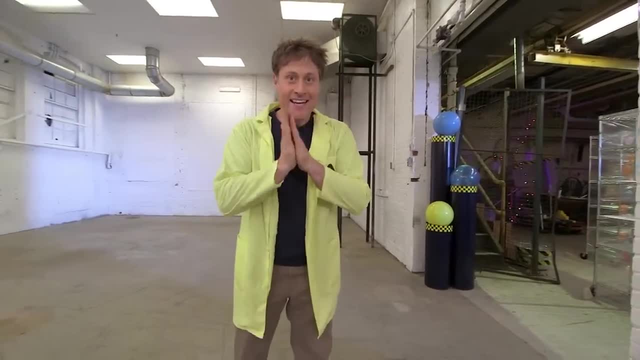 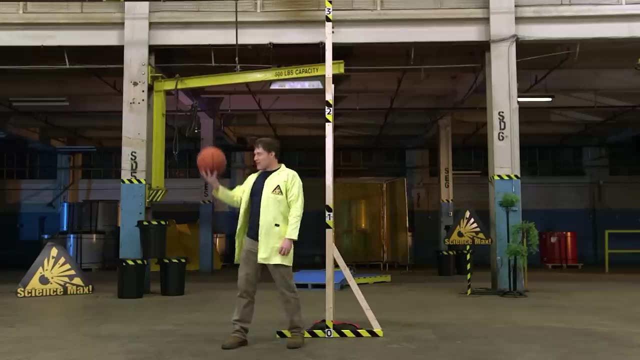 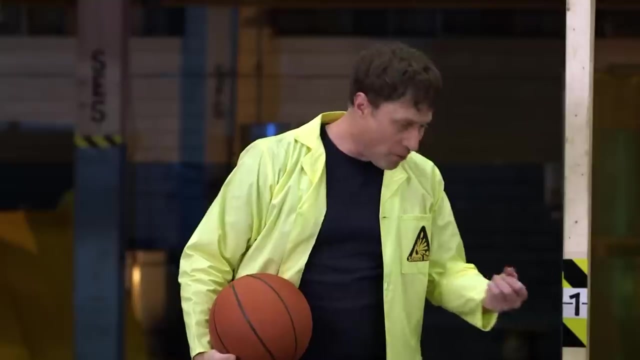 All right, Cake any minute now. This is a basketball- It bounces. This is a golf ball: It bounces, But it bounces. It never bounces as high as where I dropped it from. But watch as I put the golf ball on top of the basketball. 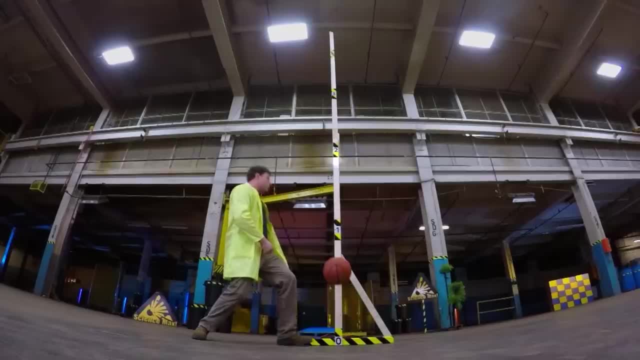 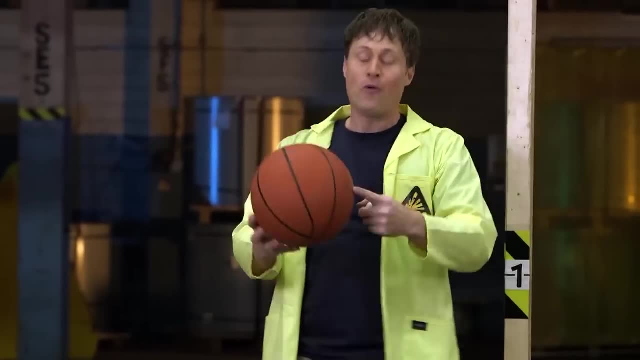 Whoa. Why does the golf ball bounce higher than where I dropped it from? How is this possible? I only bounced the golf ball from one meter high. So what's going on? Well, as the basketball hits the ground, it compresses, storing the potential energy of its bounce. 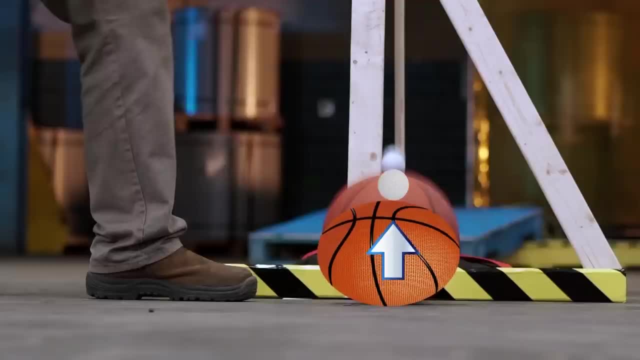 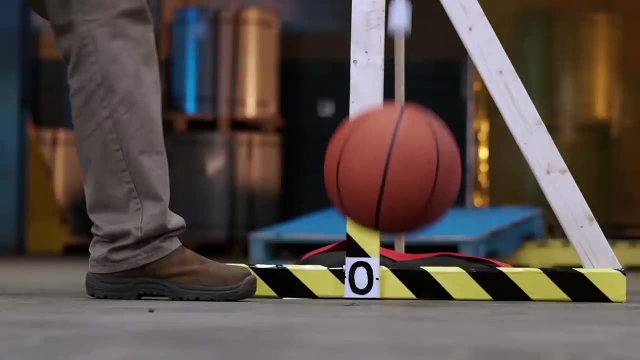 about to give that energy back as it bounces up again. But this energy works as a springboard for the golf ball And since the golf ball has a lot less mass than the basketball, the upwards kinetic energy of the basketball is given to the golf ball. 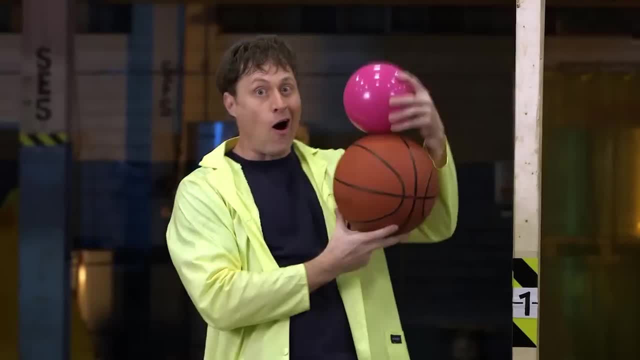 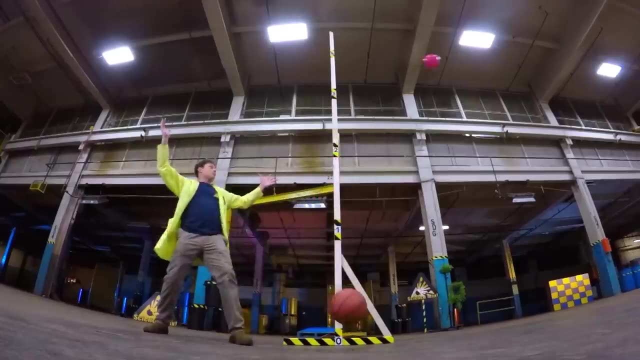 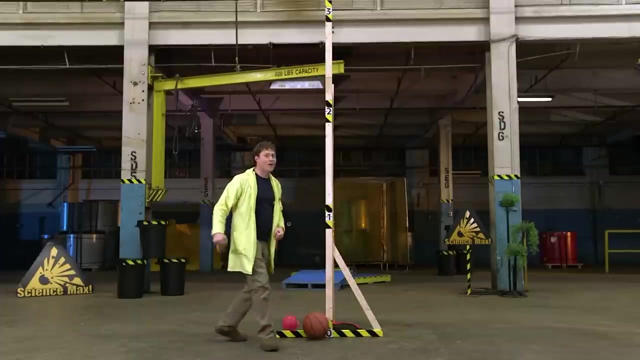 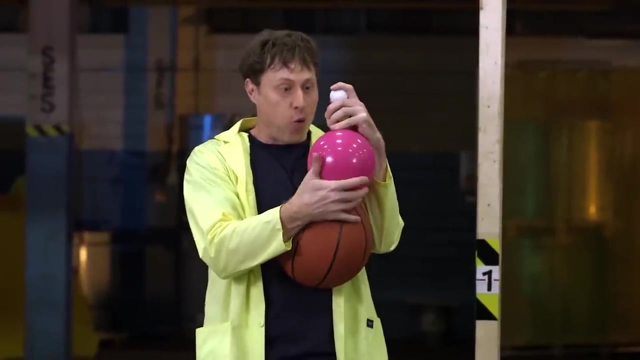 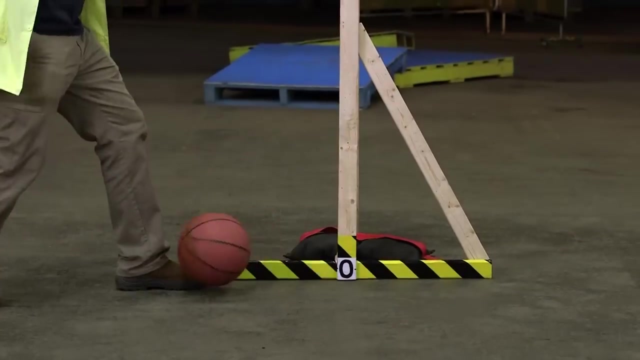 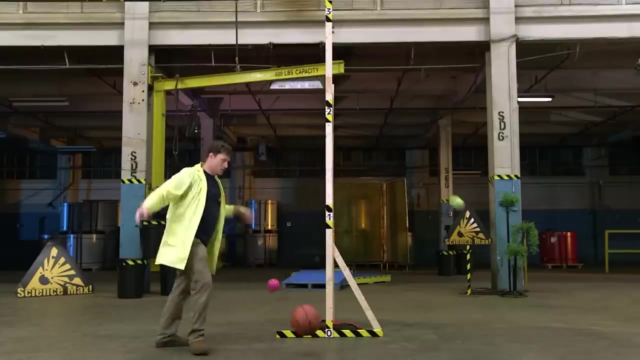 So let's max it out. Ball on a ball on a ball- Three ball bounce. Did you see that? Ball On a ball on a ball on a ball- Quadruple ball bounce? No, wait, Turns out getting four balls to drop straight down. 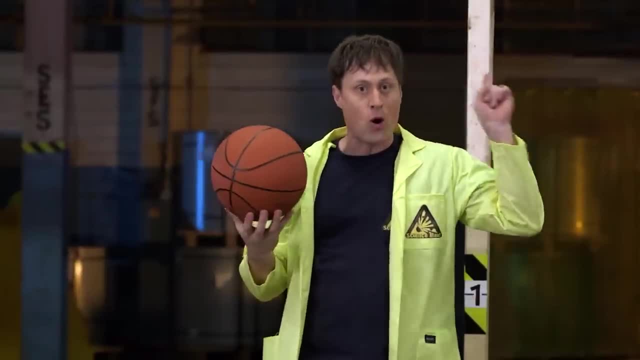 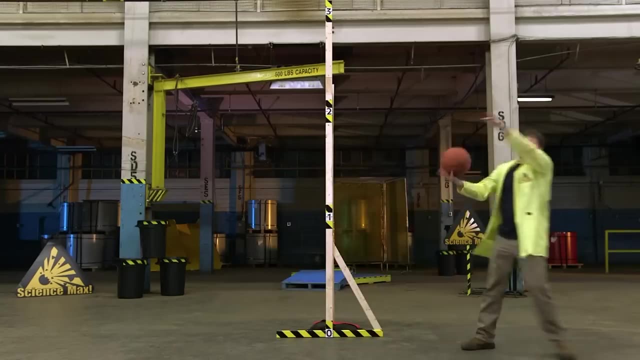 on top of each other is pretty difficult. So we know the mass of the ball is important. Why don't we max it out in a different way? This is a Swiss ball for exercising. It has a lot more mass than a golf ball. 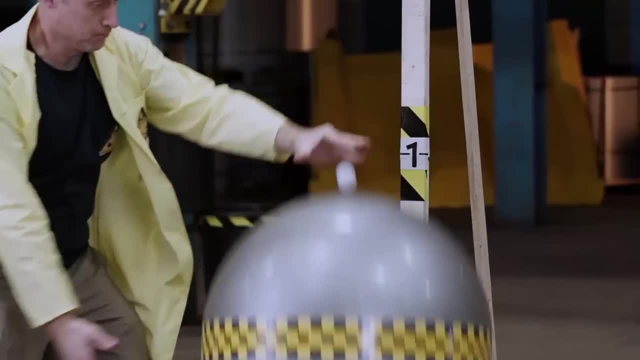 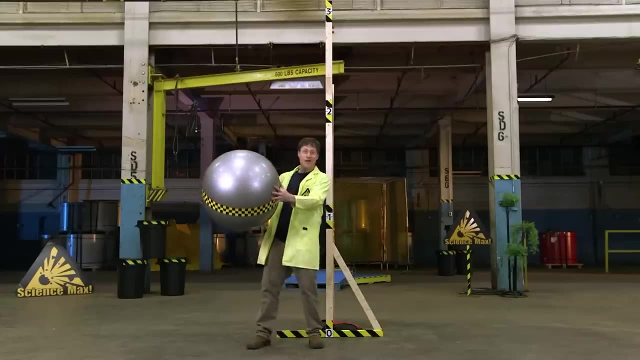 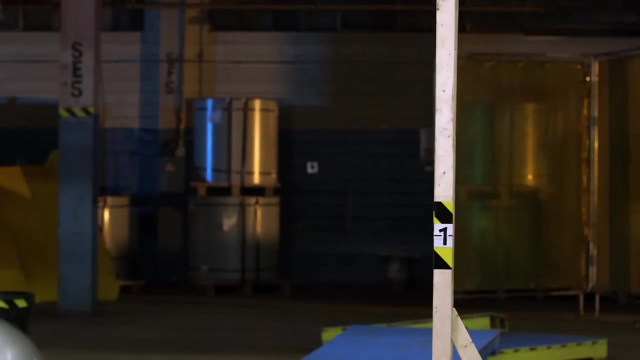 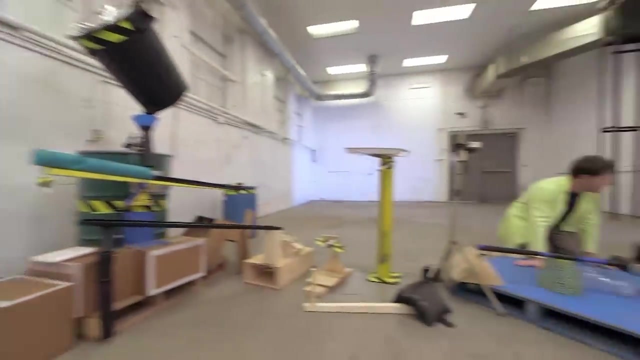 So let's try it out. There you go: The transfer of energy between balls- A great way to lose golf balls. Sonia has added one more step to our Rube Goldberg machine: a stomp rocket. It's a hammer rocket, Exactly. 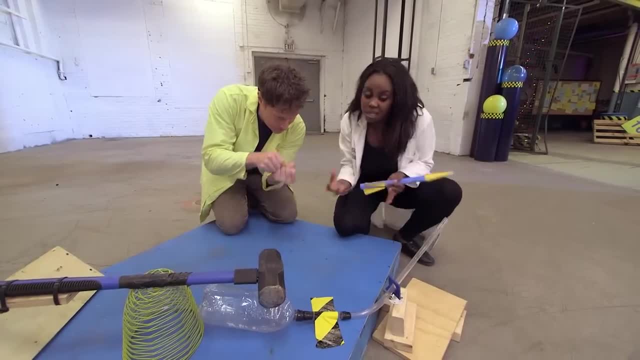 I like that. So what's going to happen is the hammer is going to hit our bottle Right, Which is going to release all that air that's built up inside of it. It's going to hit that button. Wait, wait, wait, wait. 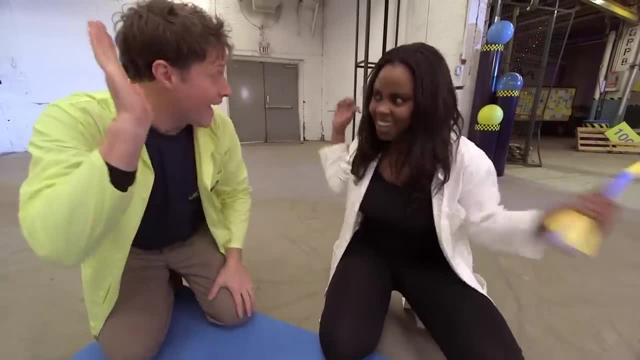 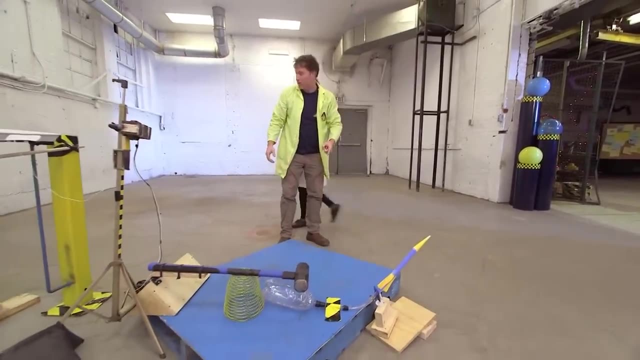 The rocket hits the button And then we get some Cake, Cake, Cake, Cake. So this is it. So we're done, the Rube Goldberg machine with this last step. Okay, Do you want to do it? I think we should do it. 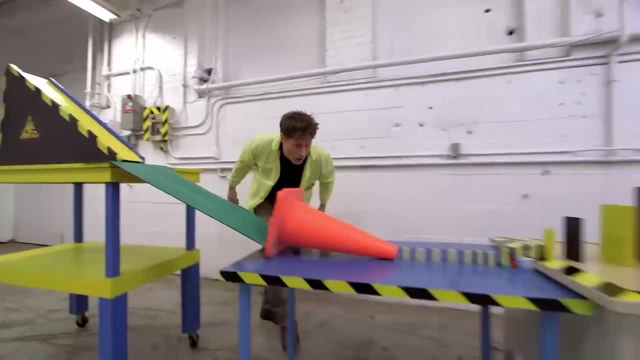 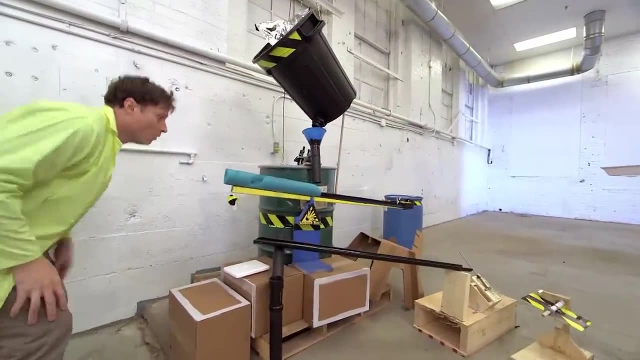 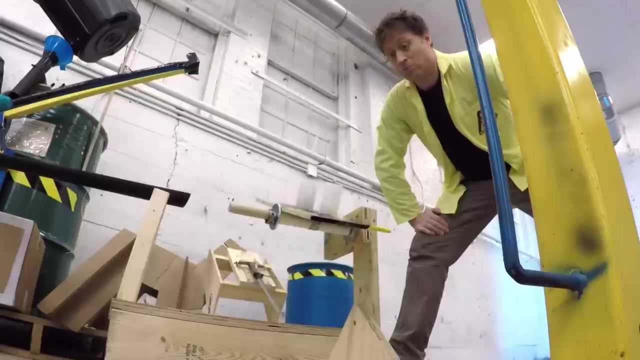 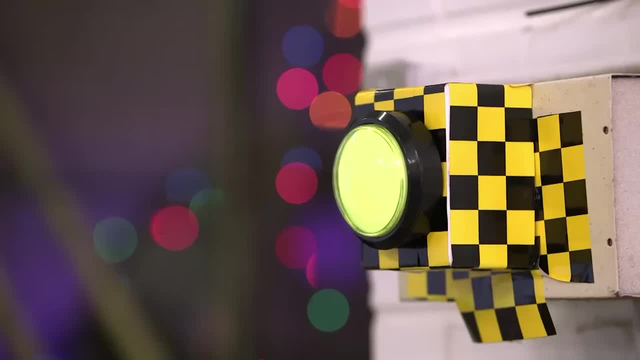 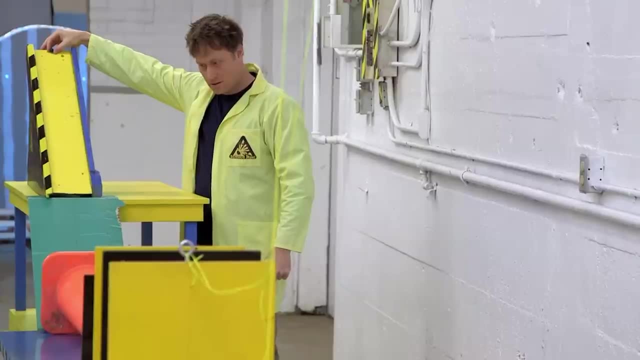 Oh, Oh, Oh, Oh, Yes, Yes, Yes. Let's pause here just before the Cake Portal's in and recap the science. A marble on top of this ramp has potential energy. As it rolls down, that changes to kinetic energy. 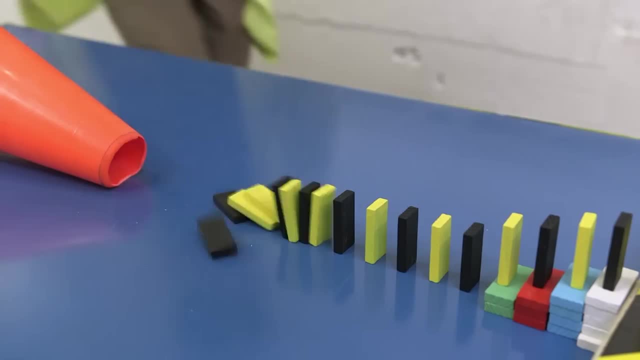 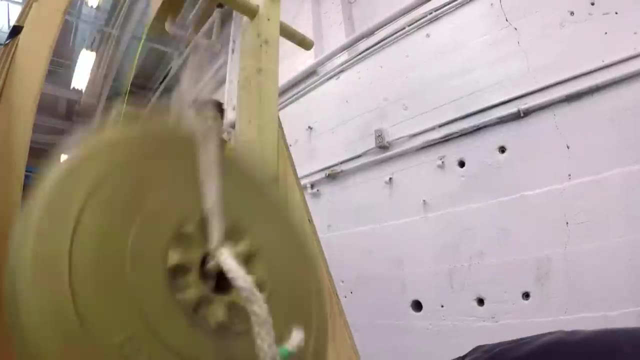 which transfers to some stacked dominoes. They fall in a chain reaction, finally causing bigger and bigger dominoes to fall, giving the last domino enough mass to pull a string. attach through some pulleys. quick release on a trebuchet. 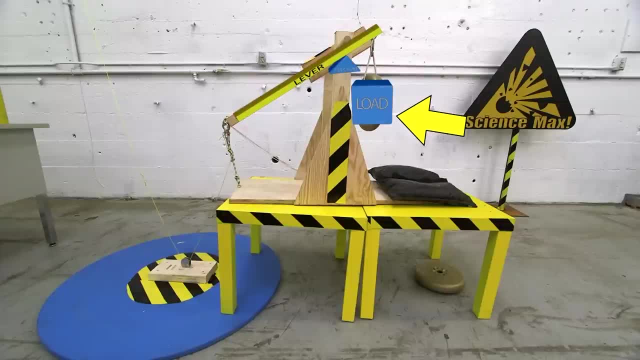 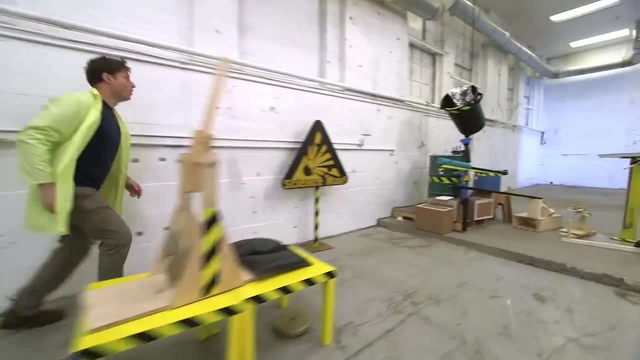 Now a trebuchet is a first-class lever with a weight on one side and a sling and a ball on the other. If the weight falls, the sling releases the ball at the right moment and it sails through the air. It's caught in a garbage can and changes directions. 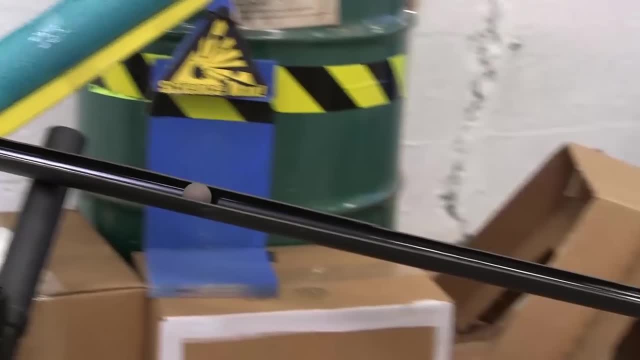 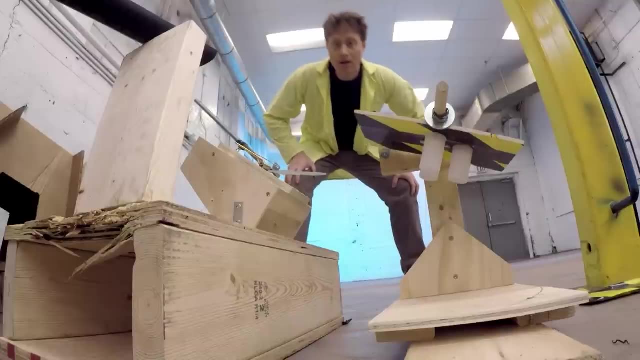 on a few ramps and another lever as a teeter-totter. Finally it falls onto a rat trap which has more energy stored in the tension of the spring. The rat trap smacks another lever which flips around, turning over some antacid rockets. 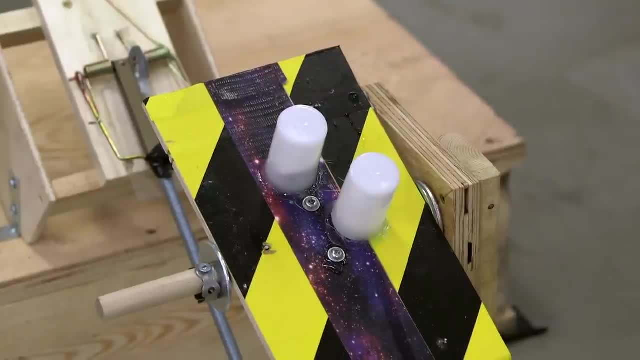 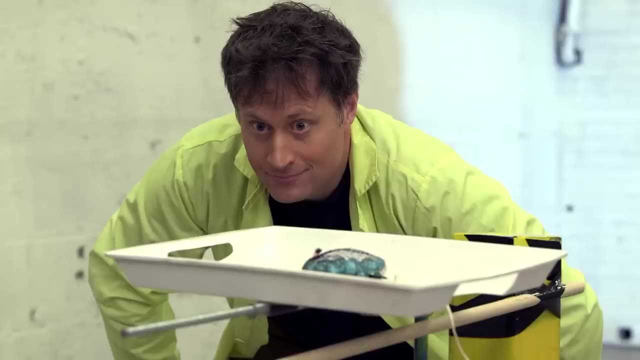 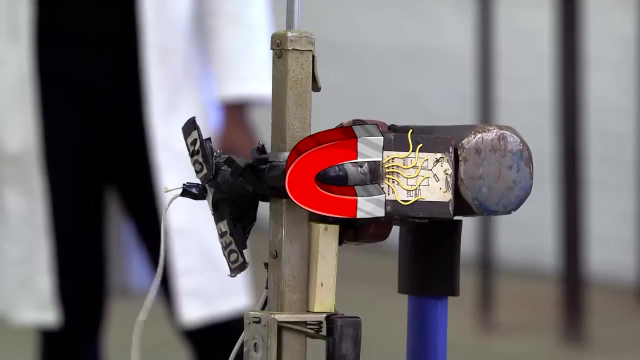 This allows the antacid to mix with the water and start a chemical reaction that produces carbon dioxide, which eventually builds up enough pressure to fire the container to another lever, which tips dropping some marbles on a string attached to a switch That turns off the electricity to our electromagnet. 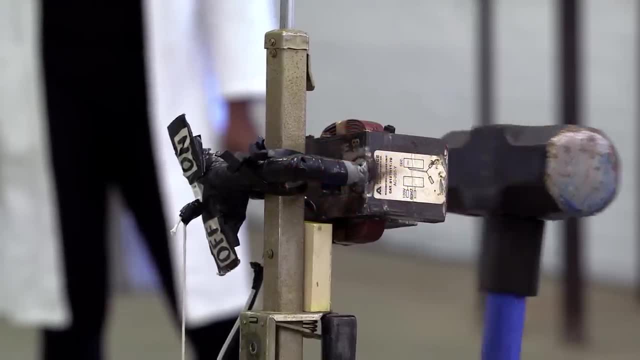 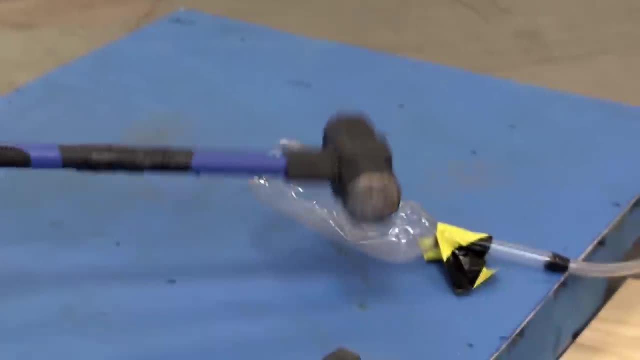 And when an electromagnet doesn't have electricity, it stops being a magnet, So our sledgehammer starts to fall. Now our sledgehammer is heavy, so it has both mass and speed when it hits this plastic bottle. All that inertia crushes the bottle, reducing its volume. 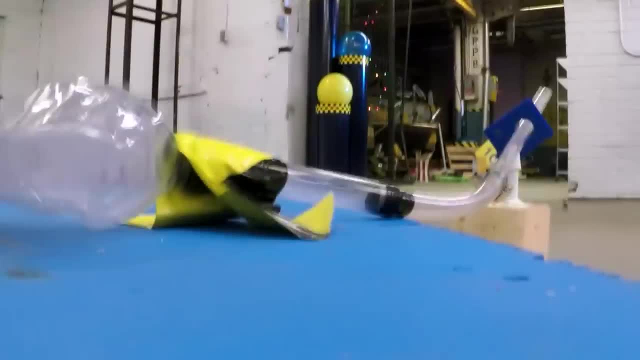 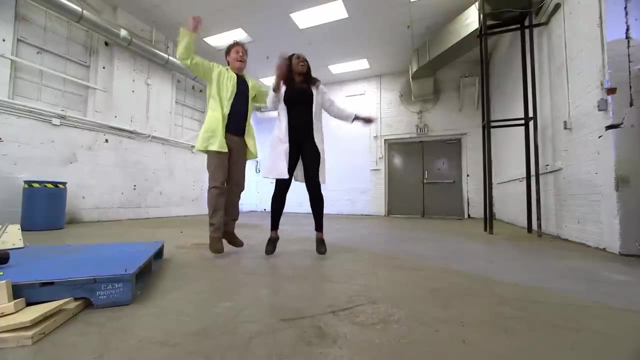 The air gets put under pressure and pushes out through a tube, which takes our stomp rocket with it. The stomp rocket flies through the air and hits our cake button, which then portals in some cake. Uh-oh, Uh huh. 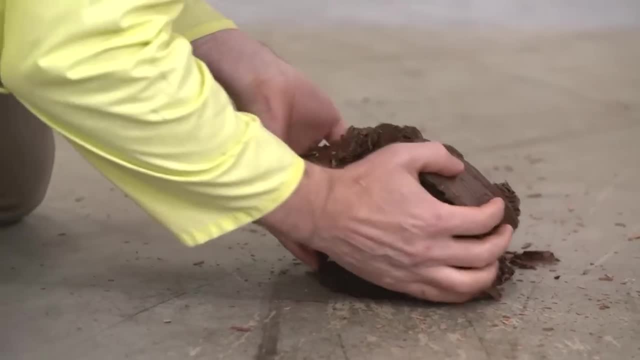 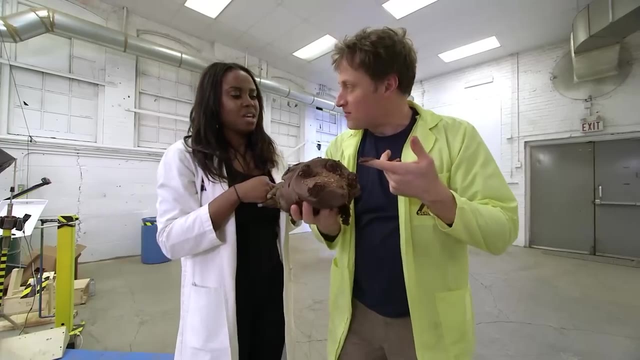 Guess we really didn't think that through huh, The cake should have landed on a table or something. Table would have been nice. There you go: ScienceMax Experiments At Large- Rube Goldberg machine. Are you sure you don't want some of this cake? 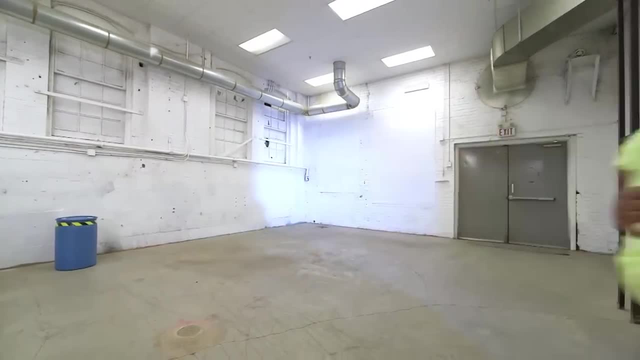 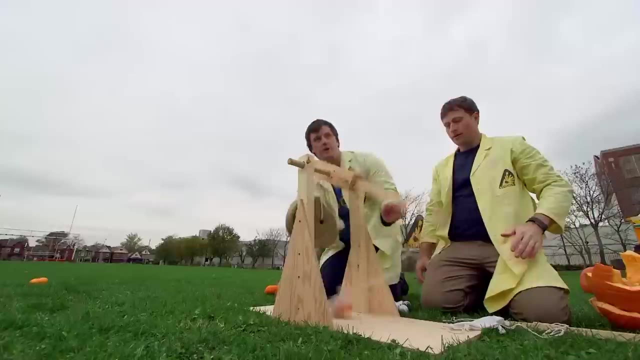 No, let's, let's go, But, but Let's go, Uh uh. This episode is all about mechanical advantage. No longer will I suffer the weakness of human muscles, Using the power of science to hurl pumpkins, pull cars, lift wheelbarrows. 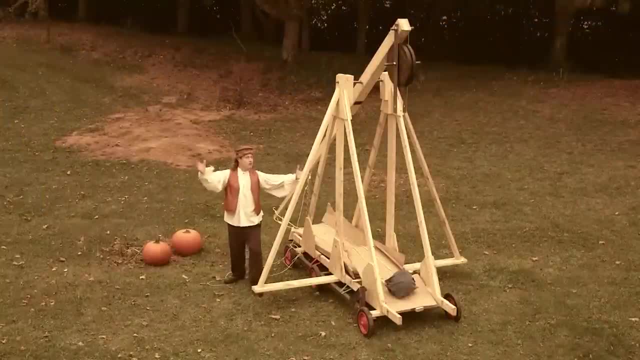 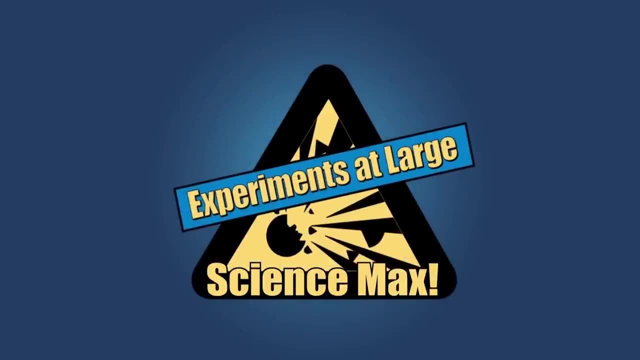 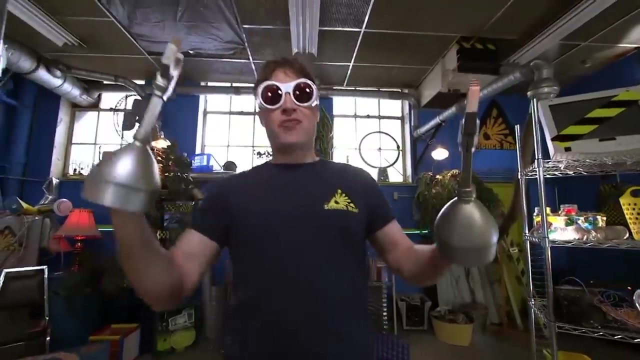 and um go back in time. A trebuchet- A what Trebuchet? All on this episode of ScienceMax Experiments. ScienceMax Experiments At Large. Behold Science Maximites. I am Filtron 2.0!. 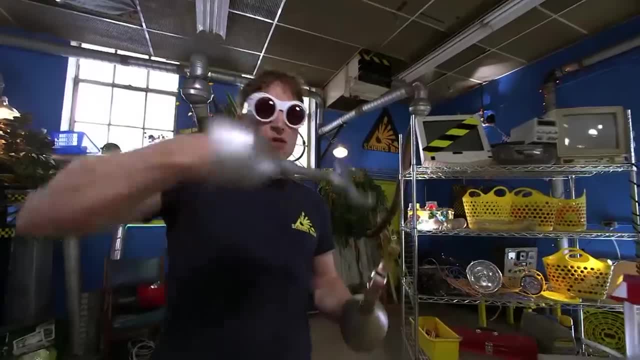 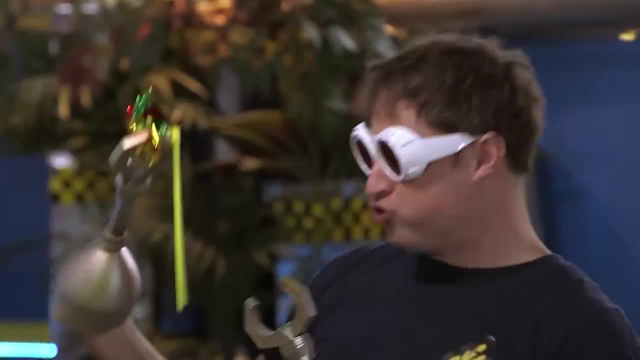 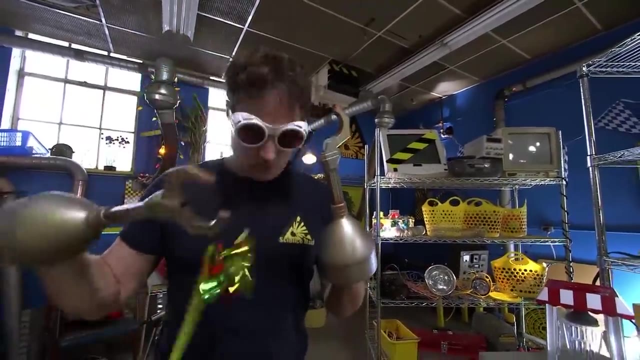 I have changed myself into a cyborg to give myself super strength. No longer will I suffer the weakness of human muscles. Behold my awesome strength. Tremble in fear at my might. I will, Hmm, Hmm, Hmm. I may have to give myself some upgrades. 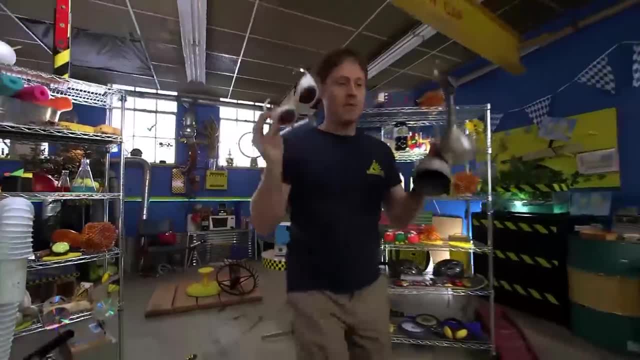 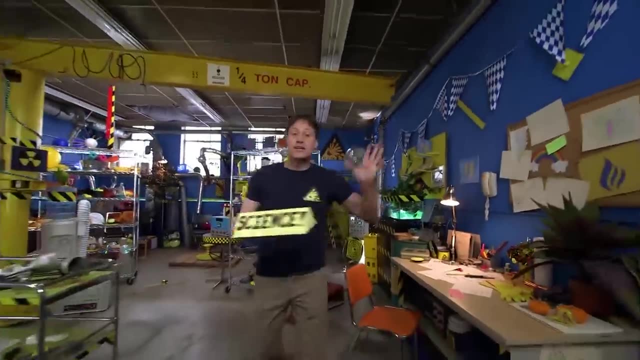 Uh yeah, so okay, Maybe I'll just give myself super strength. the old-fashioned way Using the power of science Today is all about mechanical advantage, like this fulcrum and this lever, Transferring a lot of force over a short distance. 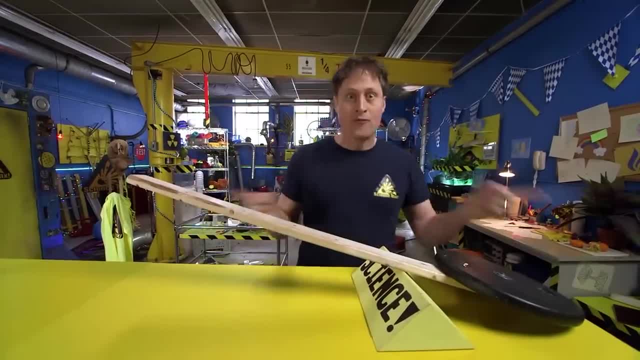 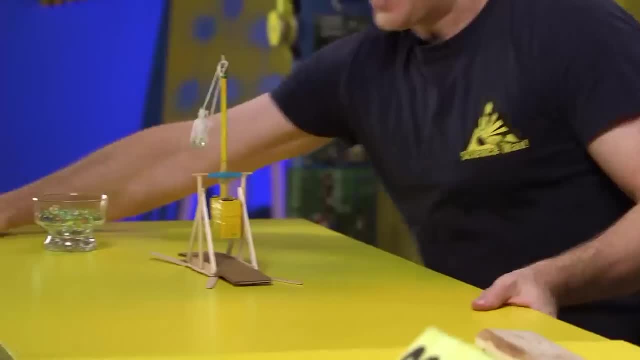 or a little bit of force over a long distance, and vice versa. We are going to be building a trebuchet, A trebuchet, So a trebuchet looks a lot like a catapult, but a catapult uses elastic force to throw something. 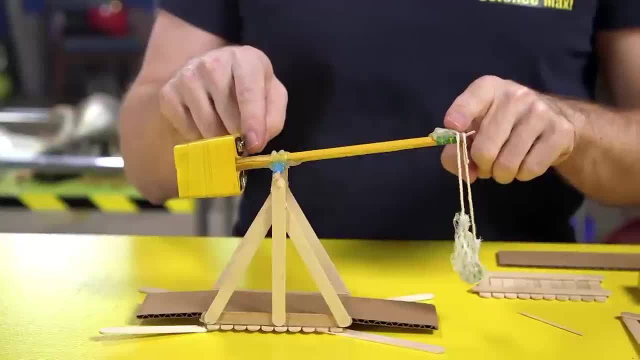 and a trebuchet uses the good old lever. There's a lot of weight on the short end of the lever and on the other side of the pivot is the long end, and we've got a sling here with a marble in it. 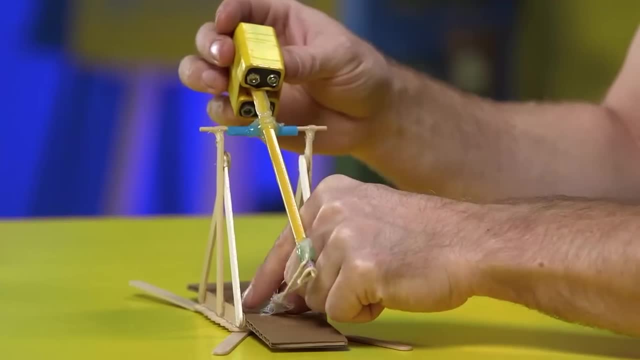 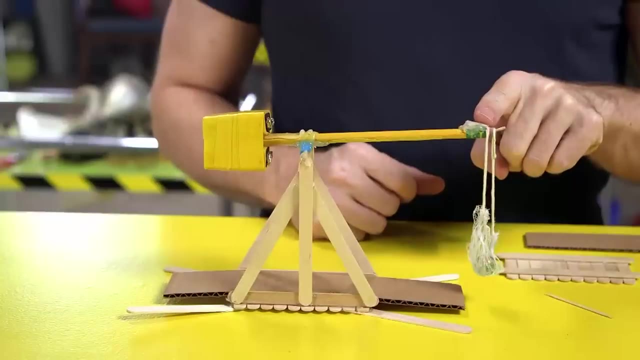 and we put that down here on the ground and then we let it go and whoosh, Whoosh, It throws the marble To build your trebuchet. here's what you need: Something to be your lever, like a pencil. 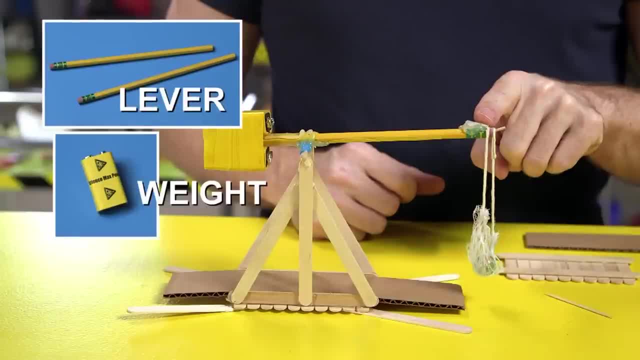 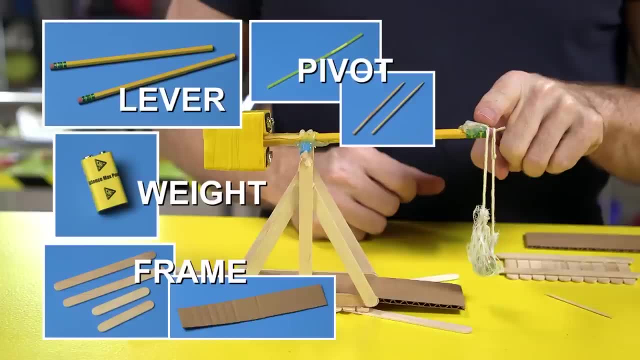 Something to be your weight. I use batteries. You'll need to make a frame and I use craft sticks and cardboard for that- A way for it to pivot like a straw and a shish kebab skewer. Then you'll want a sling, which is a rope. 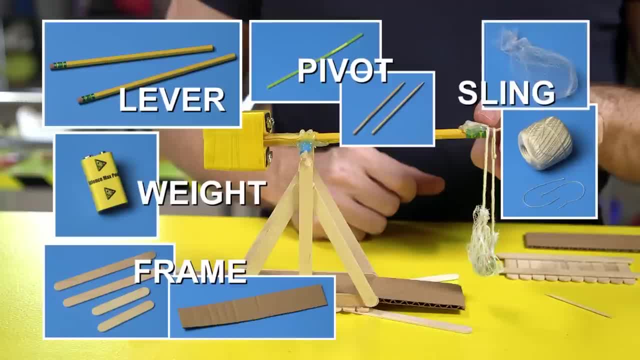 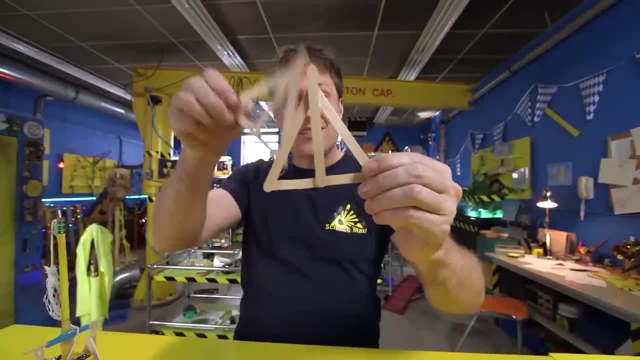 and something to hold your projectile, like plastic netting. Finally, something to hold it all together, like glue. Get your craft sticks, make some triangles with one craft stick sticking up. Then get your craft sticks and make a base, a base which you will put on with your cardboard, like that. 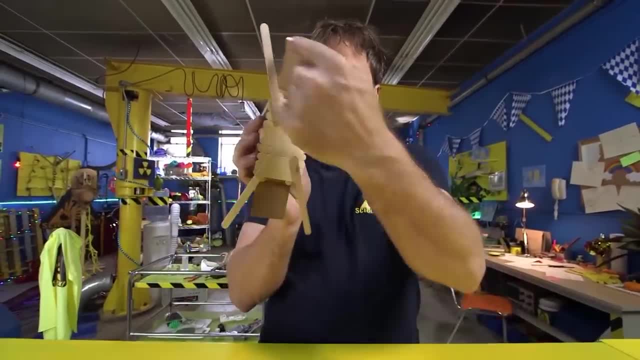 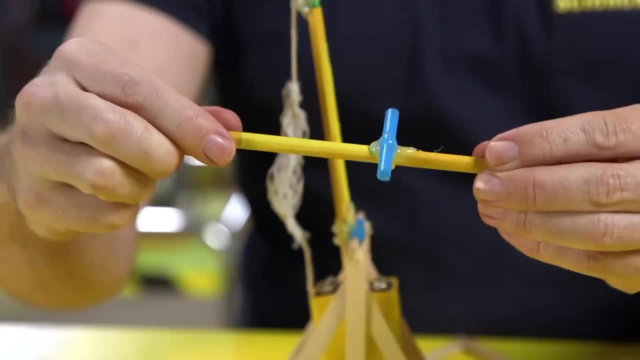 Now you'll also need to make a base, and you'll probably want to make some extra supports that go off the bottom there like that. Then get your pencil and cut a piece of straw so that you can see right through it and you can get a shish kebab skewer. 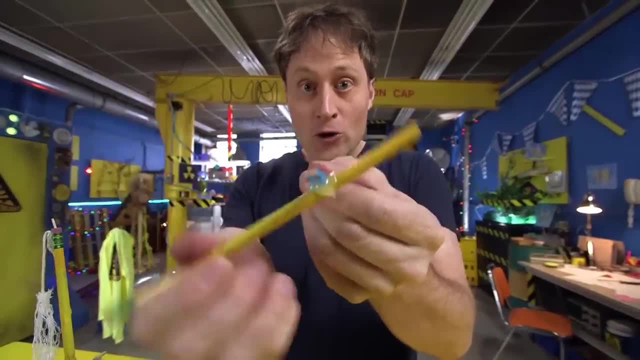 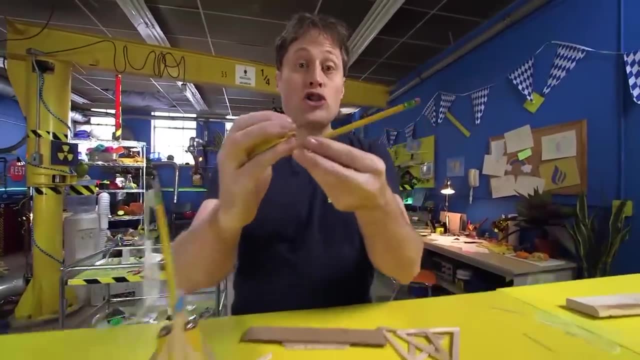 and you stick it through the straw like that and that's your pivot point, your fulcrum for your lever. What you want to do is put your weights- I've used some batteries, you can use anything that's heavy- on the short end of the lever. 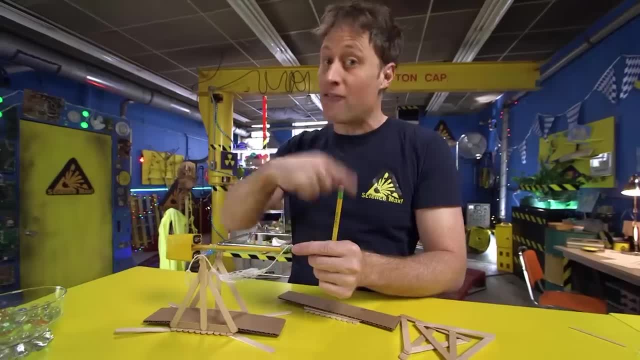 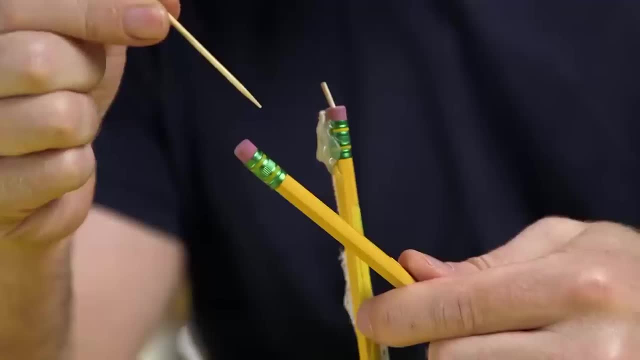 That's important, because a lot of weight here translates to a little bit of weight going a lot faster than your hands. So a lot of weight on the short end and then on the long end of the pencil where the eraser is. you want to take a toothpick. 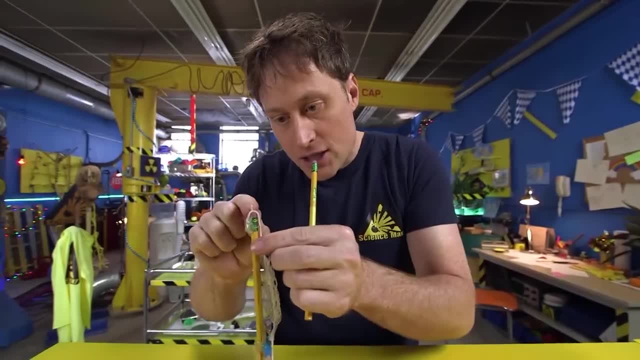 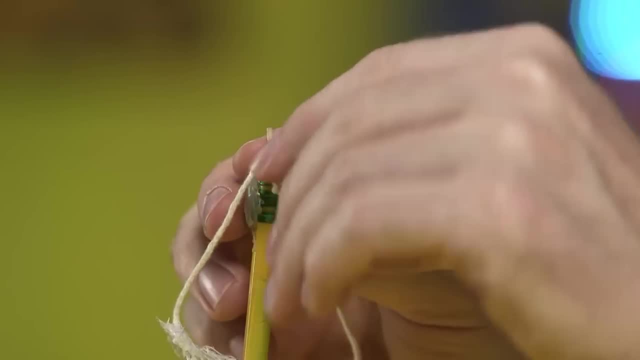 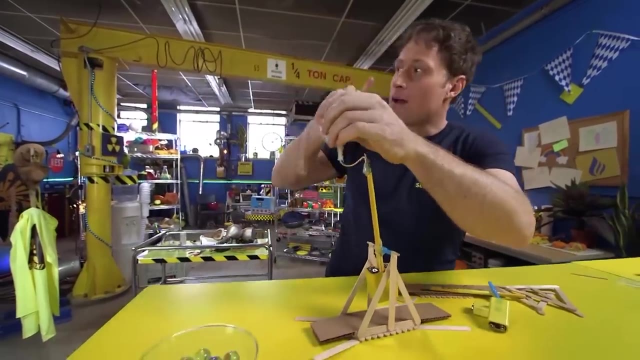 and stick it into the top of the eraser and then cut it off. so it's just like that That creates a little hook, that you put the loop of your string net on so that when it gets flipped around the loop comes off and then throws your projectile that way. 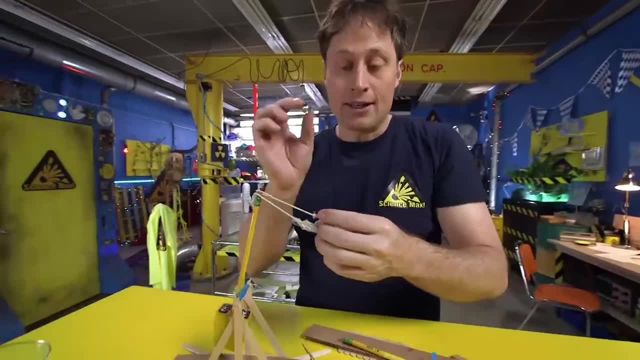 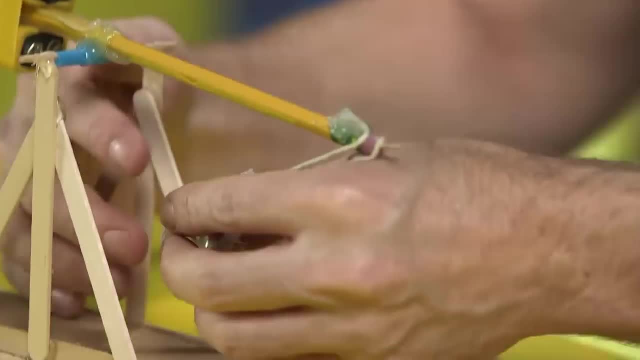 And then, of course, you need something that you want to fire. I like to use marbles, but gumdrops work pretty well because they're nice and soft And you put it in and you pull it all the way down, all the way, so it's actually resting. 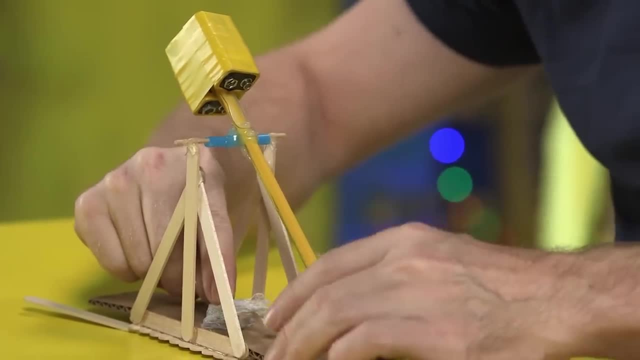 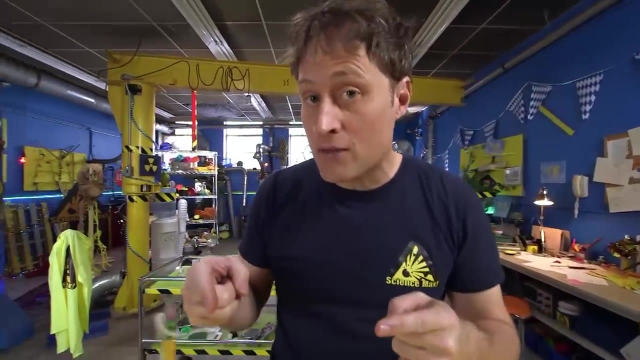 on the cardboard like this, and then you let it go And it fires, And there you go, A trebuchet. Now, if you want to research how to build one of these yourself, it is called a trebuchet, Ha ha. 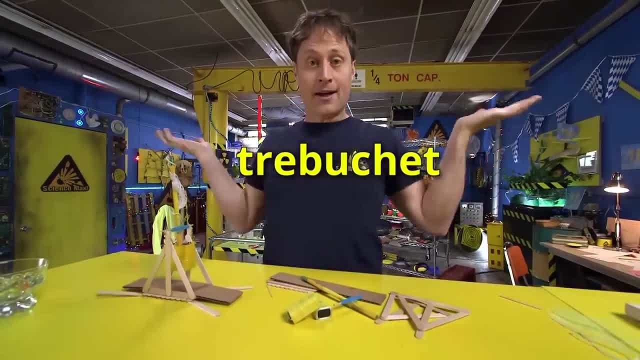 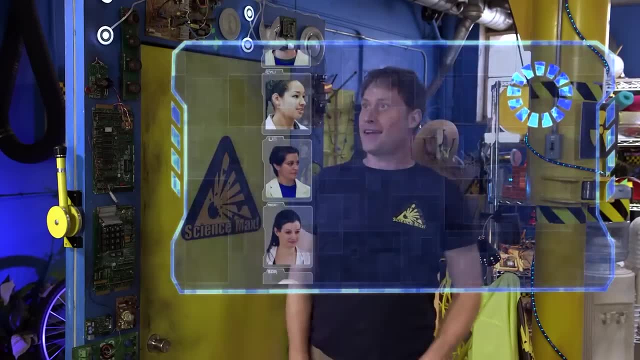 Trebu, I can make it come up, but I can't make it go away. I don't know why that works like that Anyway. So we need to max out the trebuchet. Let's see, I need an expert. 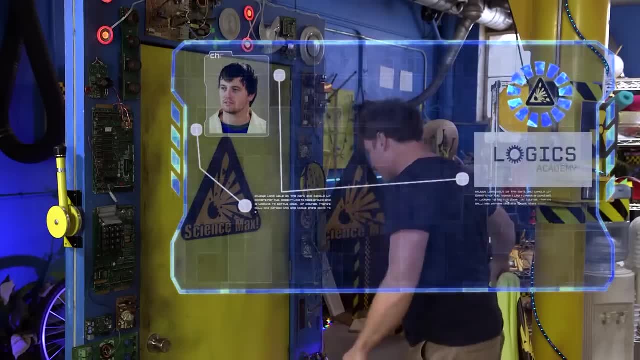 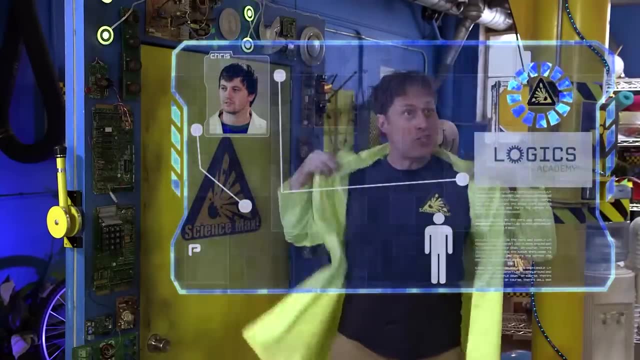 Um, Oh, Chris. Chris from Logix Academy has a trebuchet. Maybe we can use that one to figure out how we can max it out. And, of course, because it's a trebuchet and it's maxed out. 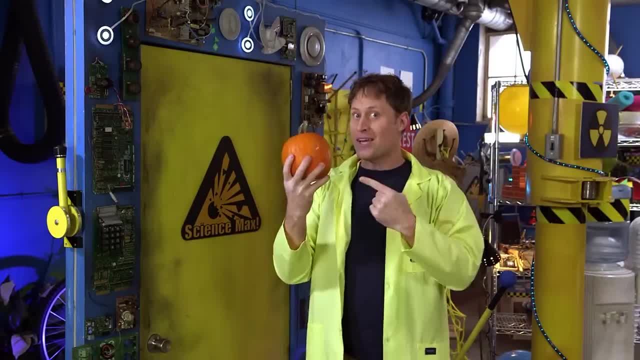 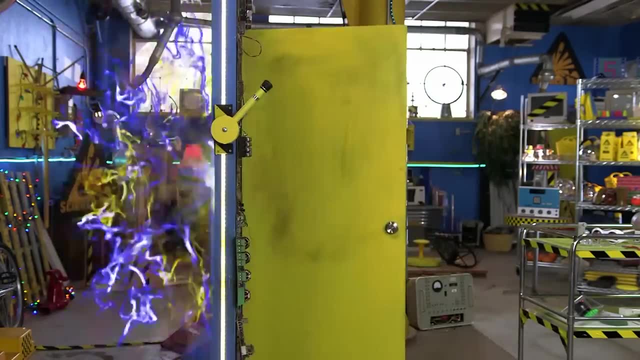 we want to fire something, so I thought we would fire. Ha ha, Pumpkins, Let's go. Good luck, little pumpkin. Hey Chris, Hey Phil. how's it going? Chris from Logix Academy, I uh had a problem with the pumpkin. 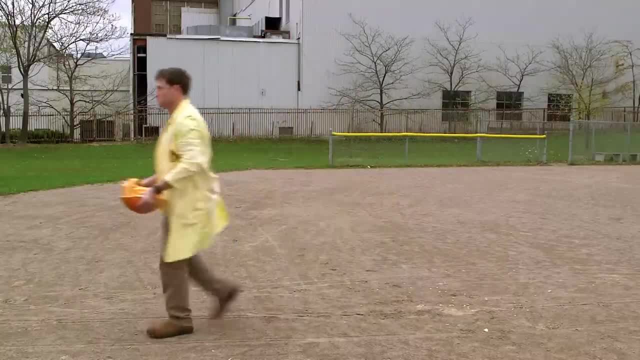 It kind of got larger than I expected. It's okay, I think this one's uh bigger than what we need. anyway, Chris shows me a scale model, trebuchet one we can use to test a few ideas before building our maxed-out version. 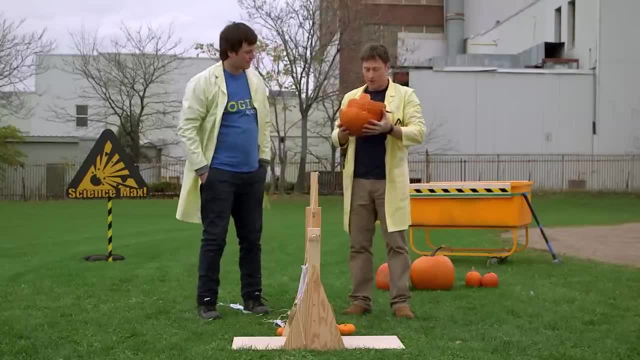 Oh, and you've got little mini-pumpkins. I know, Don't get, Ha ha ha, Don't get too attached. Oh, and you've got little mini-pumpkins, I know, Don't get, Ha ha ha. 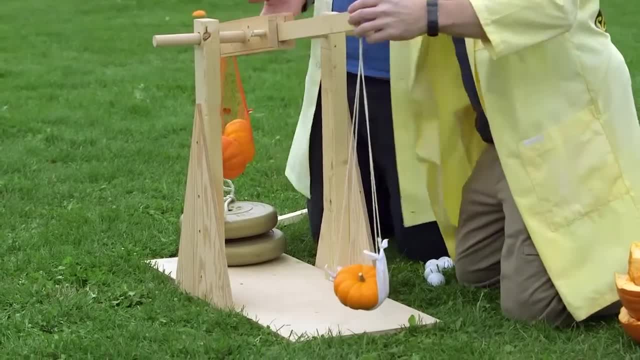 Don't get too attached. Oh, and you've got little mini-pumpkins I know Don't get Ha ha ha, Don't get too attached. The first is the arm length: getting the right ratio. That means how long one side. 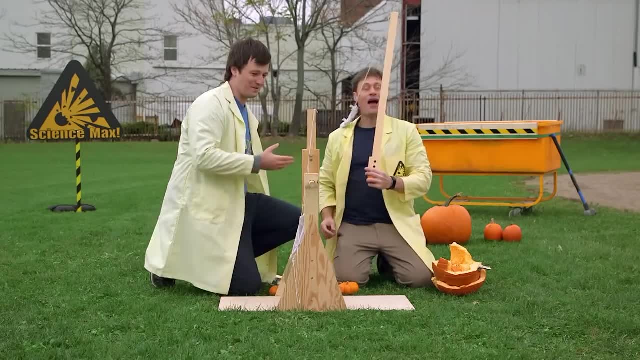 of the lever is compared to the other. When talking about a ratio, you write it like this: One to two. It doesn't matter what the actual measurement is, Just that this side of the lever is one of that measurement and this side 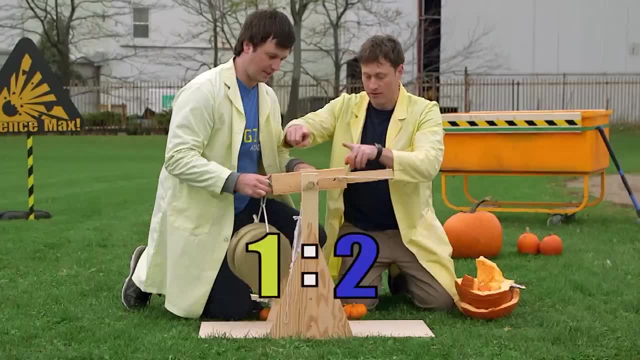 is two Or two times longer than this side, And it turns out a one to two ratio. arm wasn't great. Well, that's it for this episode. Thanks for watching. We'll see you next time. Bye, Bye, Have a good day. 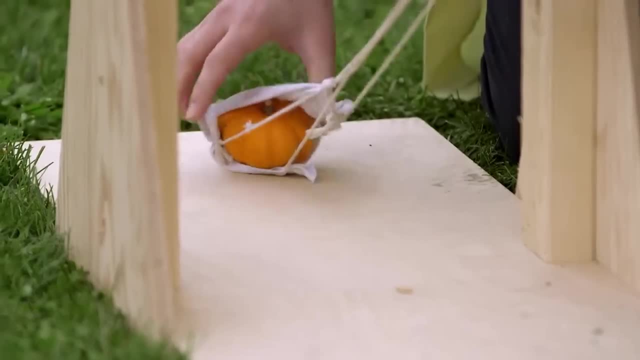 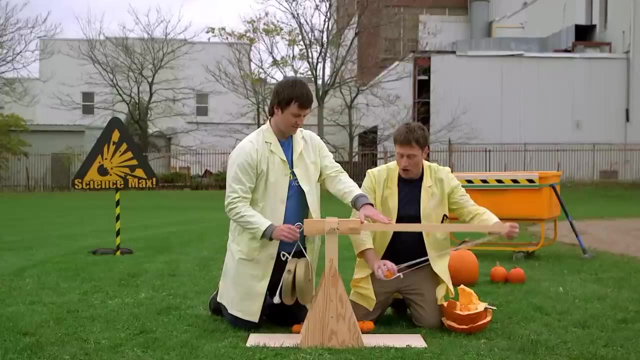 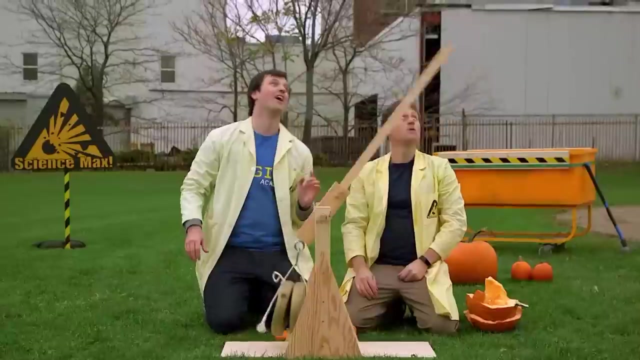 See you next time. Bye, Have a good day. Bye, Bye, Bye, Bye, Bye. Well, that could be better. It could be better. So we tried a 1 to 6 ratio arm. The 1 to 6 arm threw the pumpkin further. 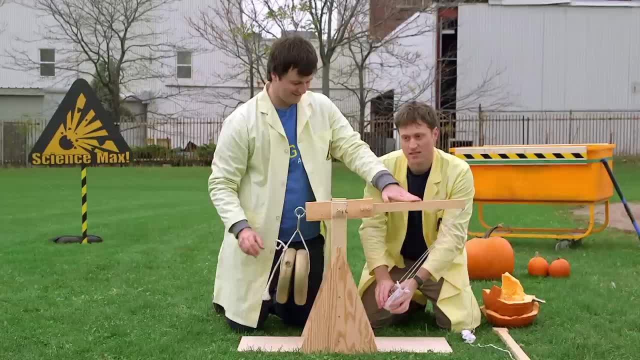 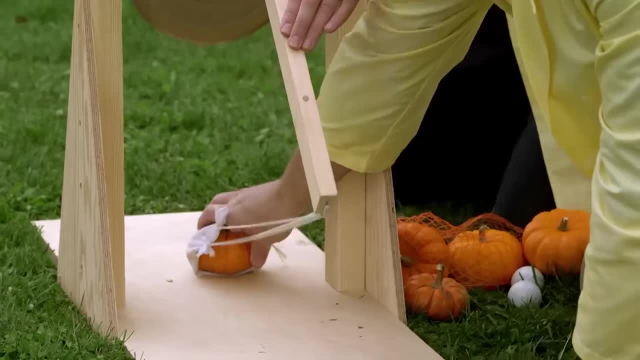 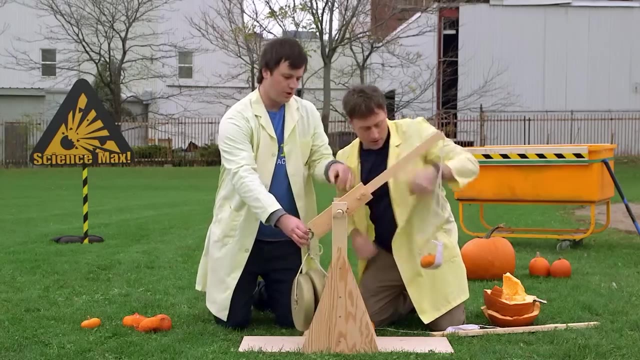 but not a lot further. Better, That's going to be better, Better. Then we tried a 1 to 4. Turns out 1 to 4 is the best arm ratio. Whoa, That's pretty good. Chris also had an idea about hanging the weights. 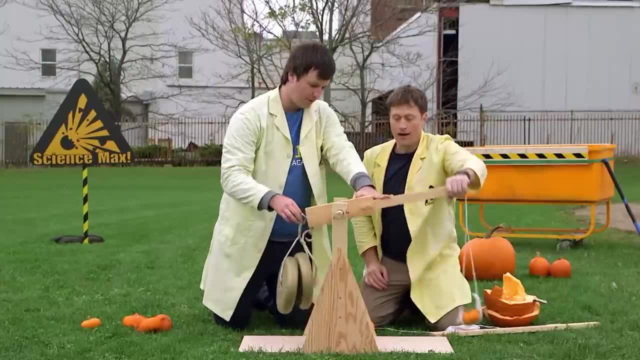 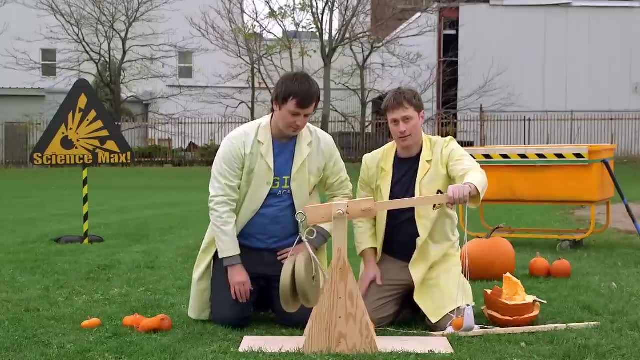 Because, as you see here, these go straight down, And going straight down actually makes this spin even faster. So when we do the big one, we should hang the weights off the end and not attach them to the end. That's right And that'll give you some extra distance. 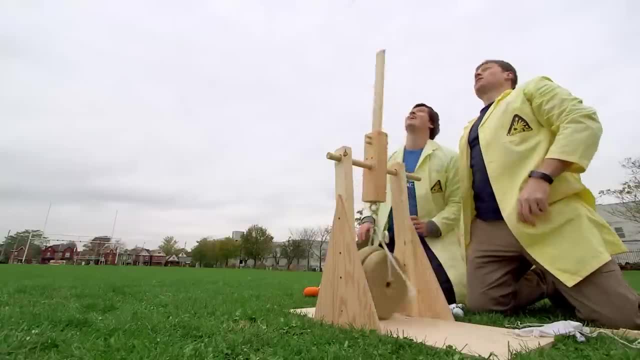 Excellent, Let's fire this last one. OK, 3, 2, 1.. Whoa, Pretty good. Yeah, OK, I wonder, when we make the big one, do you think we can get it through the goalposts? 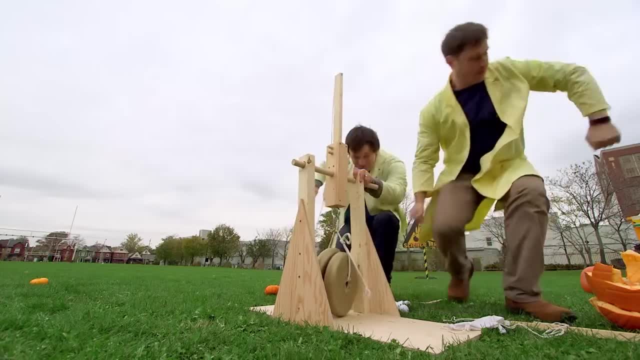 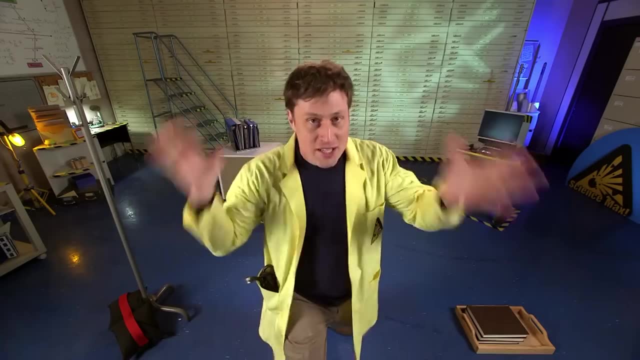 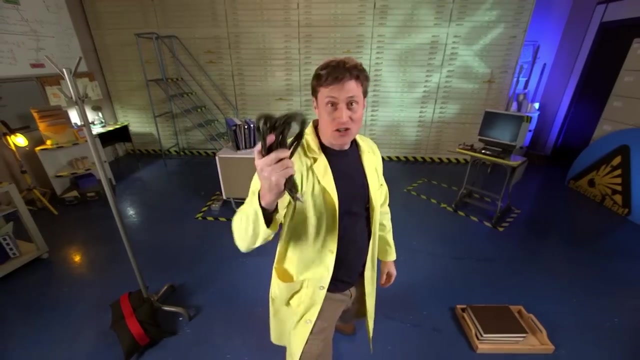 Oh yeah, I think we can do that. All right, let's try it. All right, This episode is all about giving yourself super strength using Mechanical Advantage. Well, here's how you can use a rope to give yourself the strength of a super hero. 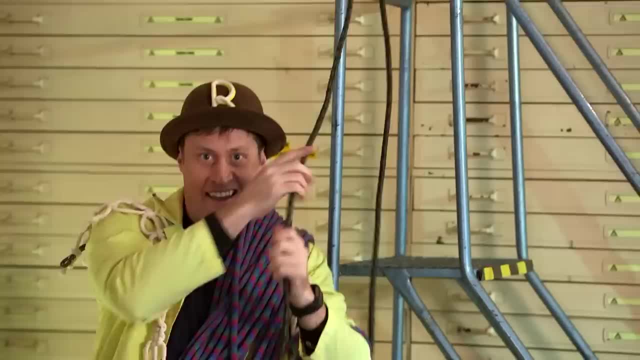 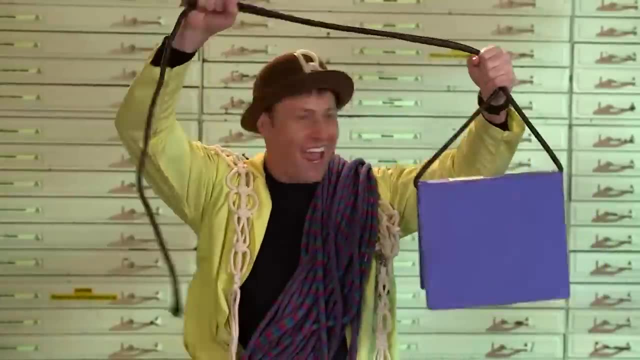 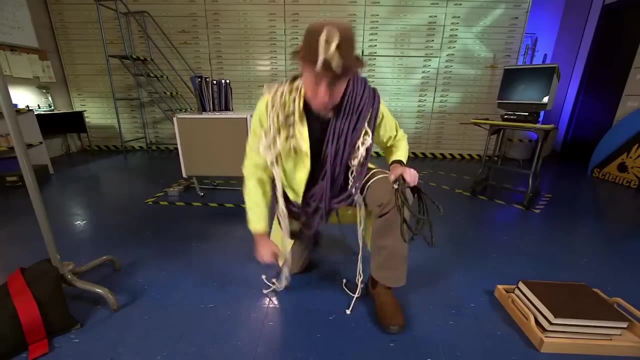 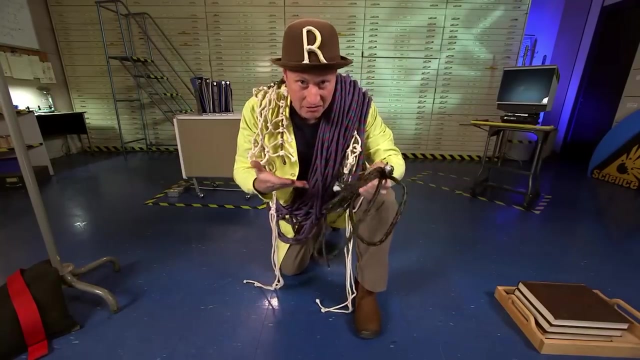 Ha-ha, I am Mechanical Advantage using a rope. man, To gain Mechanical Advantage using a rope, you need three things. First thing, a rope. I mean obviously that's a given right, You know you need a rope. 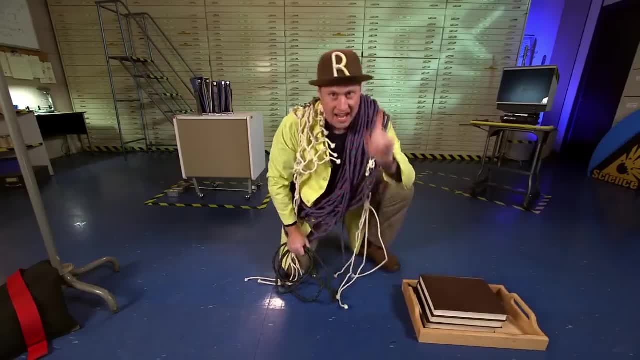 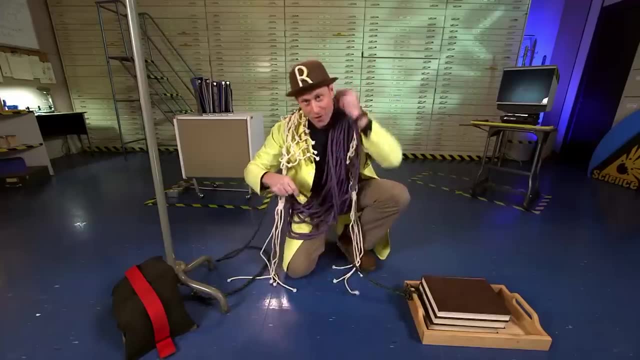 OK, good, Then you need something to pull, and something that will not move. What you do is you tie your rope to the thing that you want to pull, Then you tie the other end of the rope- you guessed it- to the thing that won't move. 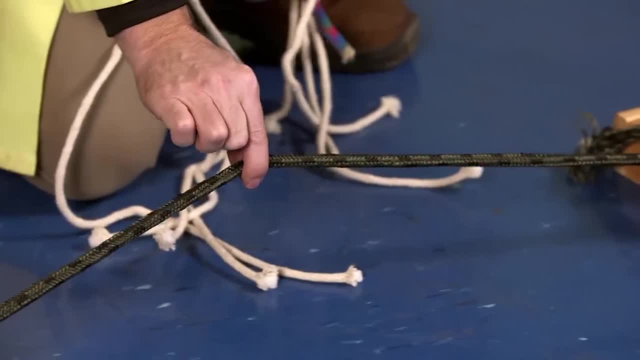 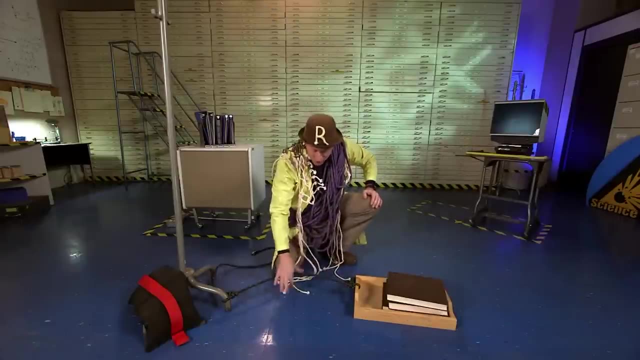 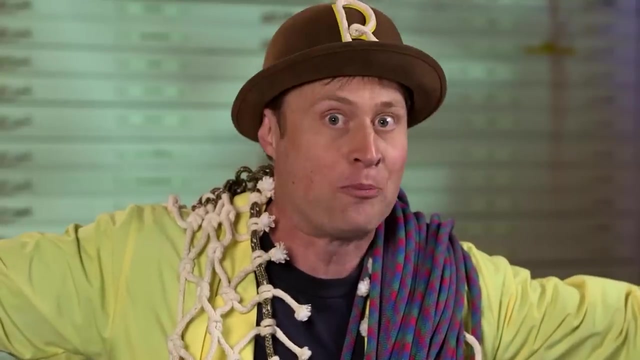 Now you pull from the middle like this: Ah, And it's very easy to pull the weight. Why? Because of Mechanical Advantage, You're using a small amount of force over a longer distance. But what if the weight is heavier? Then you lengthen the rope. 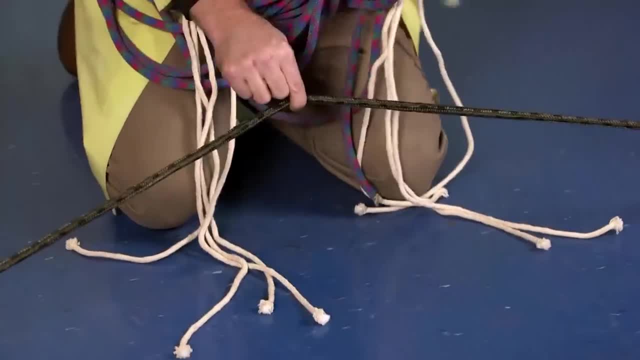 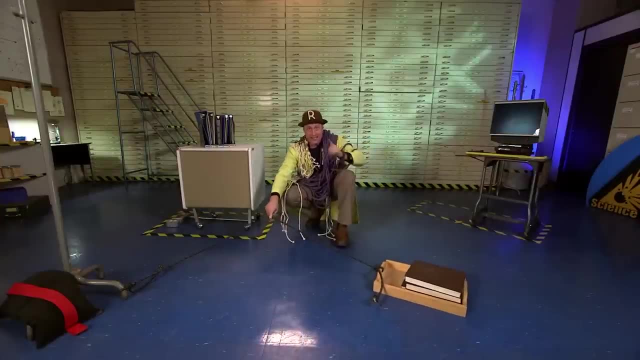 Now we pull from the middle and it's easier. Why Yes? Mechanical Advantage: A small amount of force over an even longer distance makes it easier to pull the weight. Let's max it out. Mechanical Advantage using a rope: man away. 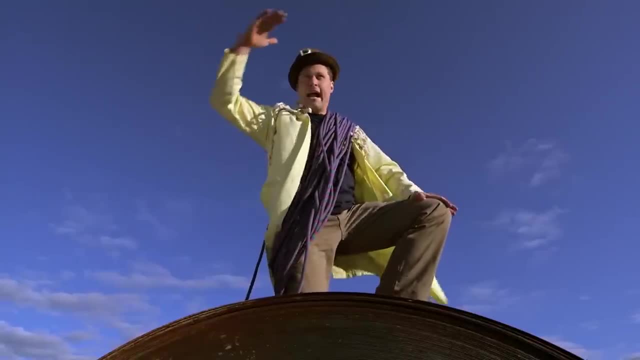 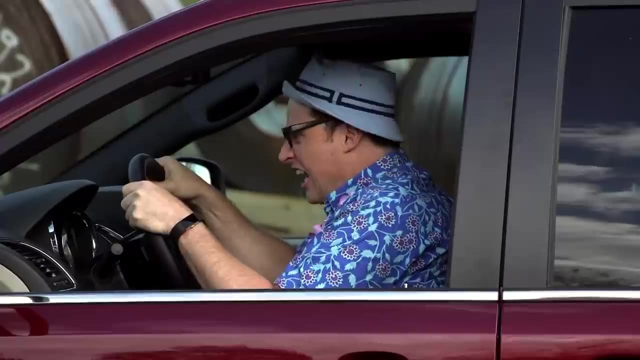 High above the city. Mechanical Advantage: using a rope, man surveys the town looking for someone in trouble. There's someone. Oh, my minivan broke down and only 10 feet from my parking spot. If only there was someone who could help me. 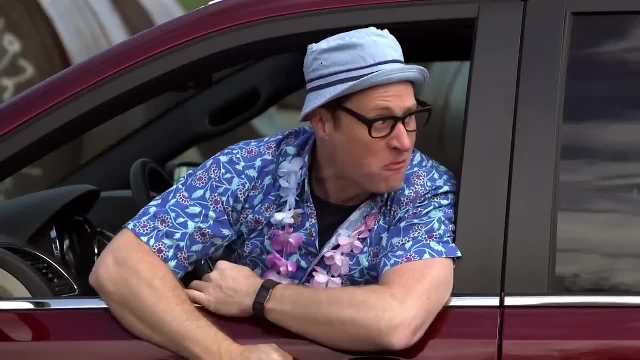 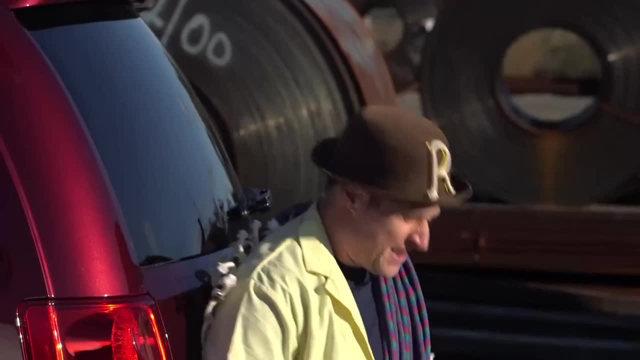 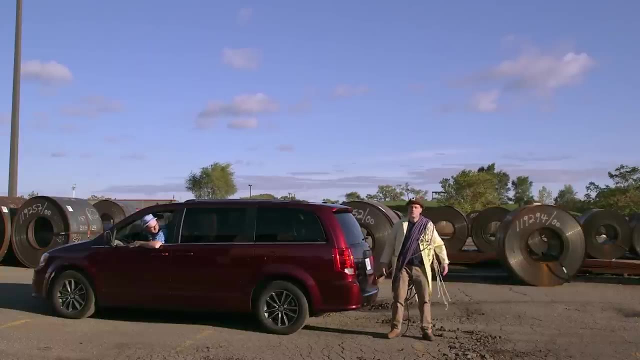 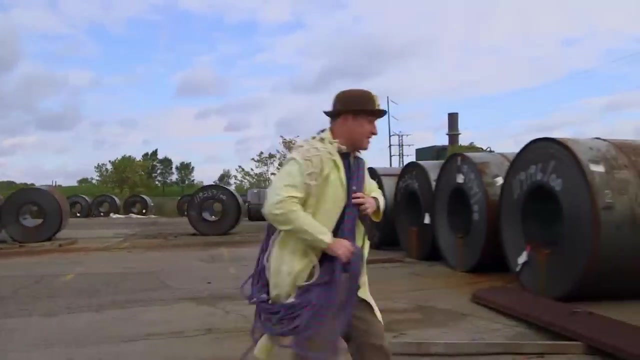 I'll help you, OK. Mechanical Advantage using a rope man. I'm saved. Maybe you should try giving yourself some Mechanical Advantage using the rope. Mechanical Advantage using a rope man. Yes, Well, I was coming to that. So I have this really long rope and I tie one end to something. 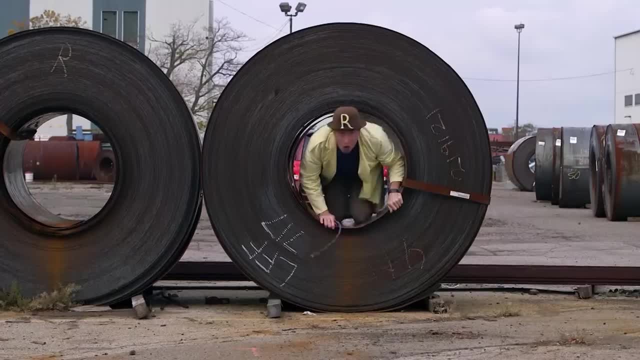 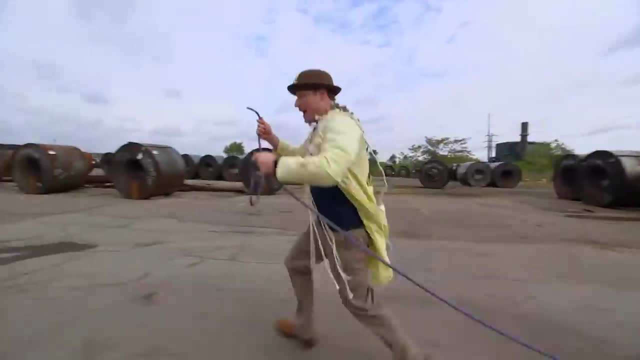 that's not going to move like a tree Or a steel coil- if you happen to have one- And then I take the other end and I run all the way back and I attach this end to the van. I call her Bessie. 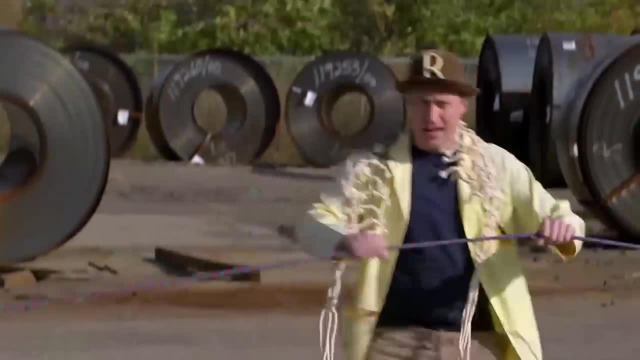 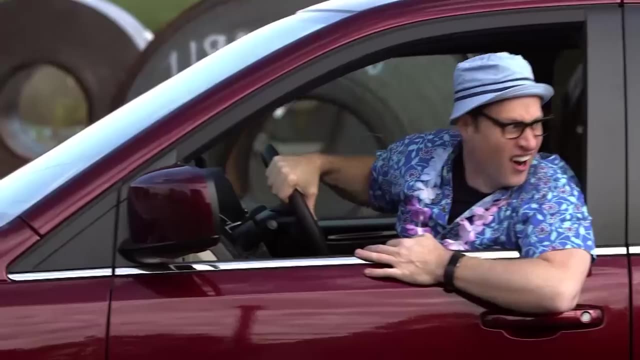 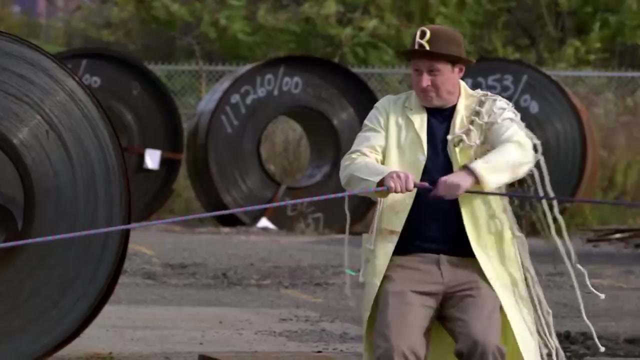 Then I go to the middle of the rope and I pull on it sideways like this, giving myself a huge amount of Mechanical Advantage. It's working. It's working. Pulling, pulling Mechanical Advantage using a rope- man, you're doing it. 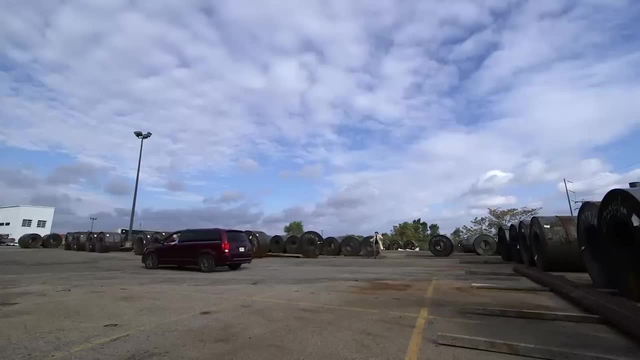 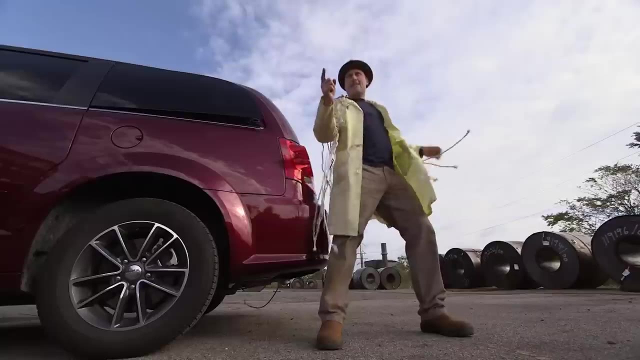 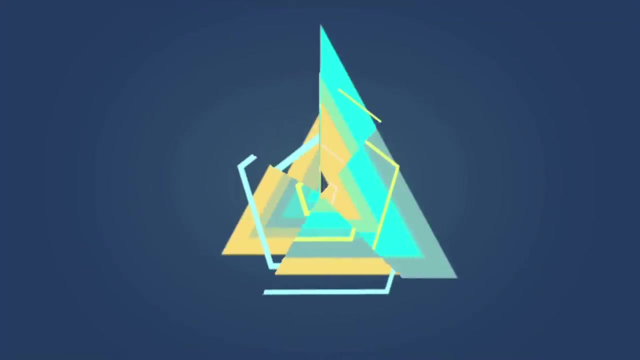 Well, gee willikers, you did it Mechanical Advantage using a rope man. You pulled the whole van And that's how you can use a rope to give yourself super strength. I am Mechanical Advantage using a rope man, Based on what we've learned from our small scale trebuchet. 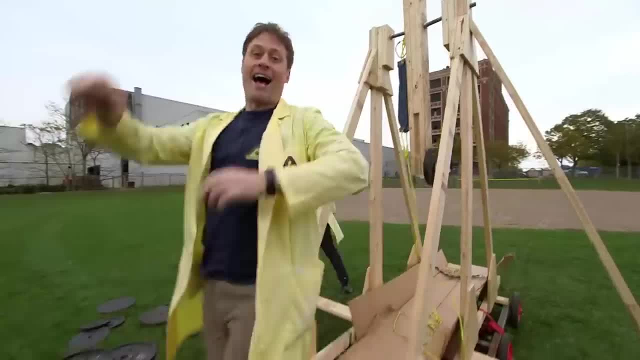 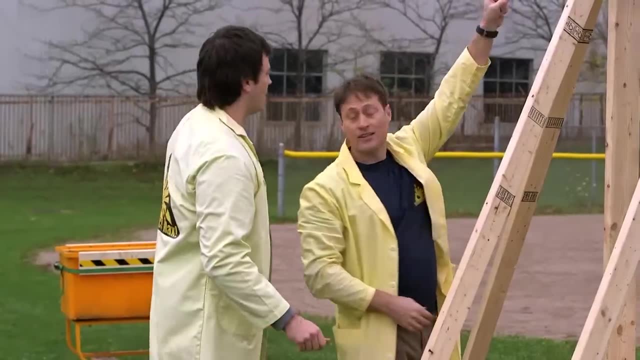 Chris and I made a maxed out version. All right, This, I think, is as big as we could possibly be. Wow, You could probably be expected to build this. This is huge. We have the length of our arm, which is important. 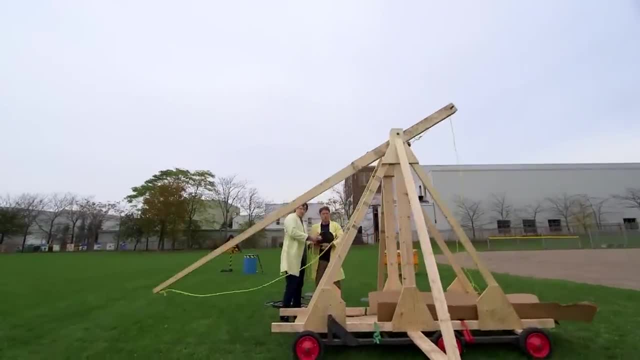 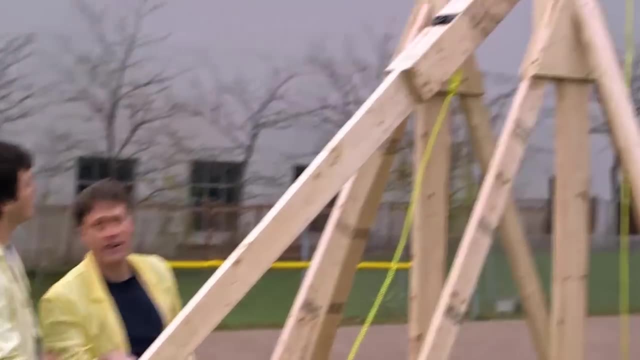 Yes, And we've got to add weight here, so we're going to loop this in: Whoa. Oh, I guess that's because I took the weight off. Yeah, So the arm is four times longer on this side of the lever. 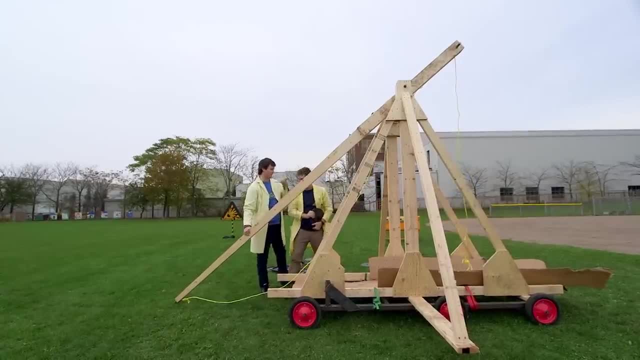 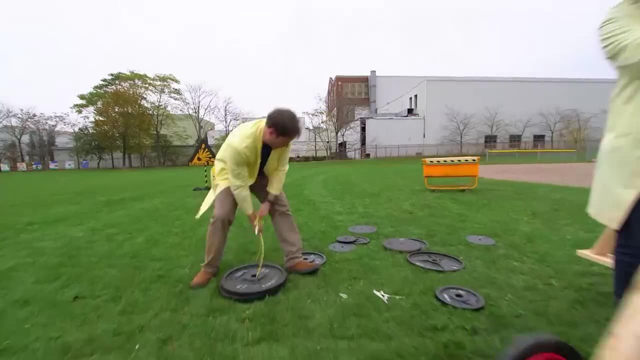 Right And on that side of the lever Right. So this arm goes four times faster than that side. But we're going to need a lot of weight. Like our small version, we needed to hang weights on the back of our trebuchet. 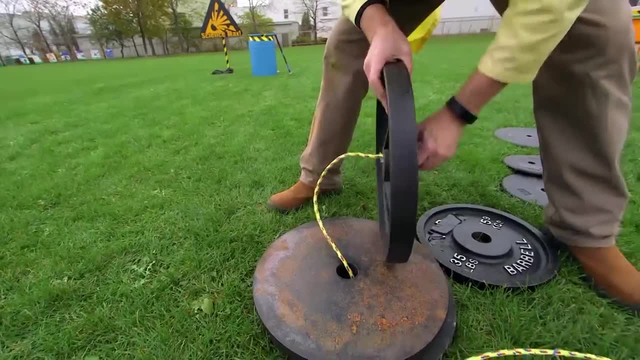 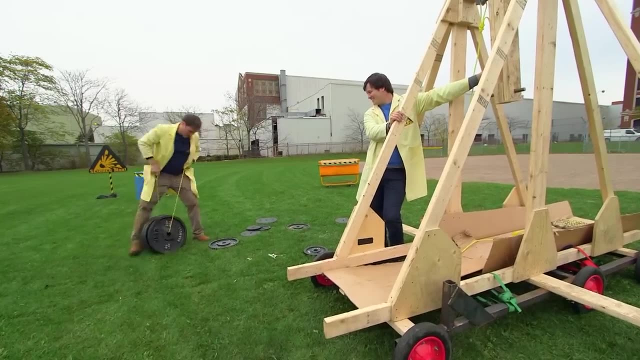 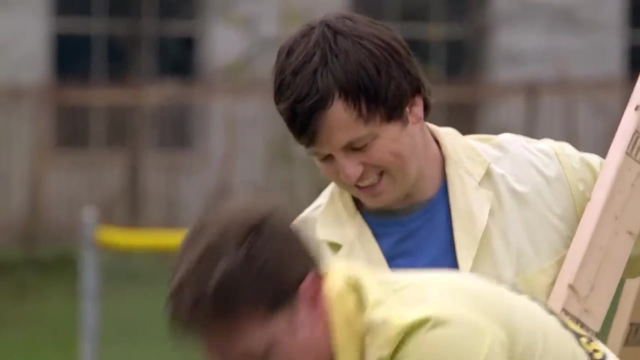 So I got a rope and put some weights on, but because our new version is so maxed out, we need a lot of weight, which I needed to get on a rope and drag it over- OK, Almost there- And I needed to lift it onto the arm. 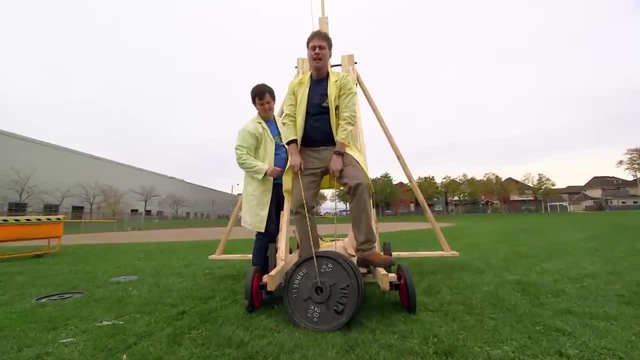 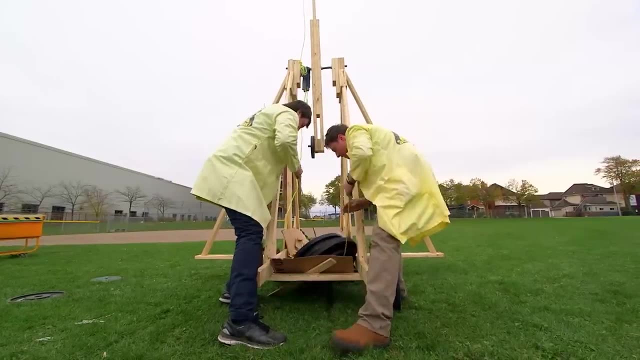 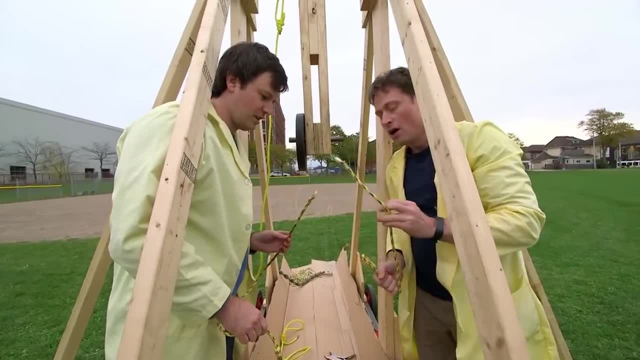 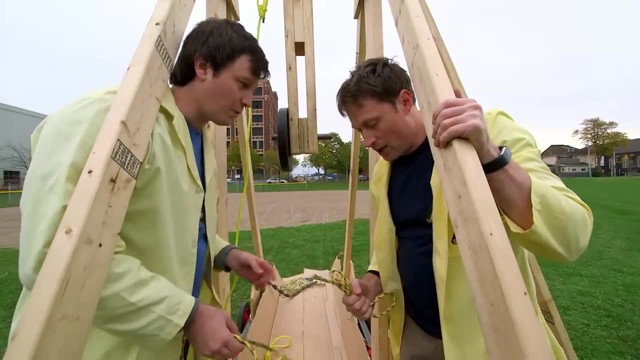 Yeah, That's going to be a problem, Phil. I'm kind of glad that happened, because there was no way I was going to be able to lift that. I know It was way too heavy And we need something stronger that can still hold the weight. 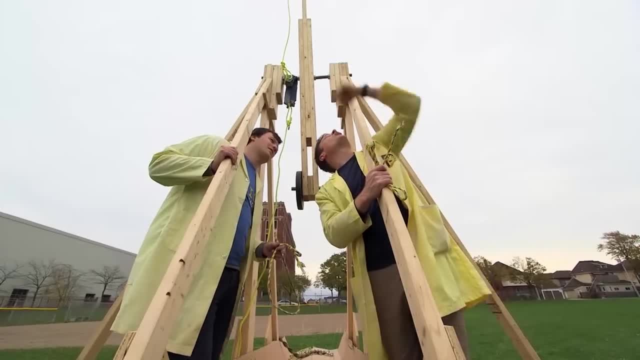 and still give us the hinge that we want at the top And once the weight's up there, if the rope broke, That would be bad news. That would be big time bad news. OK, So we need a new solution for getting the weights. 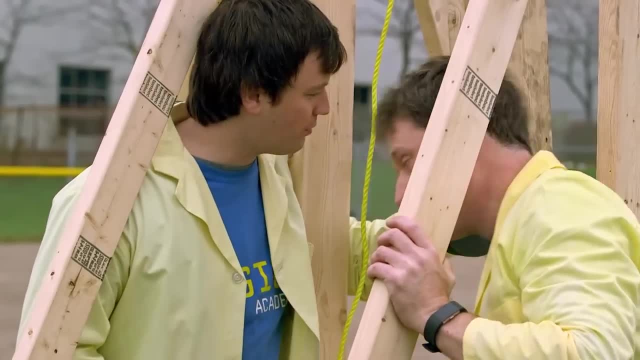 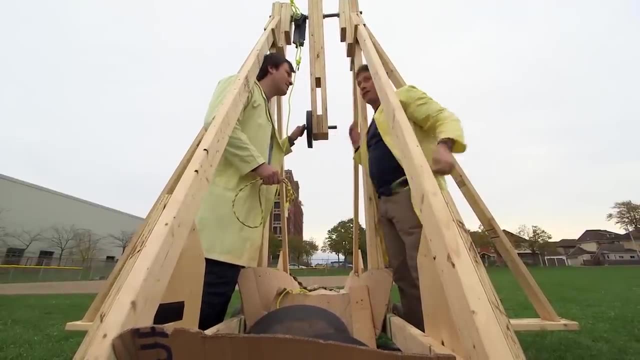 on the trebuchet. that is not Not rope. We need something stronger and hopefully that still has the hinge on it up here. Maybe we have some sort of bar system that we could hang. Yeah, I'm thinking metal. Yeah, like, yeah, metal. 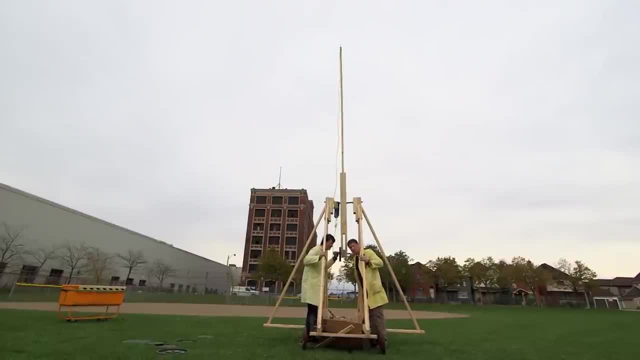 Definitely metal, Definitely metal. Metal is better than rope. I think so For holding a whole bunch of weight. OK, let's get that done. Let's do it. All right, I got some metal over in the shop over here. 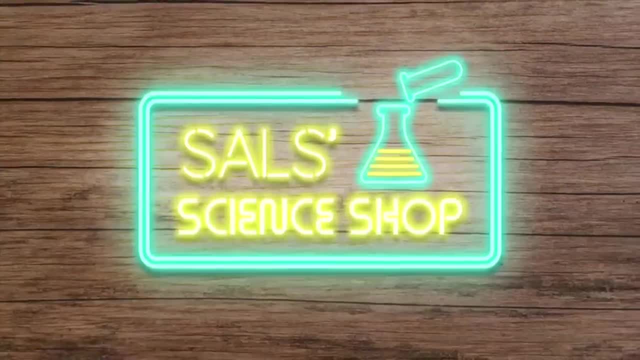 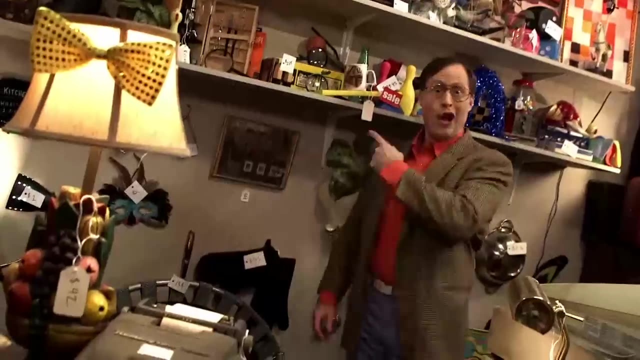 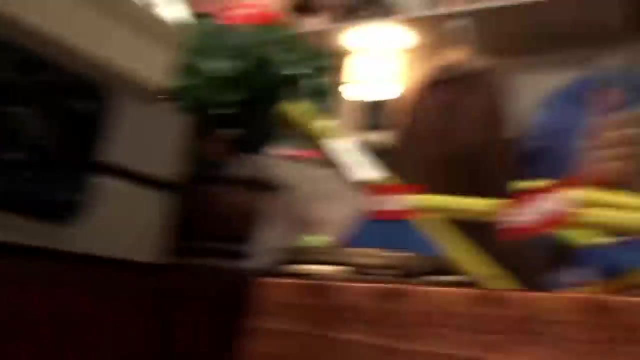 OK, Come on down to Sal's Science Shop. I am Sal and this is my science shop. You want levers? I got the best levers around: Little levers, big levers, all drastically reduced If you can find a lever anywhere. 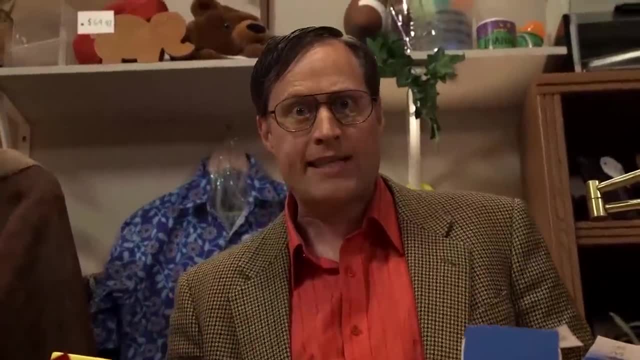 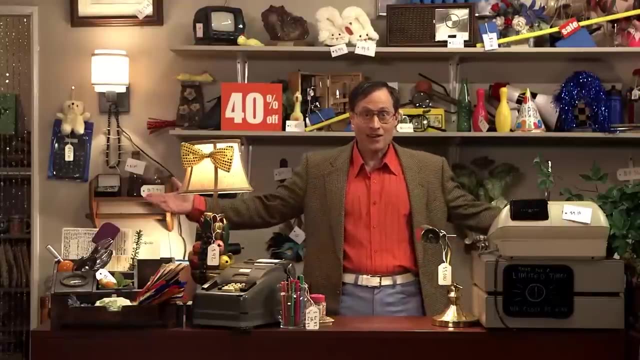 else for less. then you got to tell me, because I didn't know, anybody else was selling them. Come on down to Sal's Science Shop, your one-stop shop for science. Hey, you want some levers? Well, boom, have I got levers. 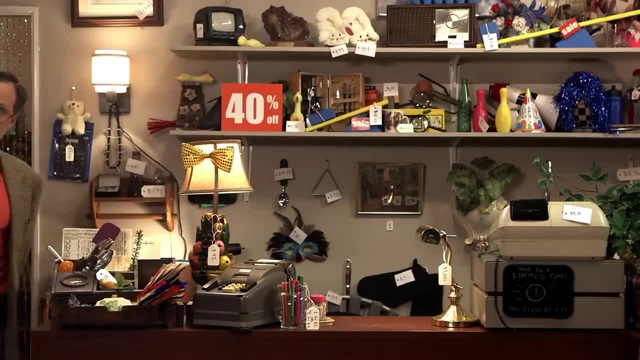 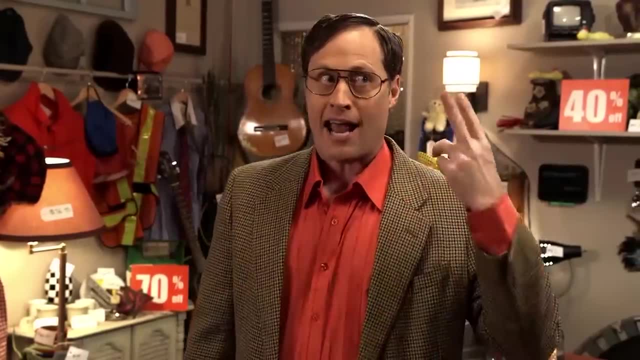 What class would you like? What's that? You didn't know that levers have different classes. Well, there are three different classes of levers: First class, business class and coach. No. first class, second class, third class. 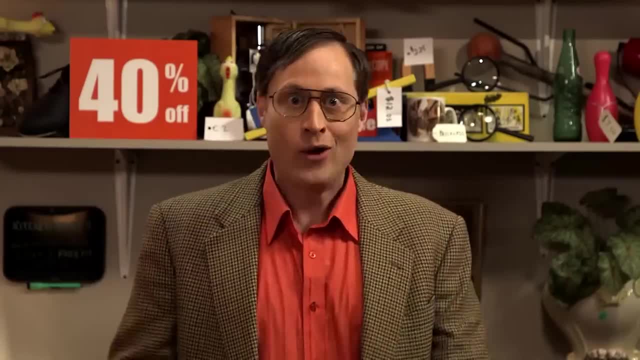 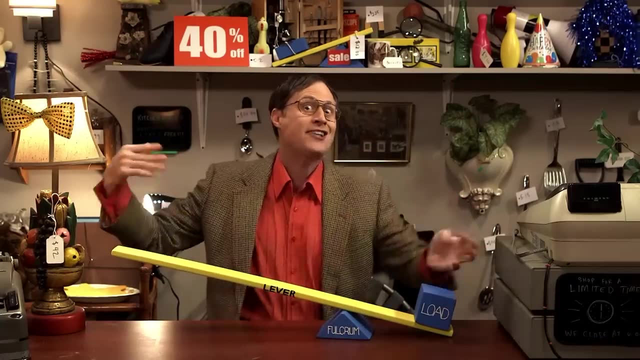 It's pretty straightforward. And what do we need when we have a lever? We need a load, we need a fulcrum and we need a lever. Ha ha, first class lever, the fanciest of levers. You got your load on this end. 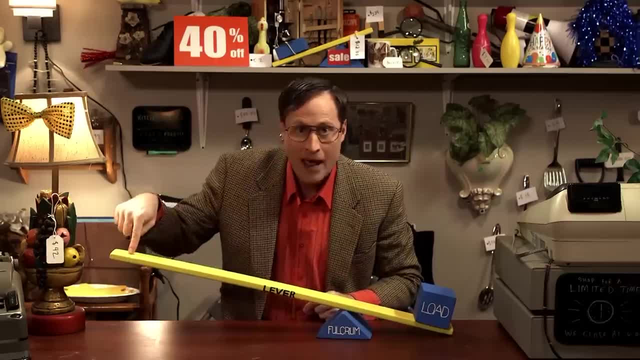 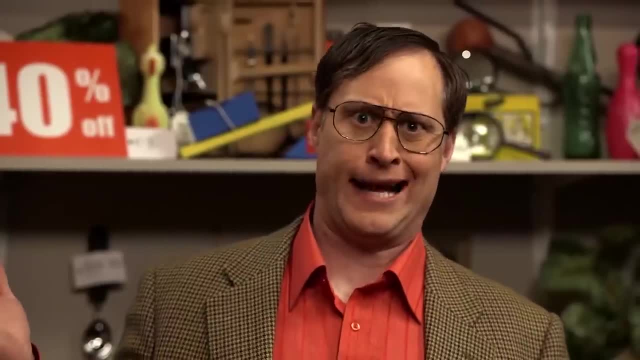 You got your fulcrum right here underneath And then you put some effort into this end And wow, look how easy that is. Ha ha, first class. What kind of thing works like that? Oh, I don't know How about this trebuchet? you've been 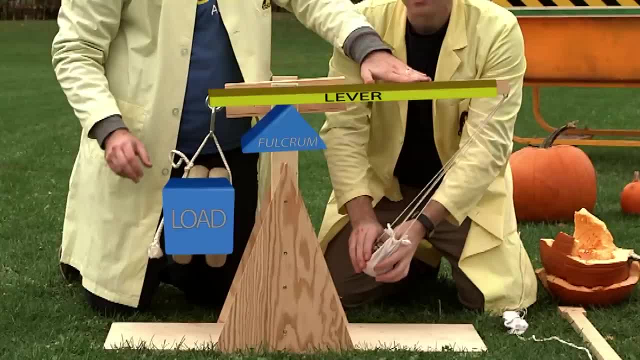 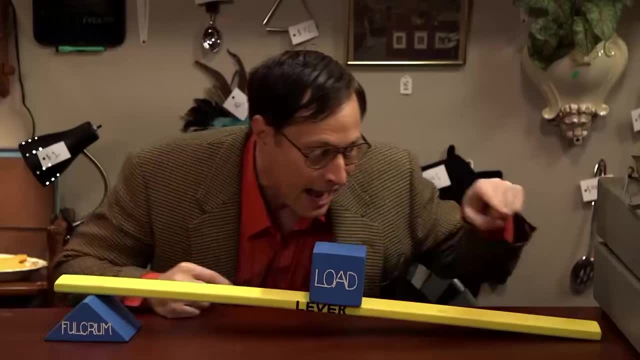 spending all this time watching First class, Second class lever right there in front of you. Second class lever- Look, there's a load right here in the middle. The fulcrum's on this end And you put your effort into this end. 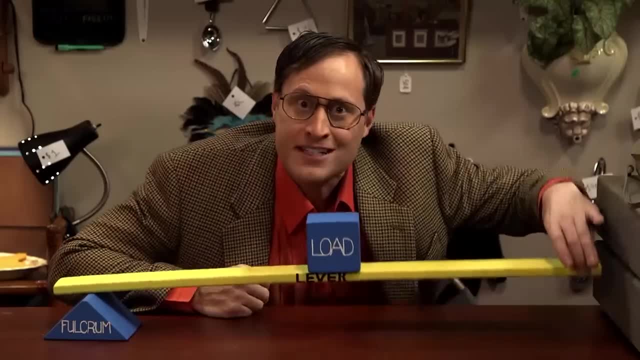 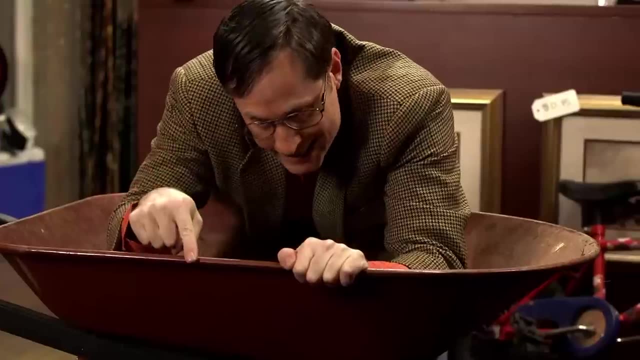 And you lift it and look it's a second class lever. Ha, how cute is that. But what kind of thing works like that? It's like a wheelbarrow. The fulcrum is the wheel. The load goes in this. I guess this is the barrow. 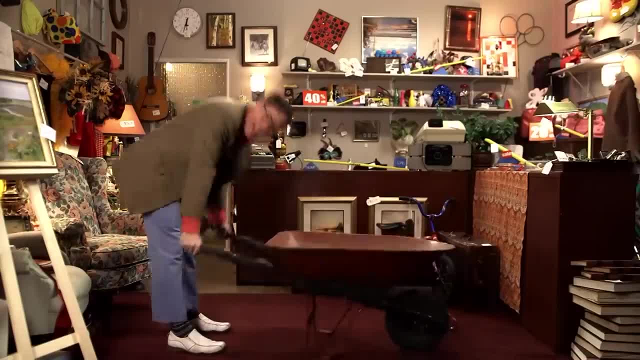 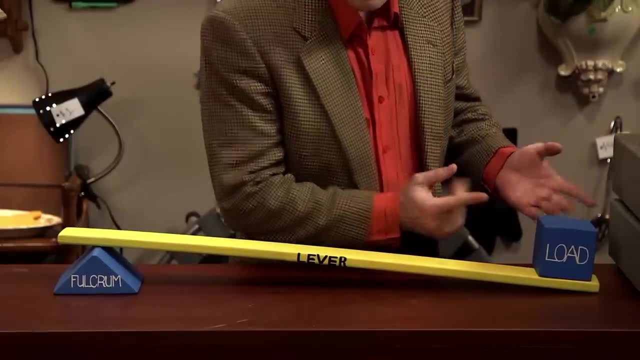 And then I lift with the handles: Ha, look at that. Ha lever. Third class lever. You got your load on this end, You got your fulcrum on this end, But where is the effort? The effort's in the middle. 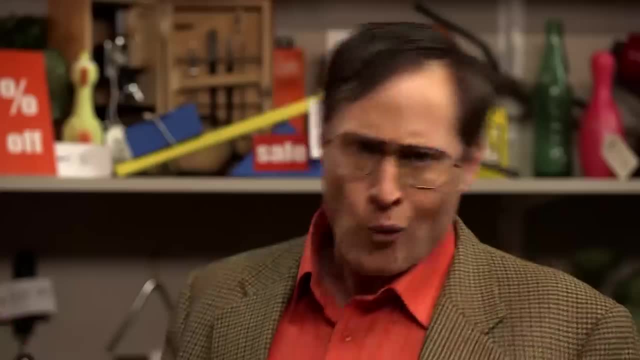 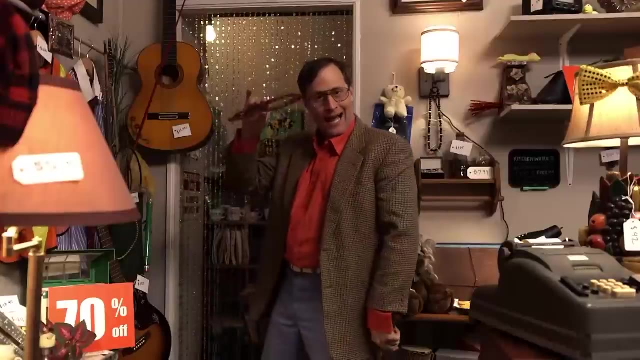 And it pivots while you move it. Huh Huh, Where are you going to get that kind of crazy contraption? Salad tongs, Salad tongs, Salad tongs. Look, you put the effort in in the middle there. 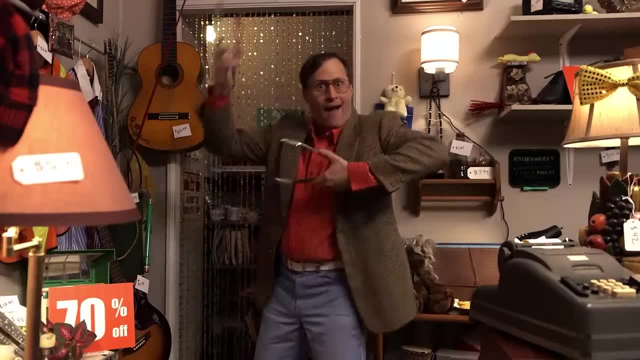 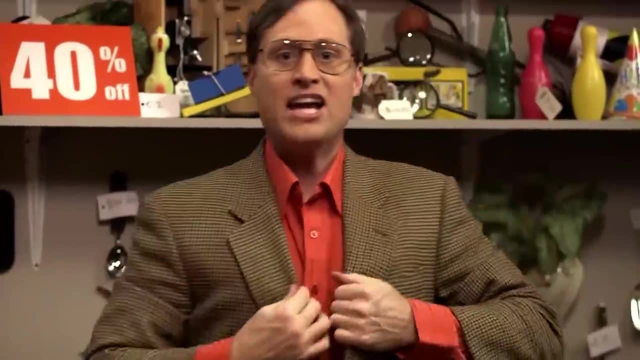 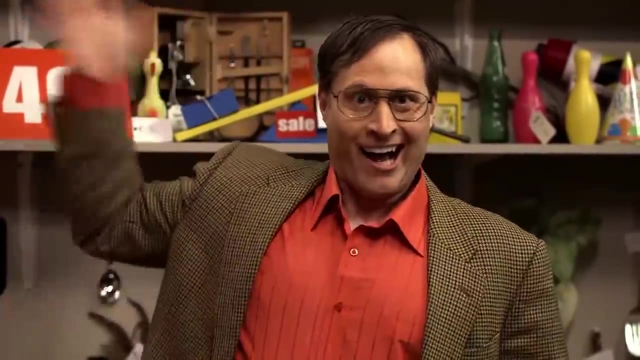 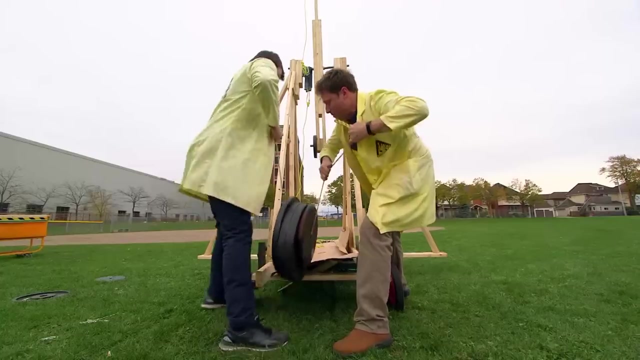 It pivots on that end And you have the load there And there you go: first class, second class and third class levers. Whatever your mood, we've got the levers for you. Chris and I had some trouble getting the weights on our maxed out trebuchet. 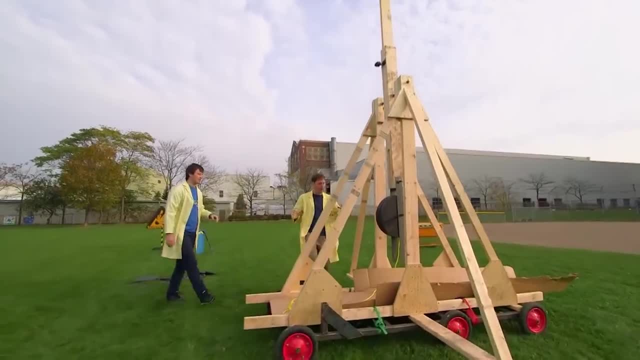 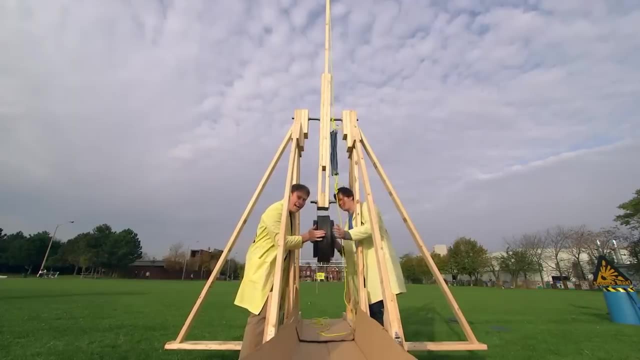 That's going to be a problem, Phil. So we had to come up with a new system: A metal bar that pivots on the bottom of the lever arm. It's got lots of spots for weights And we could lift the weights one at a time to attach them all. 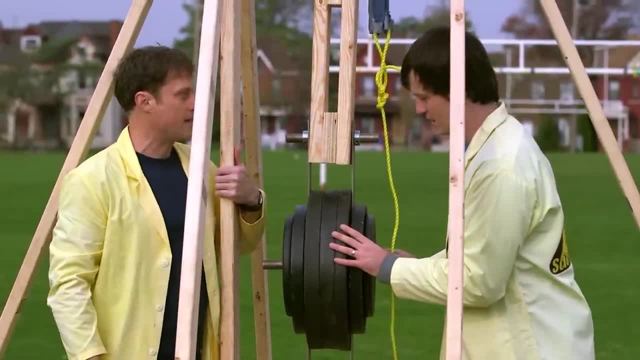 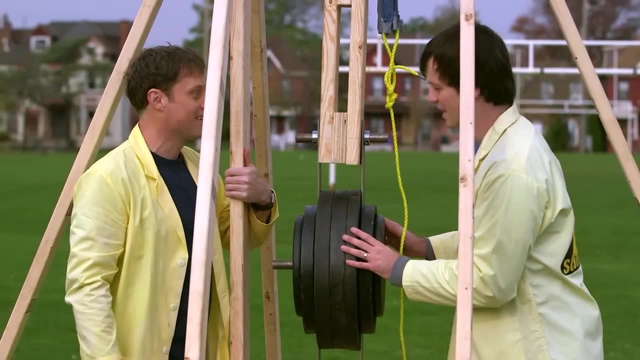 We start out with 255 pounds. How many kilograms is that? 113.3 continues. Yeah, that's what I got too. All right, that's definitely enough. weight right, Definitely. OK, let's fire a pumpkin, Let's do it. 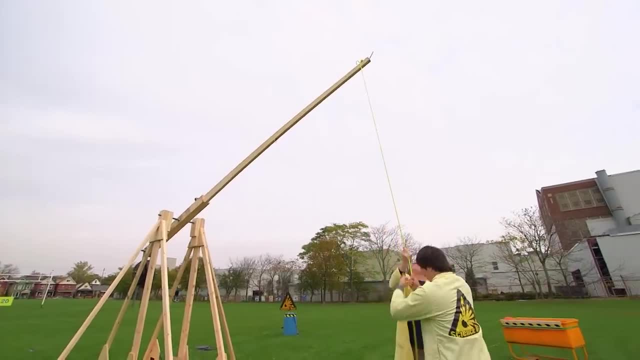 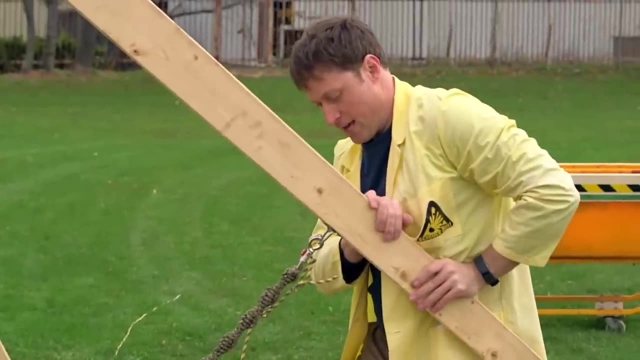 Woo hoo, hoo hoo. This trebuchet works the same as the other models, But because it's so much larger, we really need to haul on the rope. We attach the arm to a quick release which allows us to hold it in place until we're ready to fire. 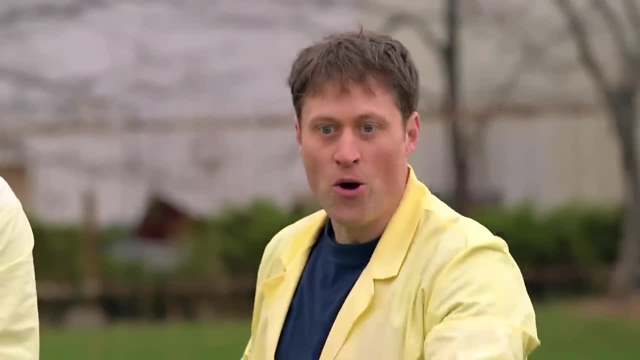 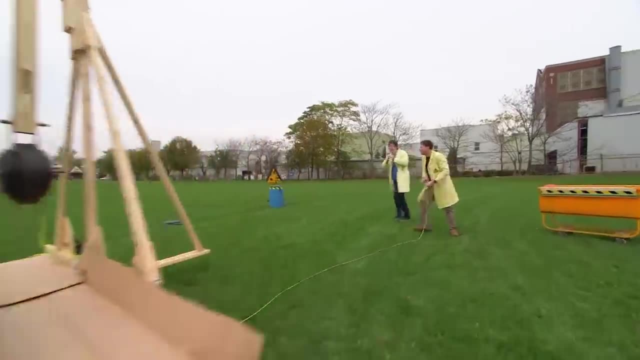 Oh, Here we go. OK, Three, two, one, Three, two one. Whoa, Whoa, Oh, Oh, Oh, Oh, Oh, Oh, Whoa, Whoa, Whoa, Whoa Oh. 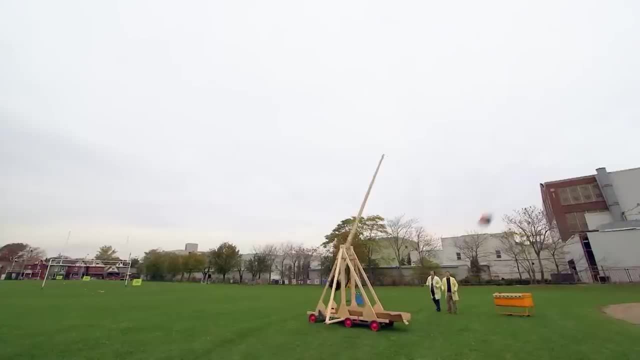 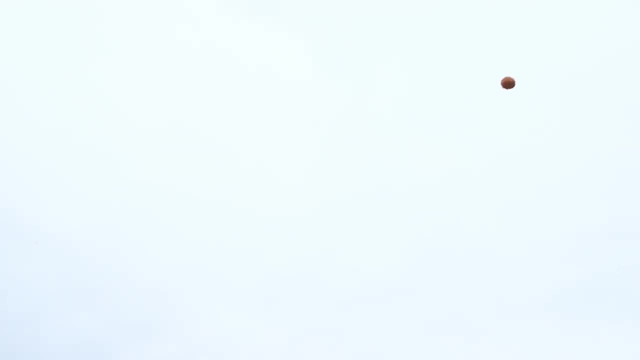 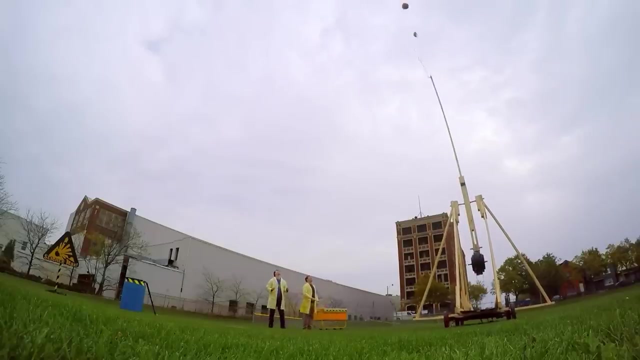 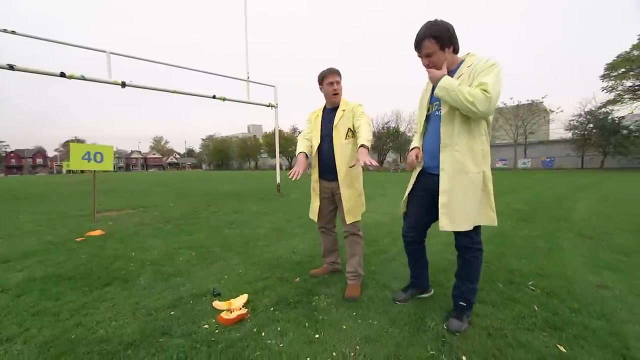 Oh, Oh, Oh, Oh Oh. We launched a bunch of the same-sized pumpkins and got a pretty good idea of the way of how far we were throwing it. Oh OK, you know what? We should leave this here so that we know how far. 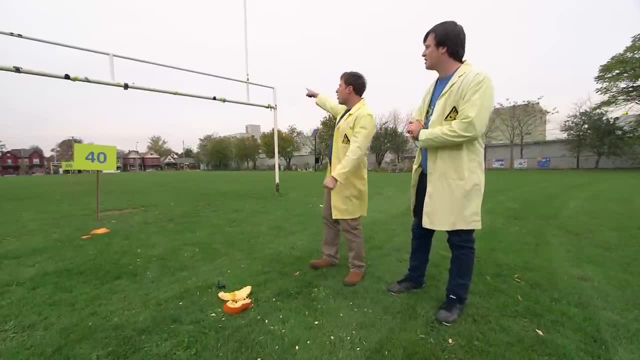 that last pumpkin went And then try to beat it, And then we try to beat it. We haven't gotten through the goalposts. It seemed to handle the more weight pretty well. I think we can add even more. What do you think? 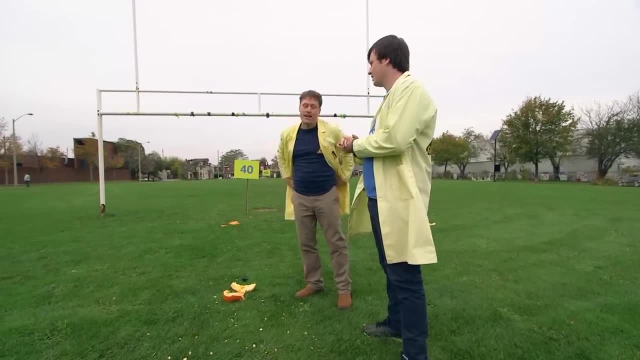 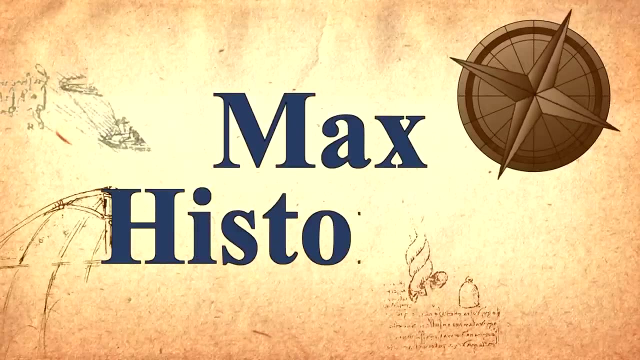 I think we should add all of the weight. This is Science Max. This is not like Science Minimum. Let's max it out. We totally max it out. OK, all the weight, all the weight, all the weight Max Historica. 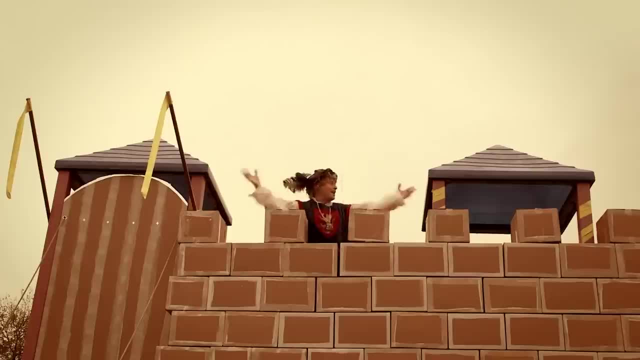 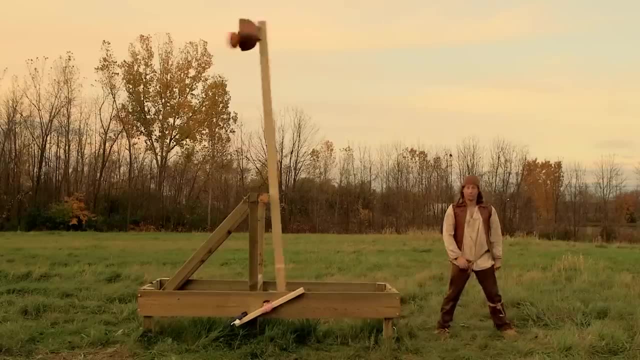 Good morrow to you. I am Lord Fillington the Fourth and welcome to my medieval castle. My father, Lord Fillington the Third, had his castle besieged by catapults And he had to share his prized collection of snow globes. 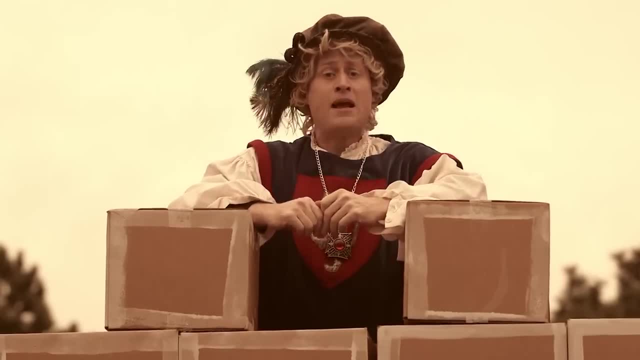 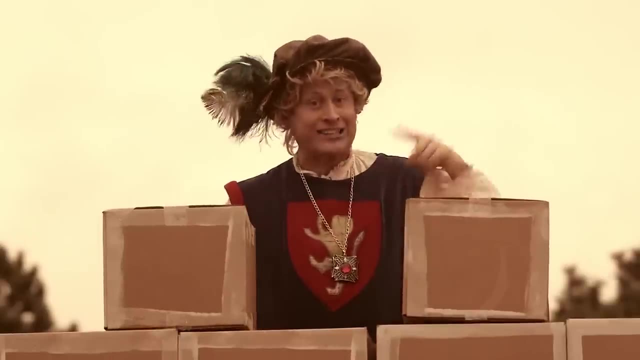 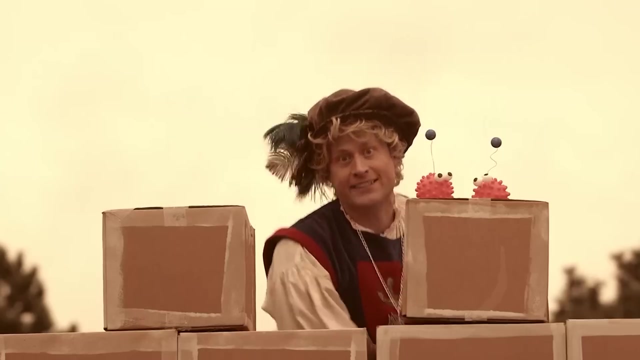 Well, I, Lord Fillington the Fourth, have made a few improvements. First was forgetting about snow globes. It was a so lost season. I collect limited edition Science, Maximals, stuff, toys, And I've collected them all And I'll never share. 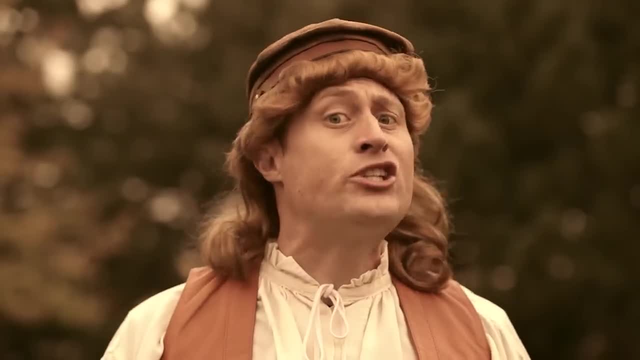 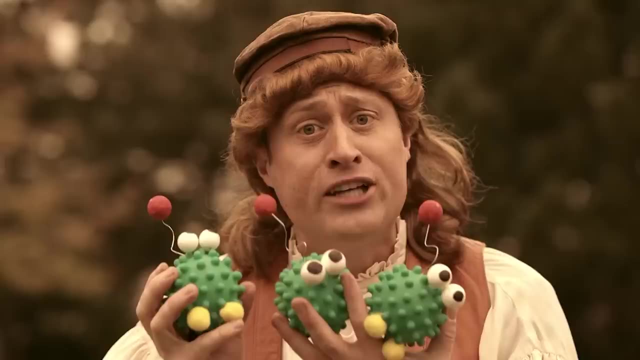 Hello, That Lord Fillington has been hogging all the limited edition Science Maximals and he won't even trade. I mean, look, I've got three floofers and all I need is a fricto, But he won't trade. 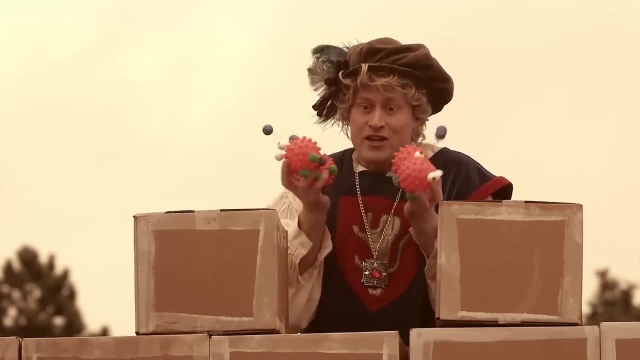 Surely you can trade. Never, Never, Never, Never. I'll have all the frictos and I'll never trade. Ha ha, ha, ha ha. That's it Time to build a-. Oh, you're going to build a catapult. 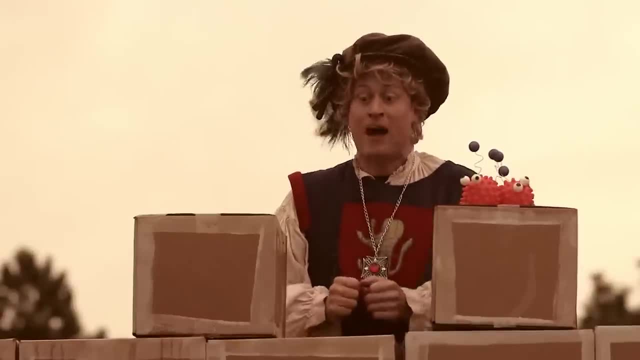 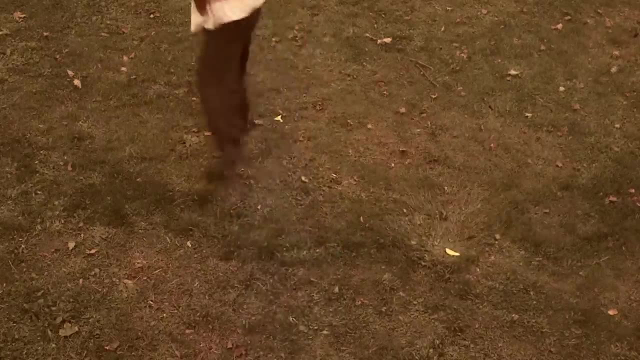 and knock my castle walls down. Well, I've learned a thing or two from my father. I too have catapults Release Ha ha, ha, ha ha. Fortunately, we've got a new invention of our own. 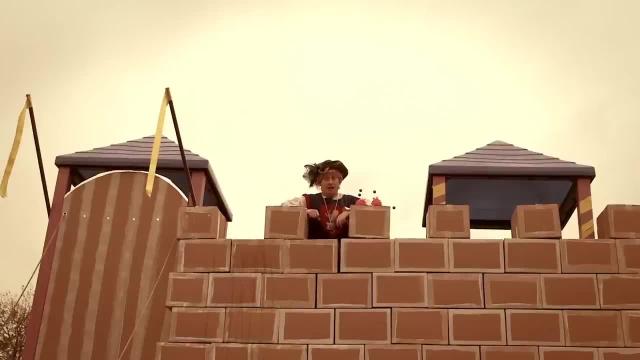 a trebuchet. Oh, fiddlesticks. They have a duck pate Trebuchet A. what A Mother's Day. A Hudson's Bay Trebuchet Cabernet. I can't hear you. You've got to come closer. 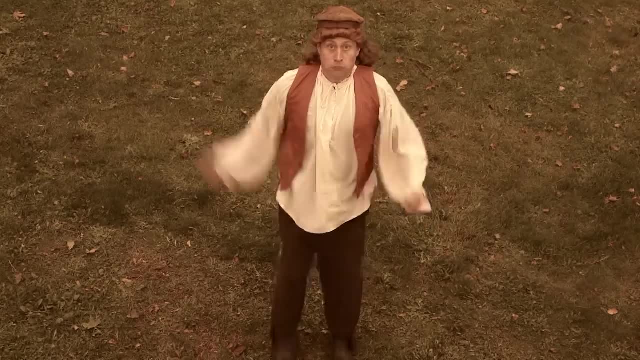 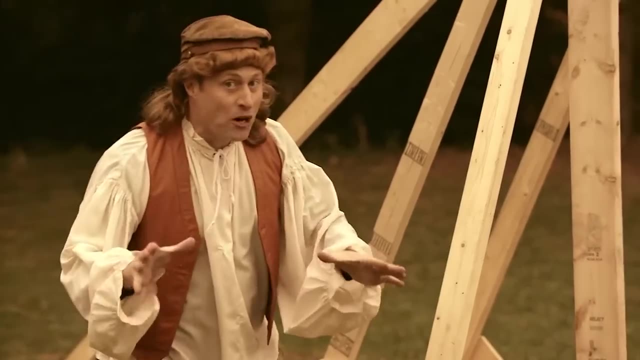 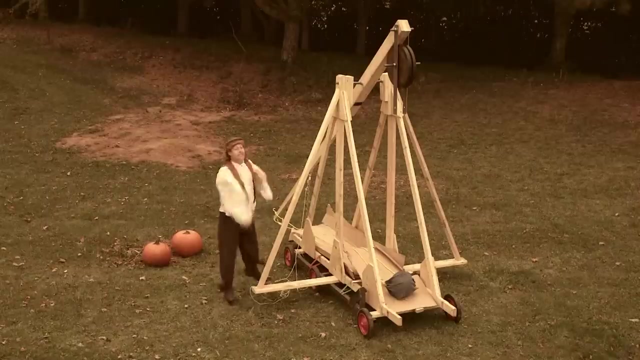 Release: Ha ha, ha ha ha. The trebuchet was the best thing around right up until the invention of gunpowder. It could throw farther than anything else, even catapults. What you do, you see, is you put something in there. 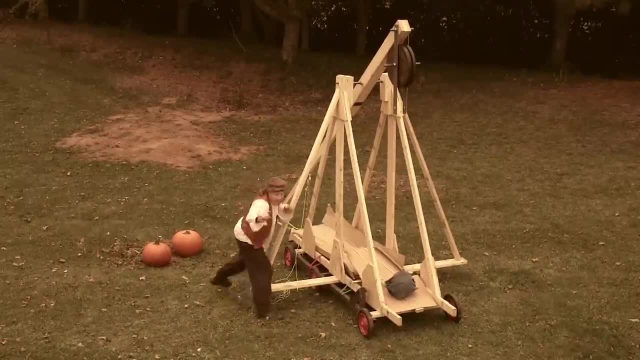 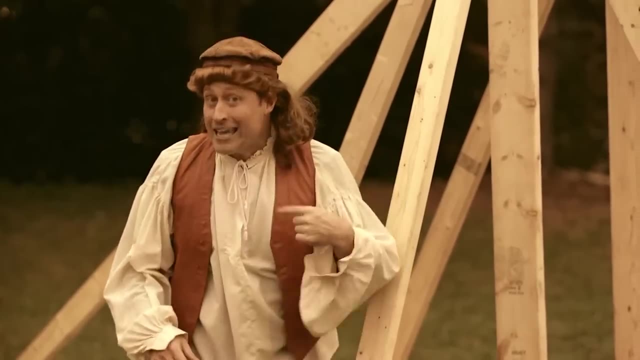 and then you put a big weight up there. all right, This goes down. That flies around and flies over the catapult. It flies over the castle walls, all from far enough away where he can't get me with his catapults, And it works like this. 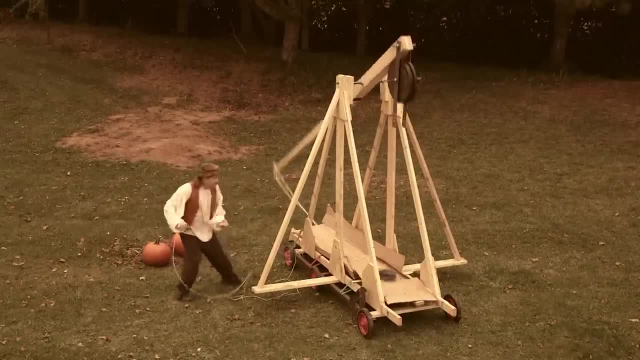 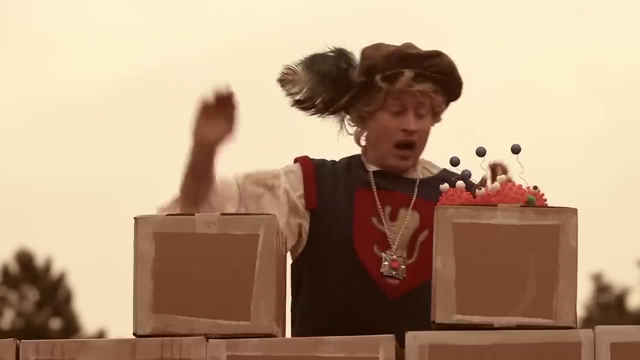 Three, two, one. No, it doesn't make it, It's too high. It's too high. Ah, All right. All right, I give up, I'll trade. Oh, That's quite nice, I like that. 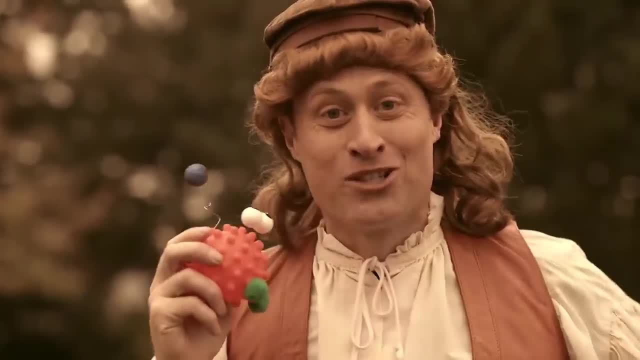 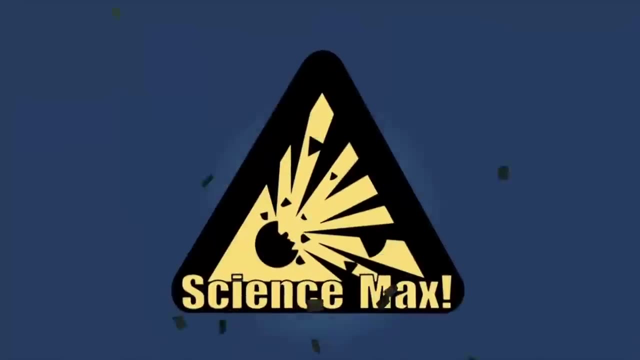 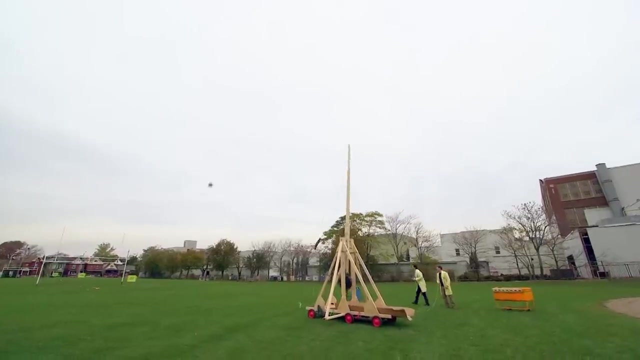 Oh Ha ha, And that's how trebuchets were used in history. Ha ha, Sort of. Our giant trebuchet launched a pumpkin pretty far. Oh Ha ha ha, Very cool, But now it's time to max it out further by adding even more weight. 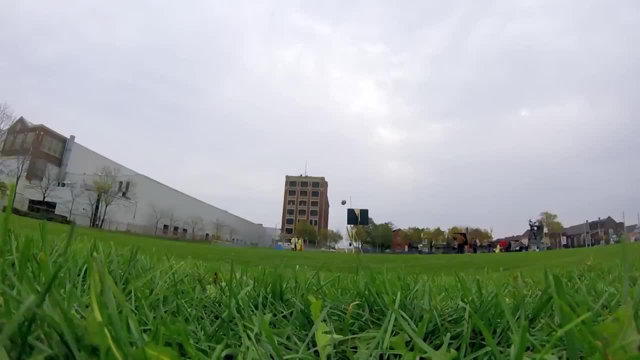 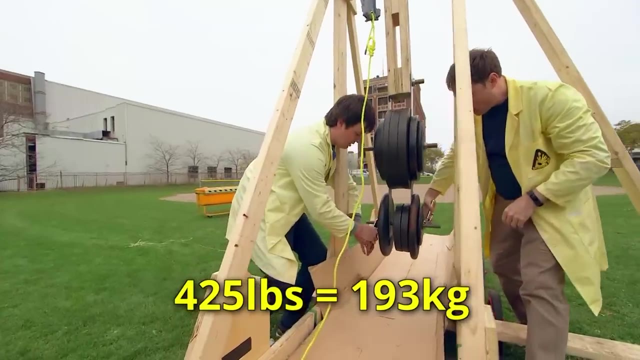 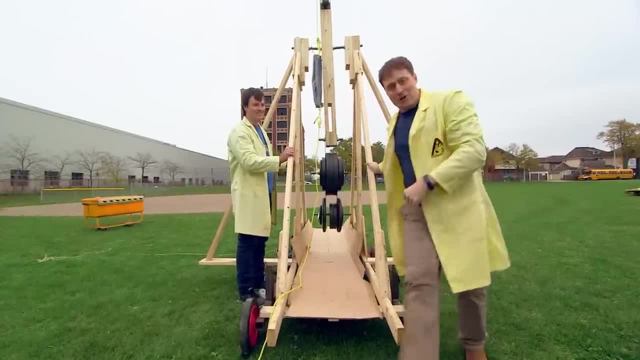 Okay, Are we ready? I think so. I can't wait to see what this thing does. I can't wait to see how heavy it is to pull Turns out. pulling that much weight using our rope was really tough, even with the mechanical. 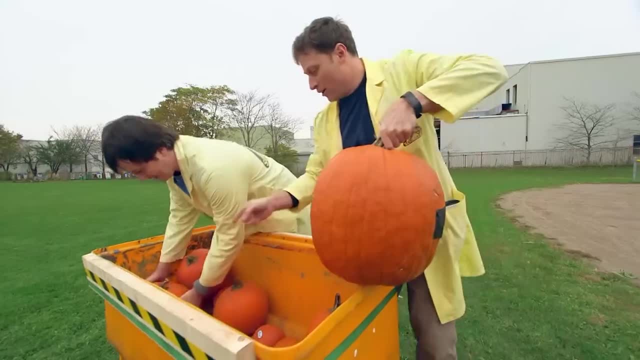 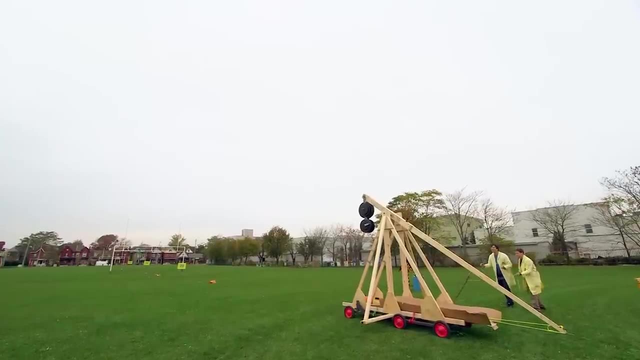 advantage of our lever. There we go. We found another pumpkin of the same size, but then we started having another problem. Three, two, one, Two, one. Let's go. Whoa, Look at how high it is, Whoa. 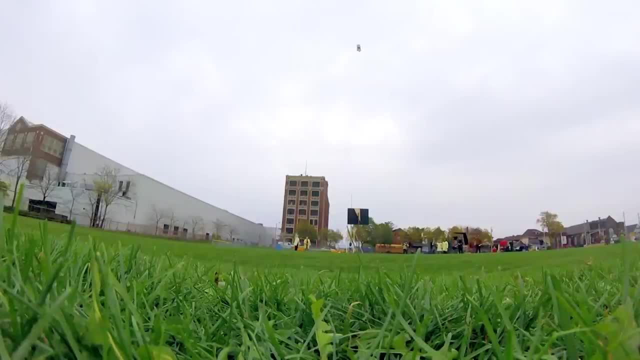 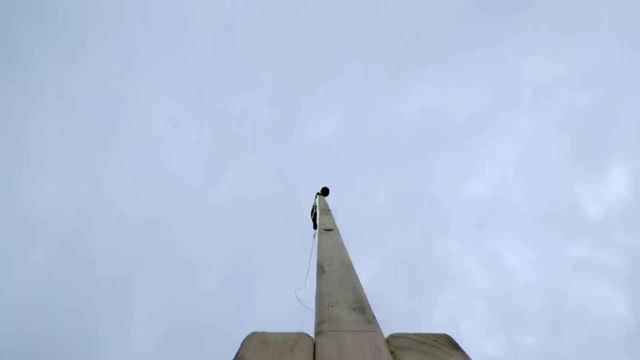 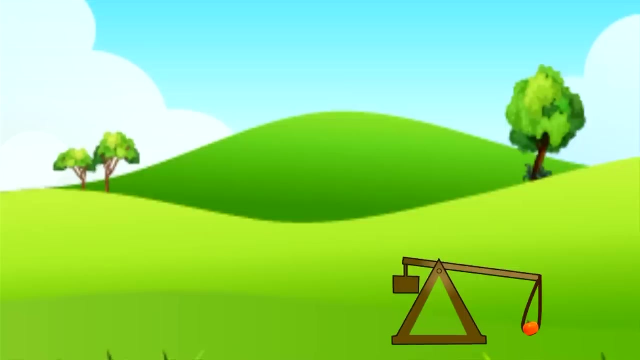 Let's go, Let's go, Whoa, Let's go, Let's go. Whoa, Whoa, Let's go. So I think we're going a little too high. Yes, It was almost straight up How far the pumpkin goes. all comes down to when the rope slips off the pin at the end. 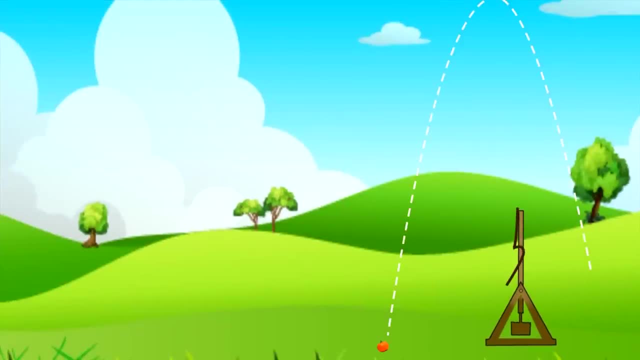 If the rope slips off too early, the pumpkin goes up, and not very far. Too late, and the pumpkin goes straight, which means it'll hit the ground sooner and doesn't go as far. A 45 degree angle is just right, And how do you adjust it? 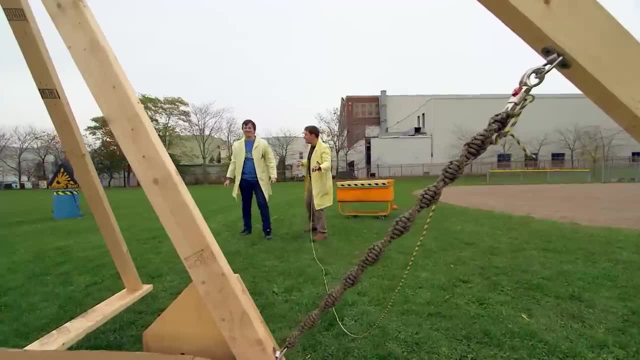 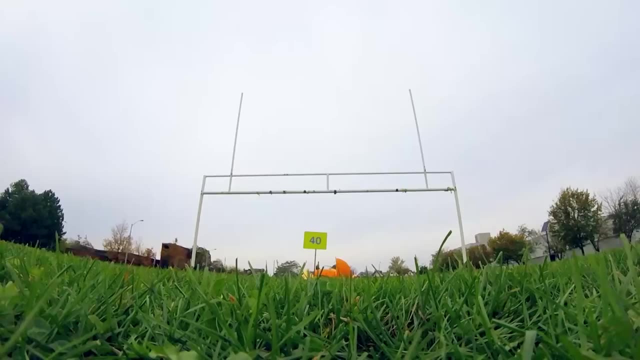 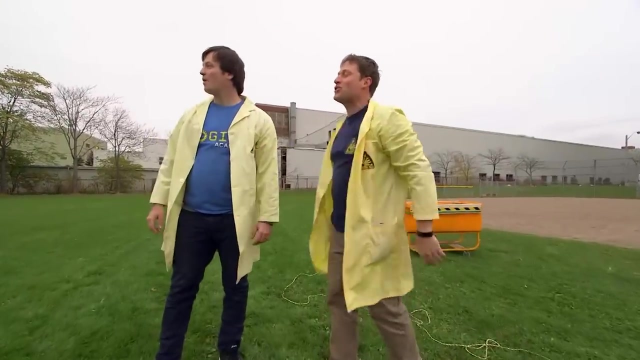 By simply bending the pin. Three, two, one, Whoa, That was great, Whoa, That was great. That went way farther than 60. We should have had another sign. I don't even know how far that went. 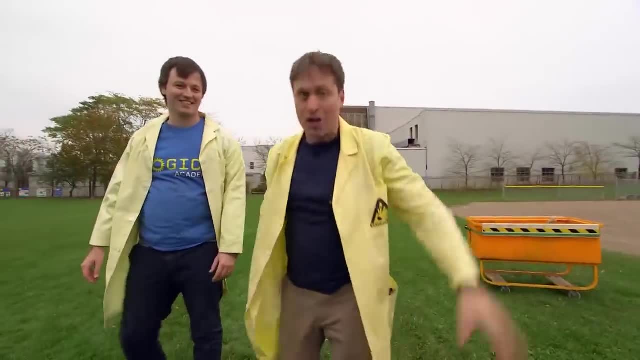 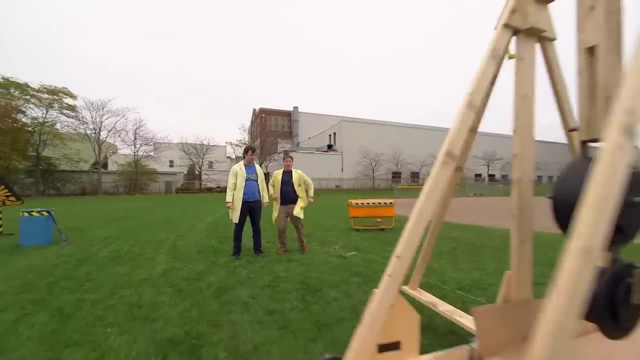 Yeah, There you go. Science max experiments at large trebuchet. So one of us has to clean up the pumpkins and the other one has to put the trebuchet away. Right, Um, pumpkins. What good is science if you can't use it? 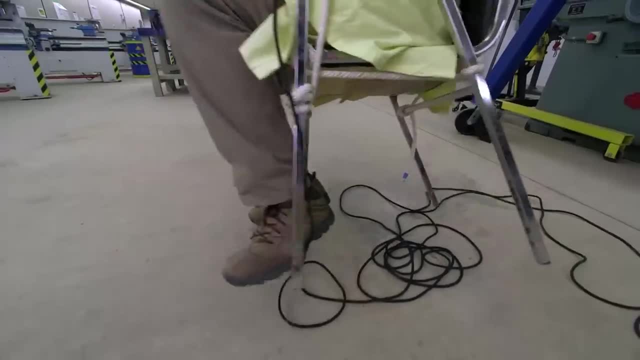 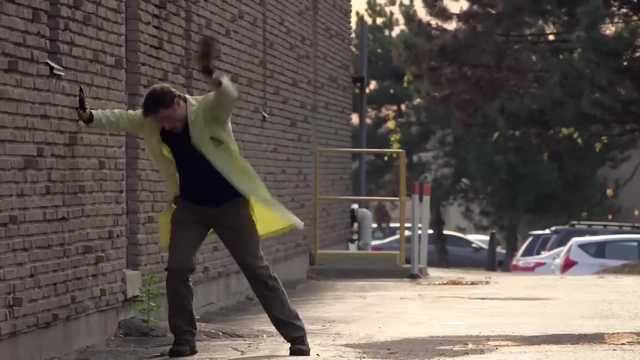 to give you super strength. Well, I tried to do just that on this episode of Science Max: Lifting more, rolling more and a whole lot of running. What, What Simple machines today on Science Max experiments at large. 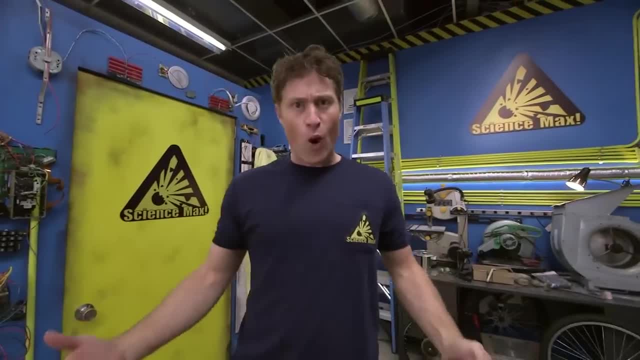 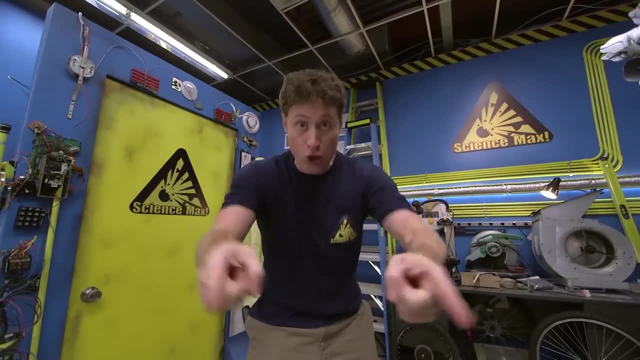 Greetings, science Maximites. I have a question for you. Have you ever wanted super powers like super strength? Well, today, on Science Max experiments at large, I'm gonna give you and myself super strength using the power of science. 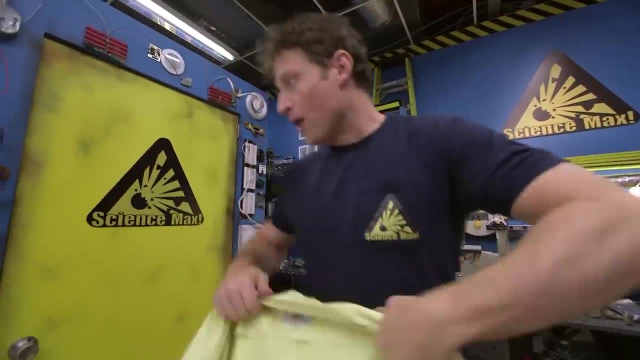 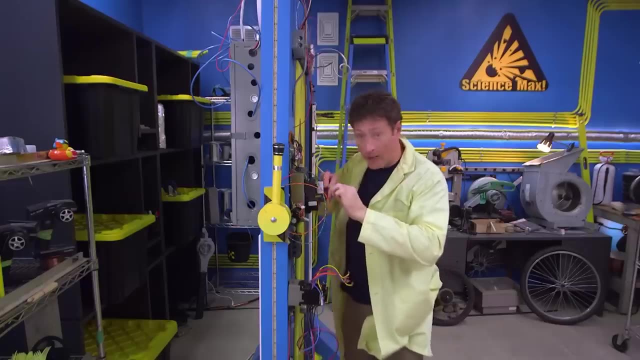 But we're gonna do things a little differently today, You see. well, the portal hasn't been working perfectly since, well, since I built it. But I ordered a new particle impulse controller and all I have to do is get it back to the lab. 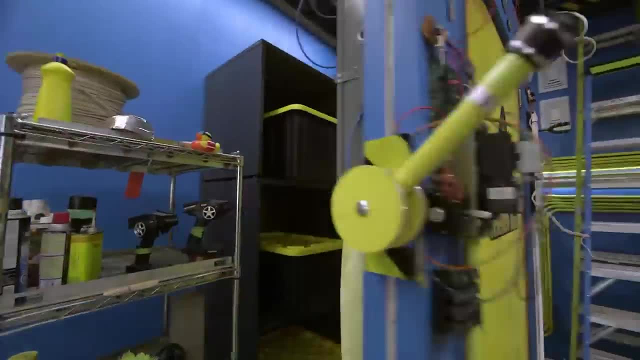 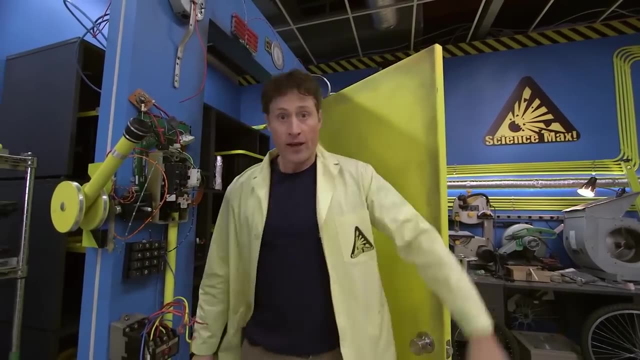 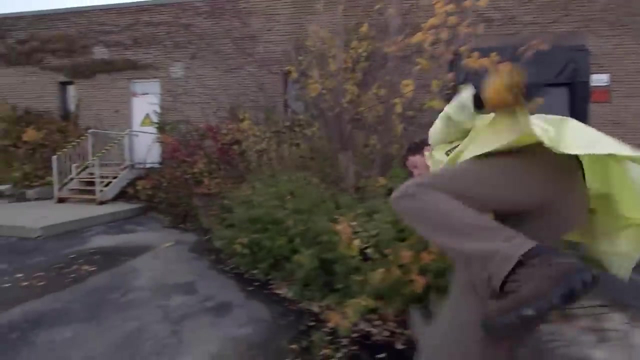 Perfect timing. It looks like the portal, the portal is broken, Um, okay, well, no problem. Okay, okay, I'm here, I'm here. Wow, That's perfect. One particle impulse controller for you. All right, thanks very much. 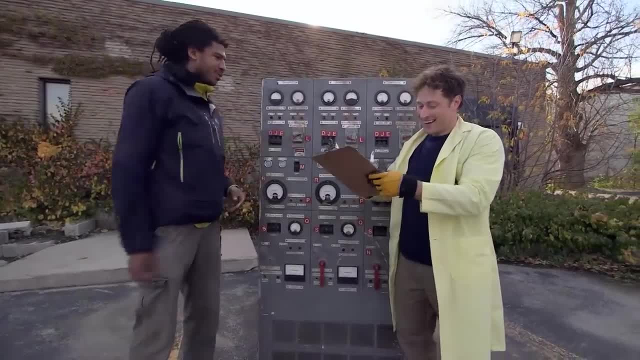 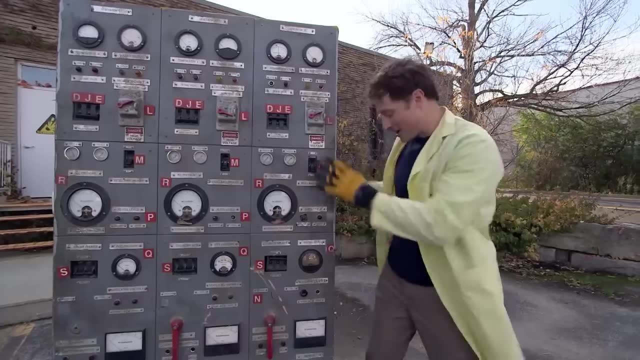 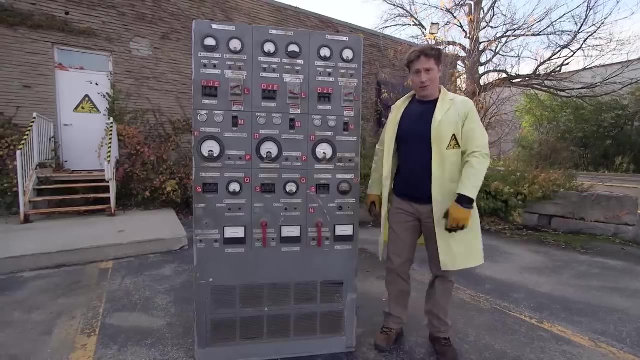 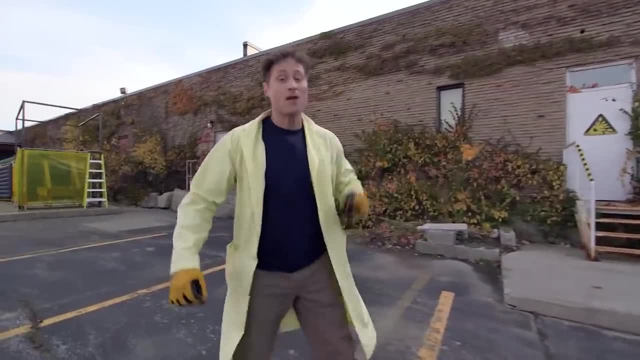 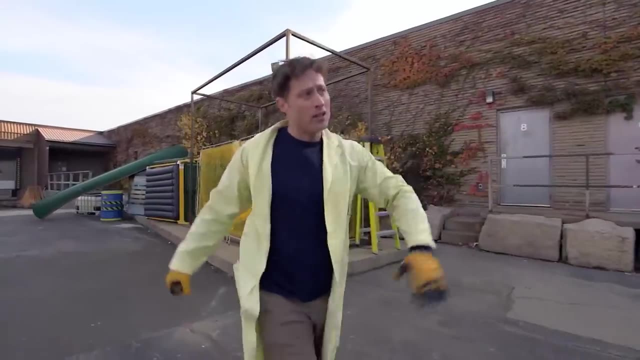 this episode of Science, Max Experiments at Large, is gonna be a little different, because today I'm not gonna have an expert come and help me, because I'm gonna move that giant heavy particle impulse controller all the way across the parking lot and all the way up that loading ramp. 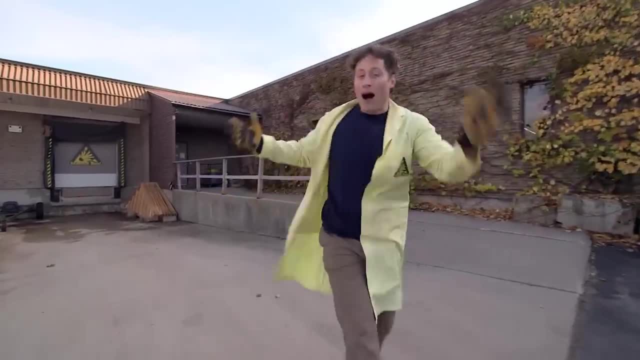 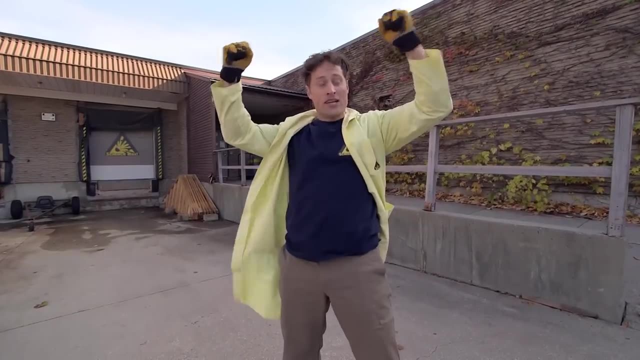 by myself, With nobody's help. How am I gonna move a giant heavy machine all that way if I can barely even budget? Well, I'm gonna give myself super powers, super strength, with the power of simple machines, And the first machine we're gonna start with is the lever. 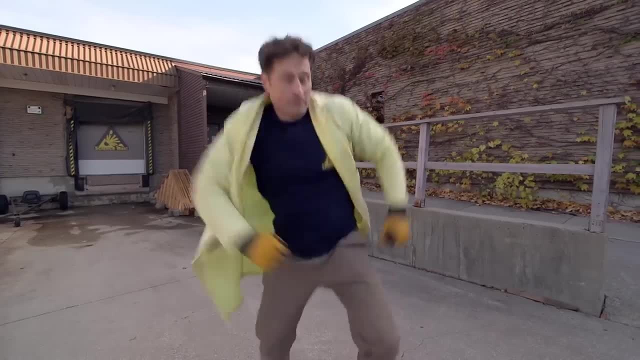 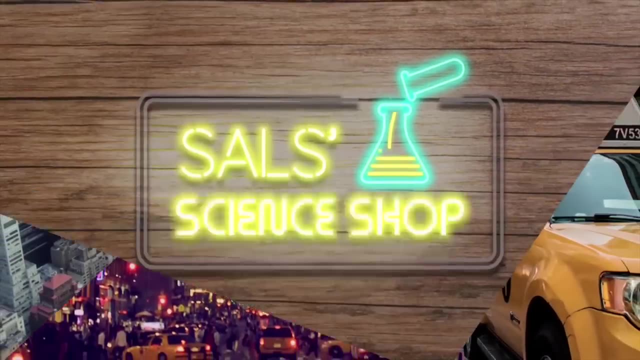 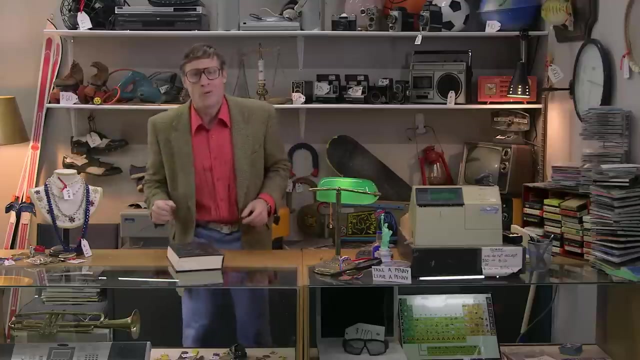 which I guess I should go back to the lab to tell you about. All right, Sal, I'll see you next time, All right? Oh, hey, how you doing. Let me guess You got some work to do when you need it done, easy, right. 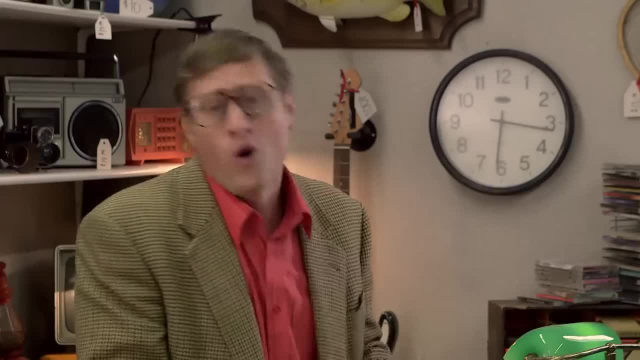 I mean, look at this book. I mean you could pick it up. but what Are you gonna be some sort of book-picker-upper person now? Is that all you're gonna do? Is that gonna be your life, just picking up books left, right and center? 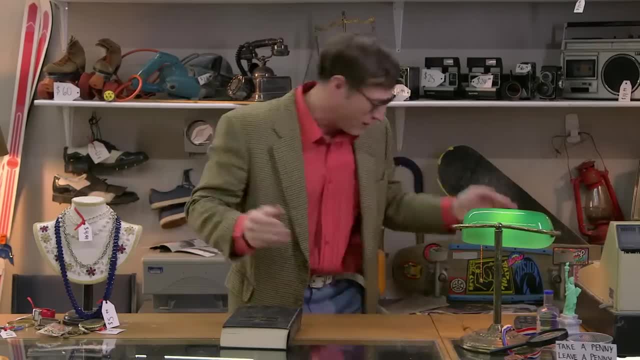 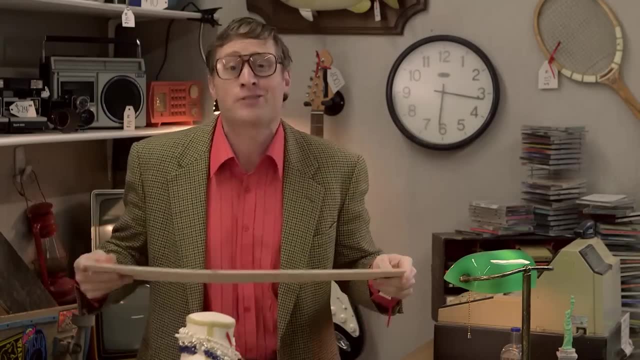 No, you're smarter than that. You know what you need: A lever Like this. Now, I know what you're thinking. I know you're thinking: hey, this is just a plank. You're right, That's because you're smart. 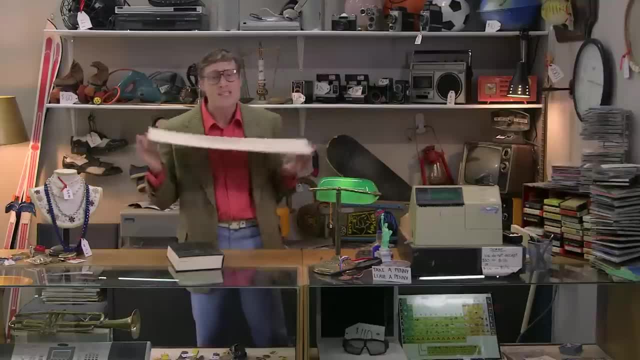 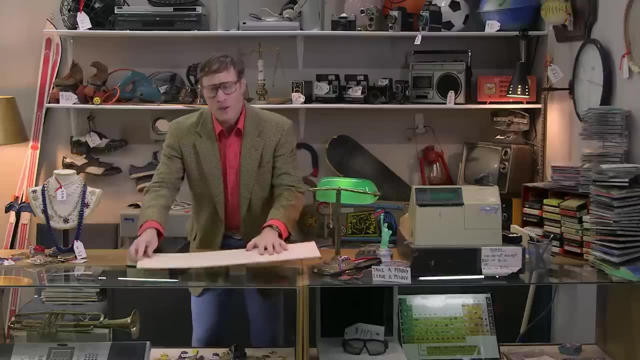 A plank can be a lever. All you need is two sides and a place for it to pivot- A fulcrum. It can be anything. Look at this Bam. Now it's pivoting. I put the book on this side and then I push down on that side. 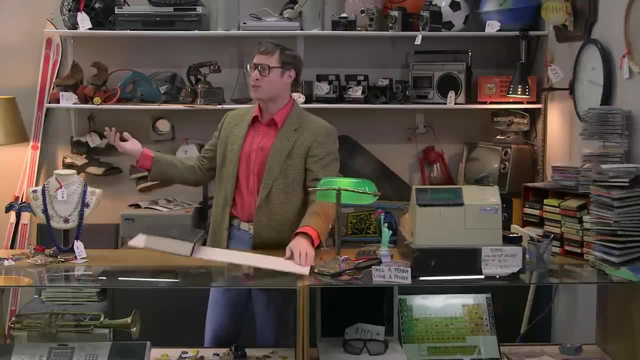 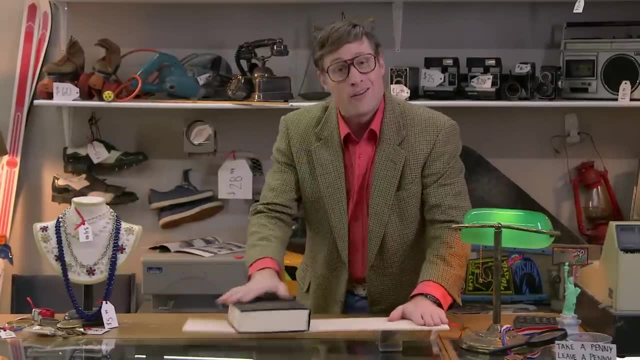 I'm doing work easy. Hey, look at me doing this work over here. If I want to do more work, I could move the fulcrum a little bit further over. Now. I do lots of work, but I lift the book a lot further. 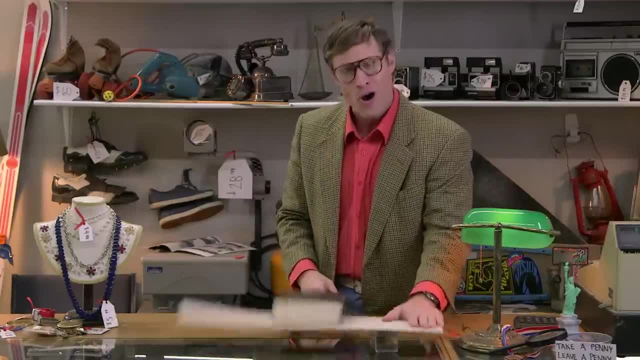 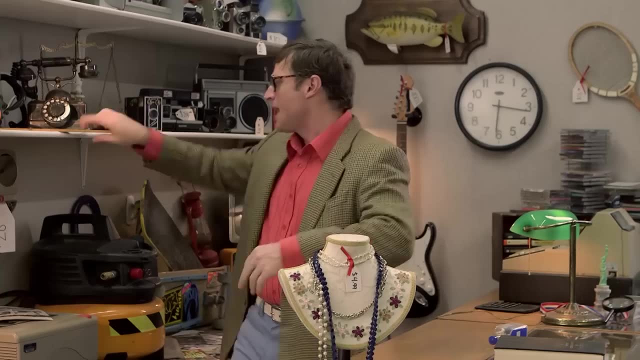 Look at that: Whoa, What, Whoa, Yeah, Huh. What do you say? What do you say? Huh, Huh. You don't like this lever, Don't worry, Hold on, I got another one for you here. 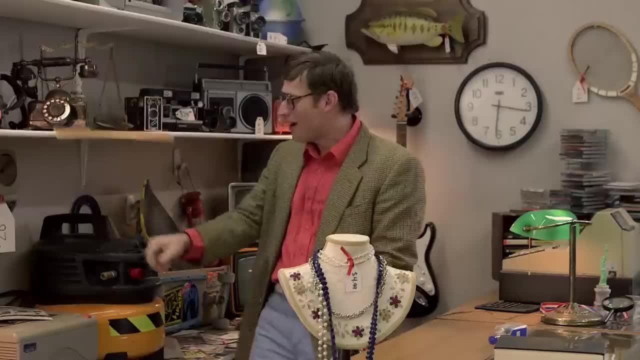 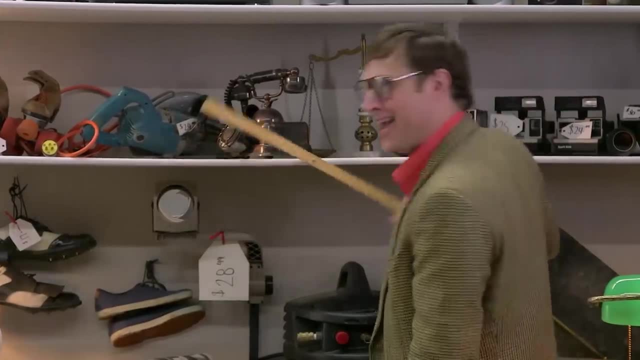 Hey, take this stick. All you need is two ends and a place for it to pivot Like this Bam. Now it's a lever. This side goes down, That side goes up, Down, Up. It's a lever, It's a lever. 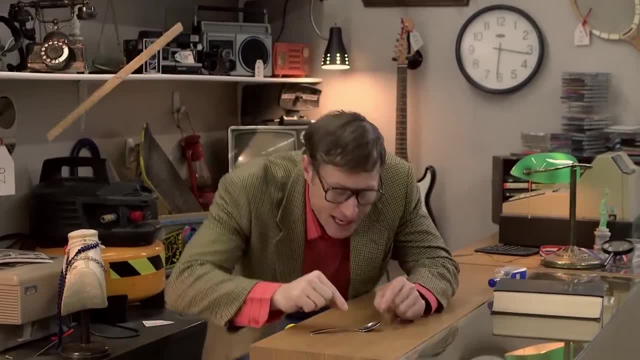 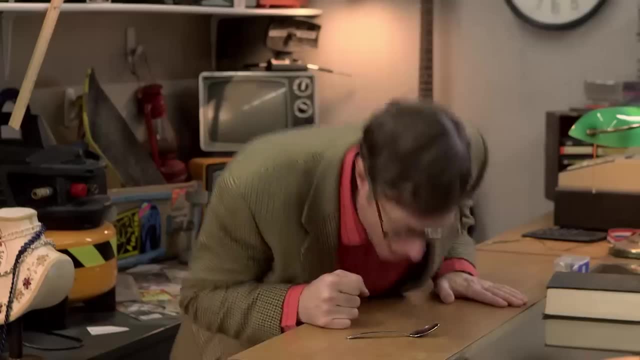 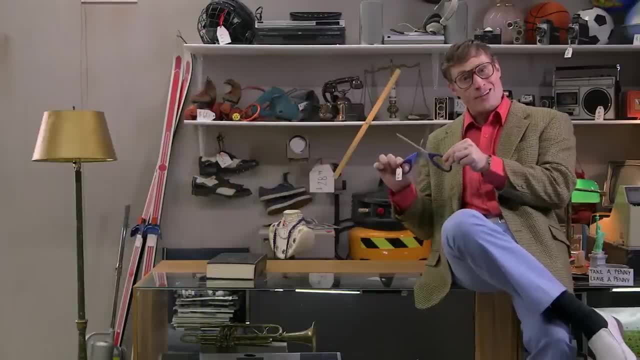 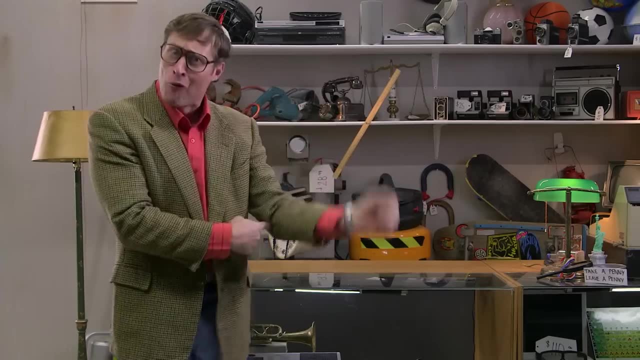 Now it's a lever Scissors, Two levers, Your forearm. It's a lever, Two ends And the fulcrum where it pivots. Yeah, the fulcrum can be at one end. Crazy, This fish. 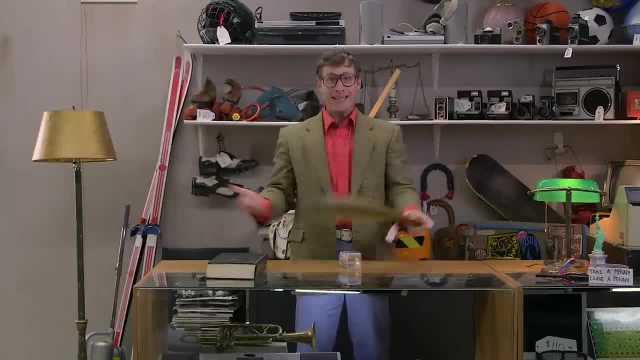 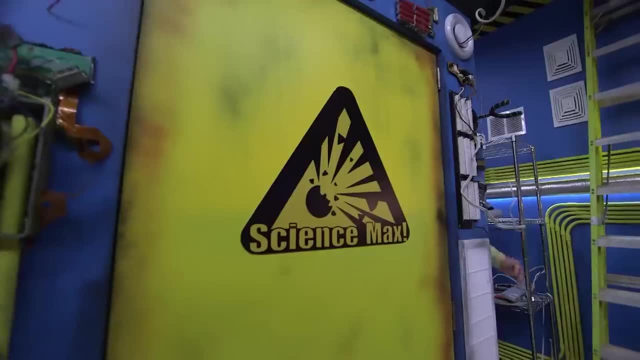 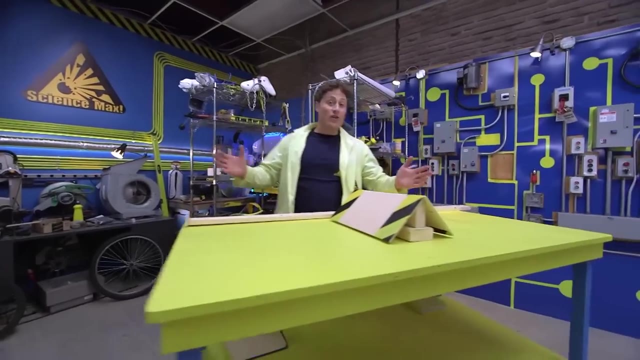 You guessed it. Now it's a lever, And now you know your levers. Okay, Where were we? Oh, yeah, levers. So you can use levers to become much stronger Or at least lift something you couldn't normally lift. 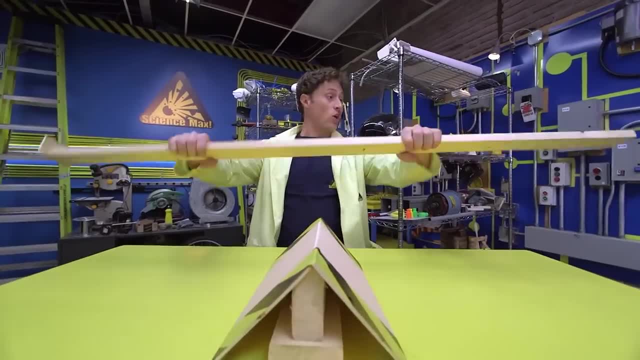 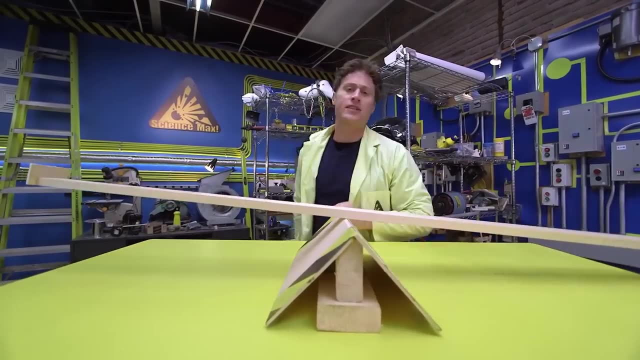 Levers are simple machines and they work like this. Levers are just a long rod or stick or pole or piece of wood like I've got here, And something for them to pivot on A fulcrum. Now let's say you have something heavy like this book. 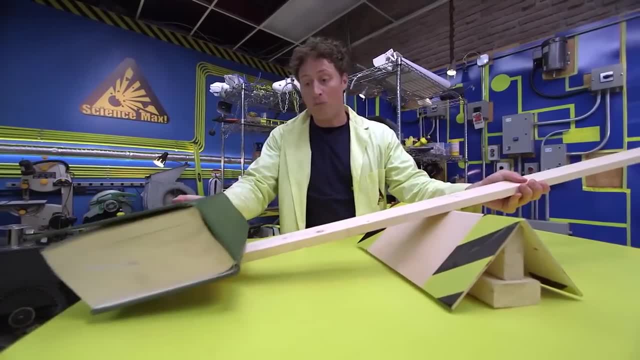 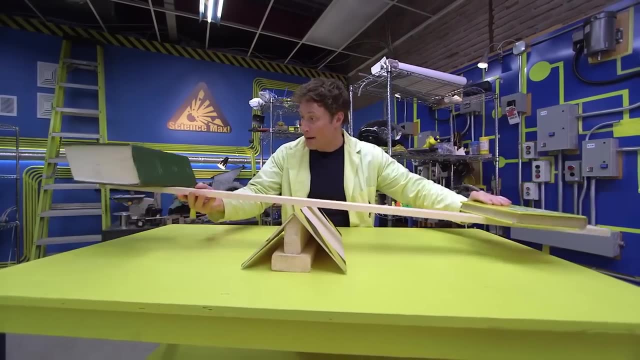 Sure, I can lift it. But what if I told you I can lift this heavy book with this book? Now, if the fulcrum is in the middle, like a seesaw, you can tell that book is much heavier than the other book. 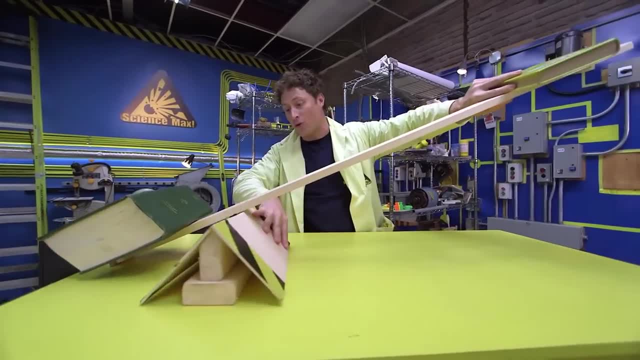 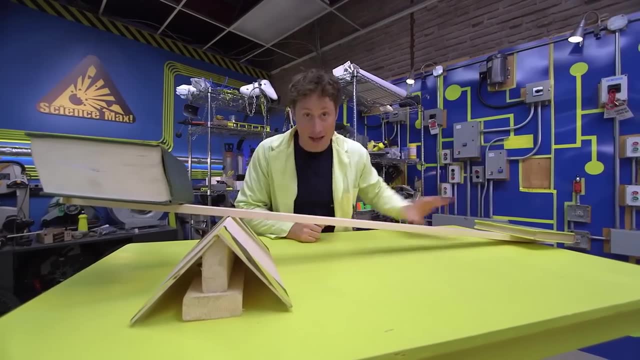 But watch what happens when I move the fulcrum: Mm-hmm, Mm-hmm, Huh, It's like magic, But it's not magic, It's science. Whoa, It's because the small weight is moving a long distance. 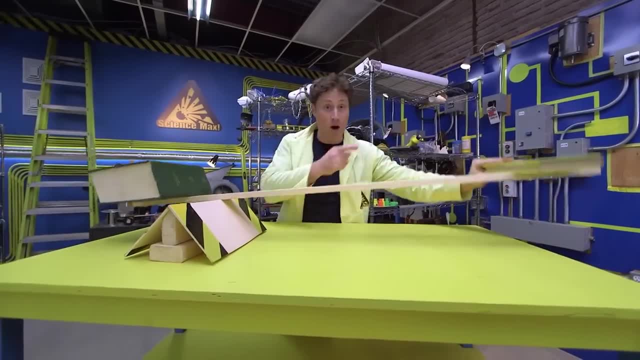 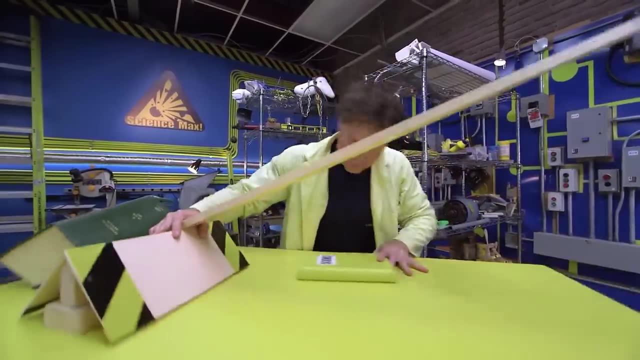 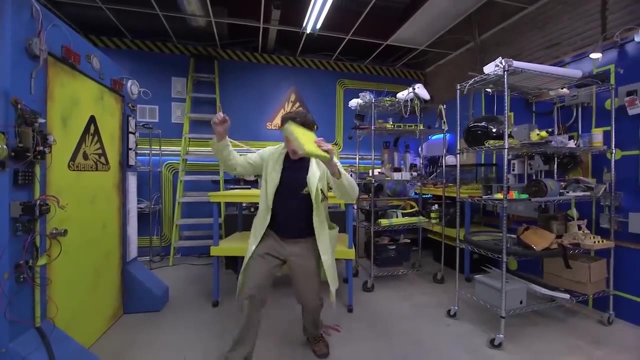 and the heavy weight is moving a long distance And the heavy weight is moving a short distance: Small weight, long distance, Heavy weight- short distance. So everything balances out. But here's where it gets interesting: The longer your lever, the more weight you can lift. 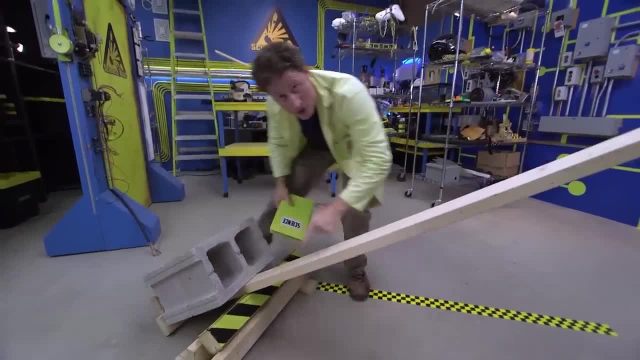 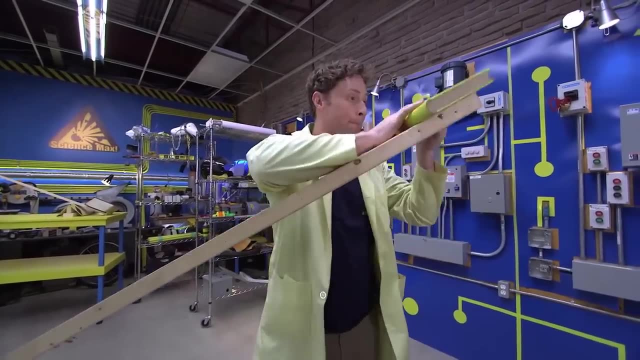 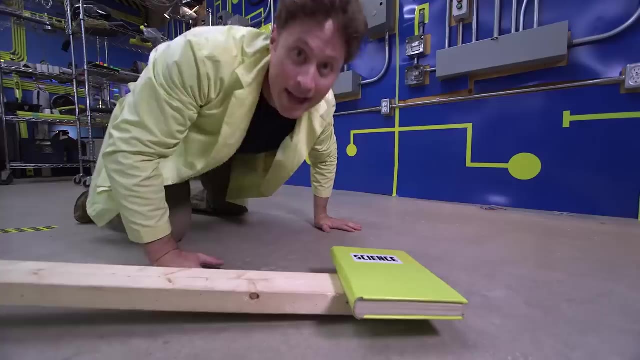 These are two heavy cinder blocks. There's the fulcrum and here is a very long lever with which I am going to lift those cinder blocks with this book. Ha-ha. And there you have it, Levers. Now back to the particle impulse controller. 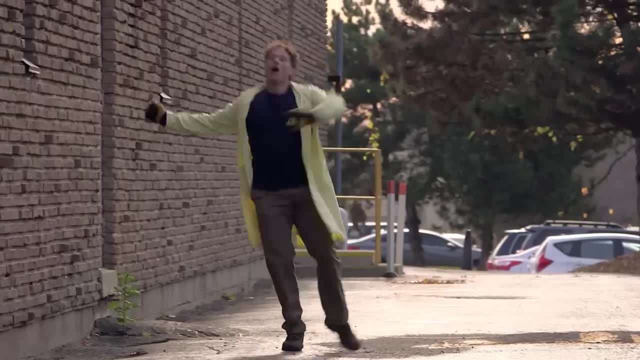 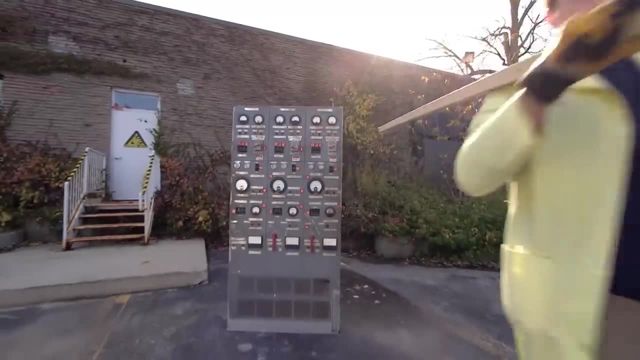 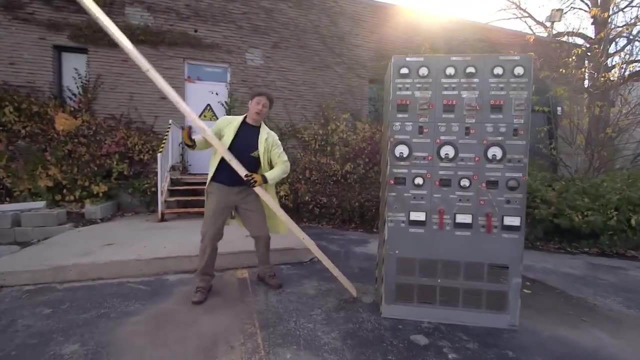 Oh right, Uh-oh, What, What? Oh? Oh, Ha-ha-ha-ha-ha Lever. Here we go. I got my giant lever. The bigger the lever is, the easier it is to do the work. 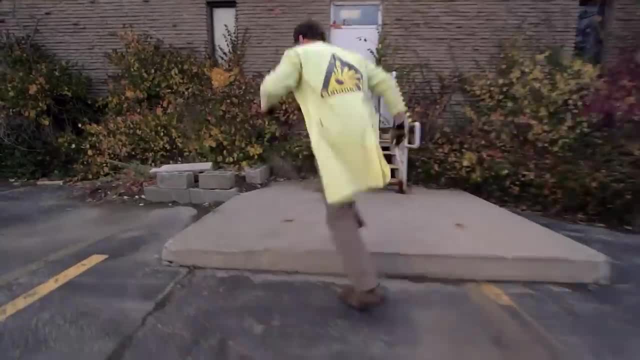 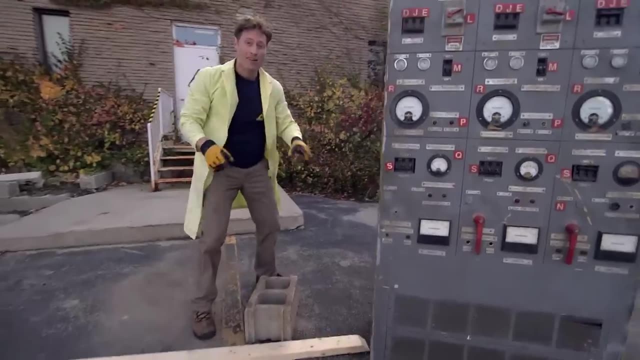 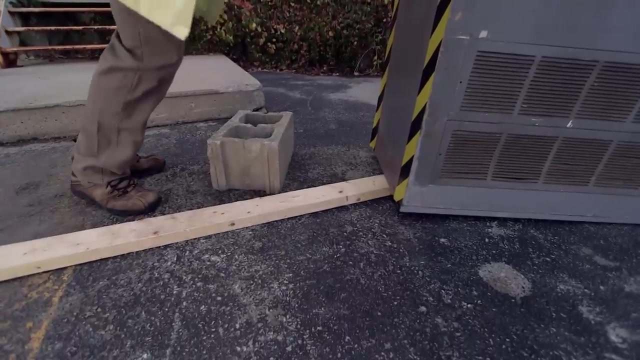 Uh, I need a fulcrum. Uh, ah, Just about anything will do for a fulcrum And put that there Now. the hardest part is getting it on the lever. Okay, Okay, Okay, Okay, All right. 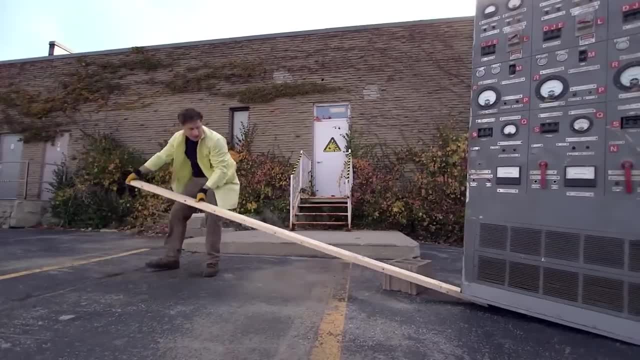 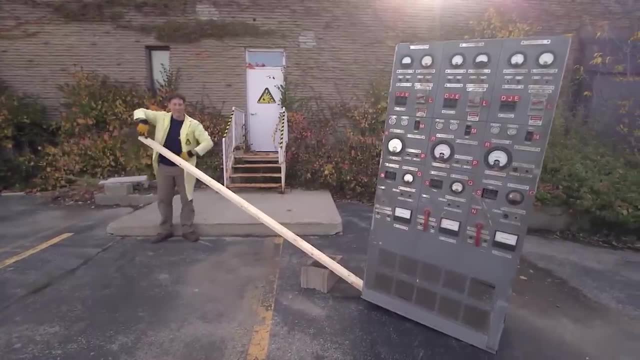 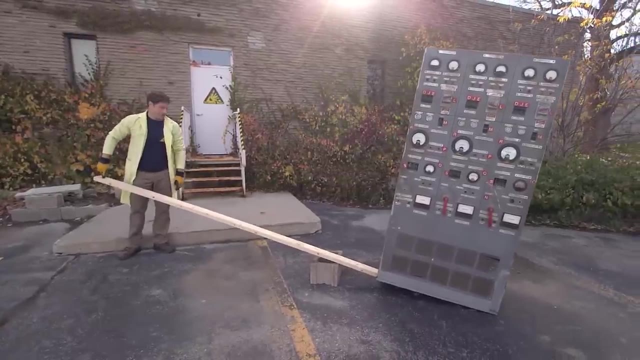 Hardest part is over. Get the lever up on the fulcrum And Oh-ho-ho-ho, Look at this. No problem, One finger lifting. It suddenly became very easy for me to move this. I guess I need to do more than just lift it, though, huh. 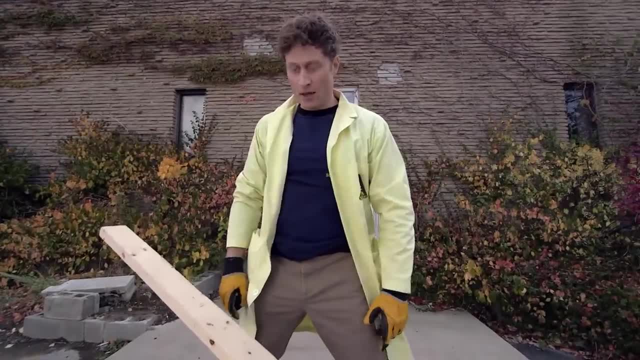 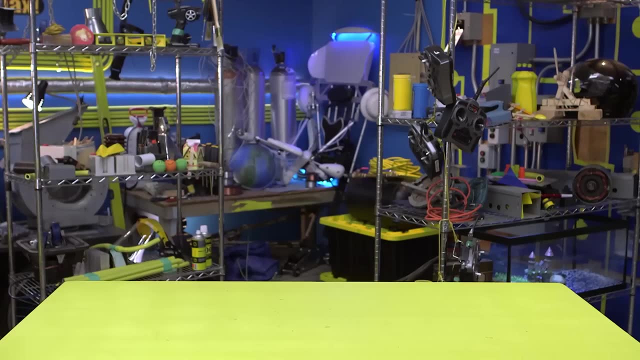 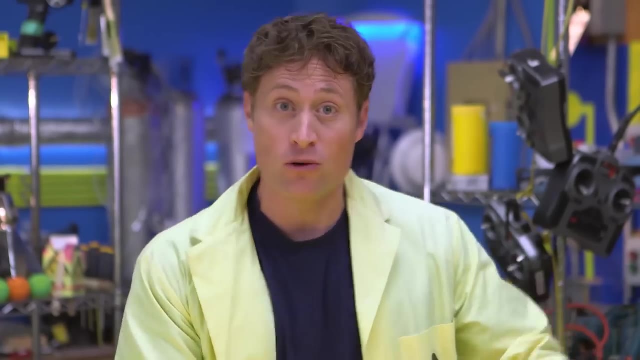 Because I have to move it all the way. uh, Oh, rollers. Come on Back to the lab. Okay, Rollers. Rollers are like wheels, except they're not attached to anything. In ancient times, they used to move giant, heavy blocks of stone using rollers. 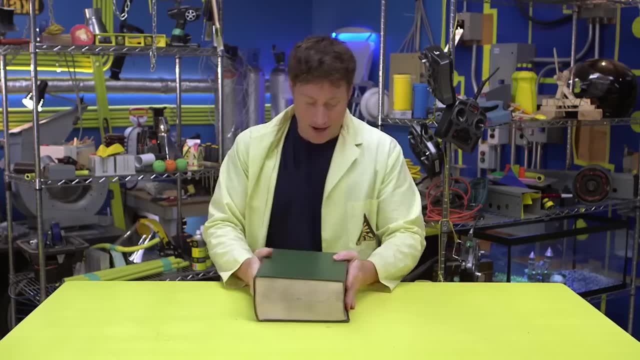 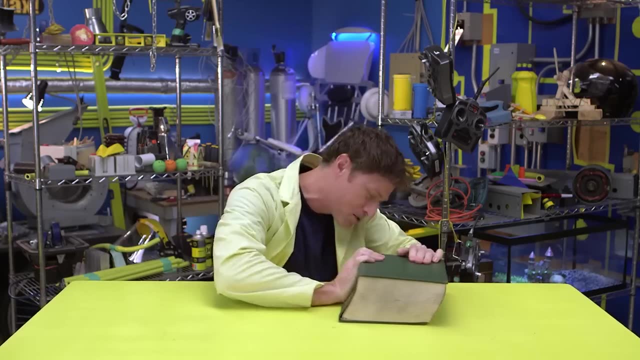 We can do this. We can demonstrate using a book. Now get a book, put it on a table and try to move it across the table. You'll see that it's very difficult. I can't move this book across the table. 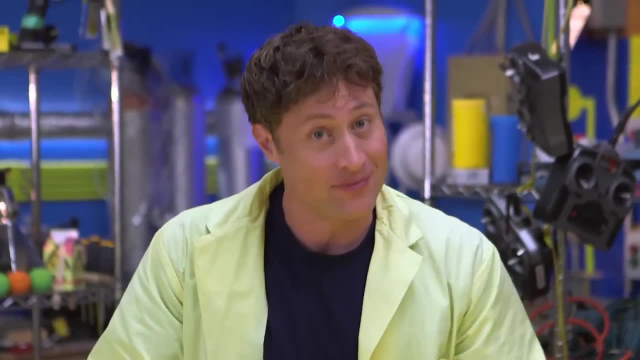 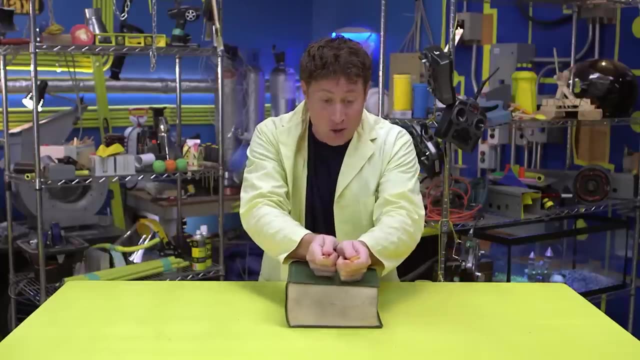 I can't. Okay, it's not really that hard, But still it takes effort. But if we get some rollers, I like to use pencil crayons and not pencils. and here's why: Take a closer look, You see, pencils aren't round. 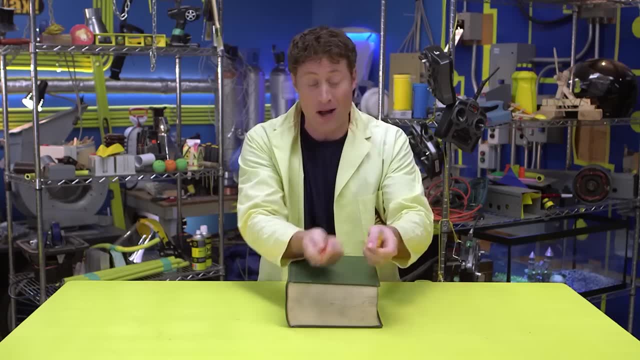 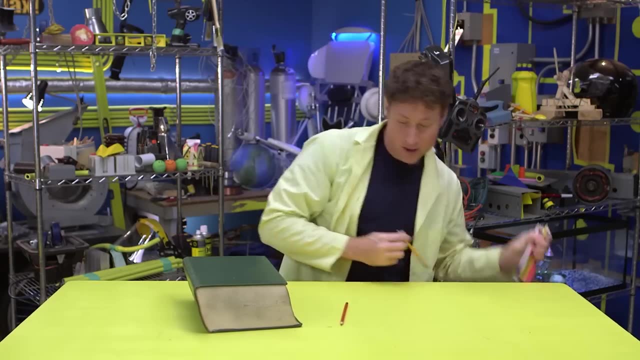 They're hexagonal, They have six sides, whereas pencil crayons are round And, of course, if you want something to roll, you can roll it. You want something round, So get a bunch of pencil crayons and put them on the table. 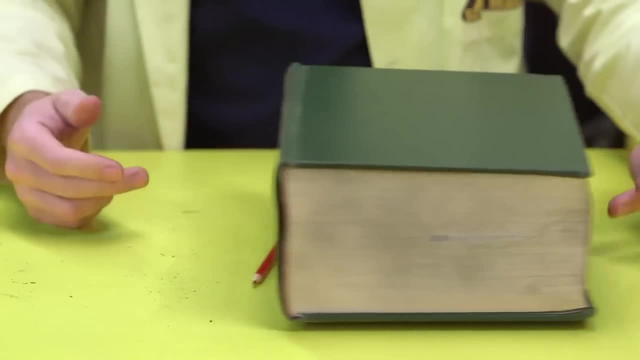 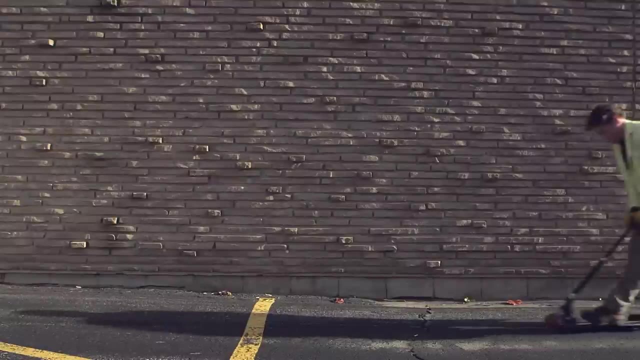 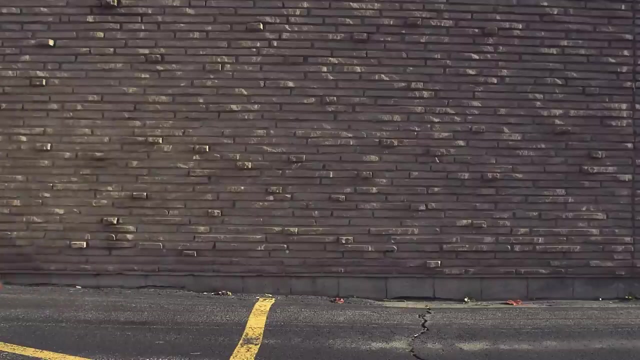 And put the book on the pencil crayons And you'll see that suddenly moving it is a lot easier. All right, That's rollers Back, I go. Now it's time for Science. So Simple A Caveman Could Do It. This is a caveman. 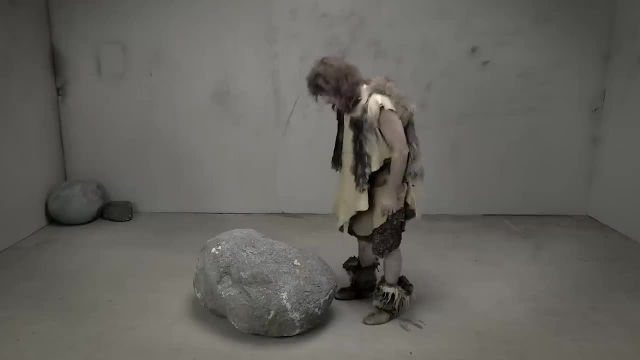 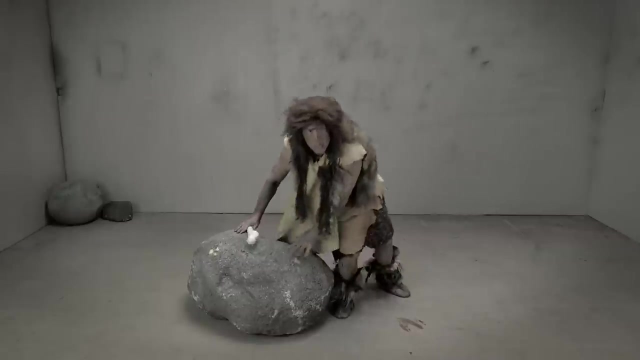 Huh, This is a rock Knock. It is a well-known scientific fact that if this caveman were to try to move that rock, he would not know how to do it easily. Poor caveman. But in ancient times people learned how to move heavy rocks. 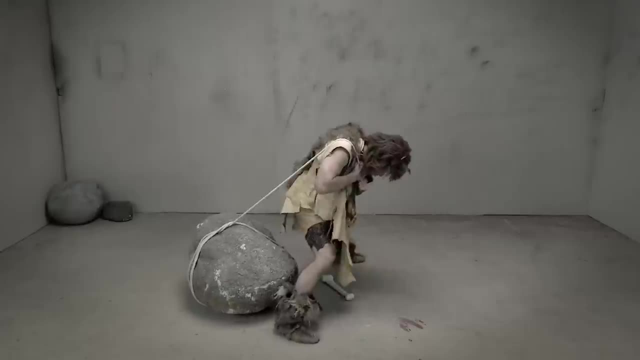 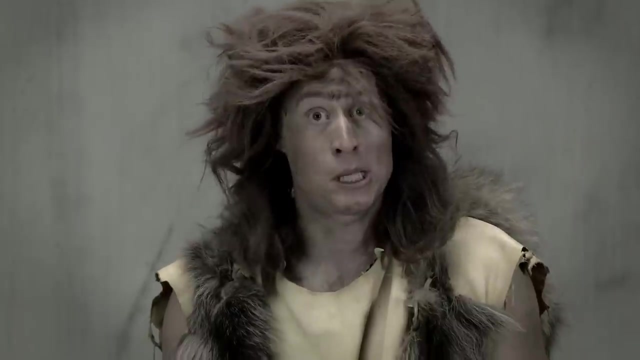 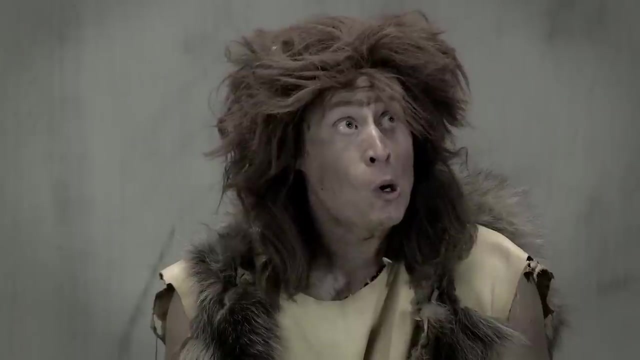 using ropes, and ropes, Uh-oh, Oh, no. And rollers, Oh, Rollers, Yes, rollers, Rol-ers, R-rollers, Rol-ers, Close enough. Rollers make it much easier to move a heavy object. 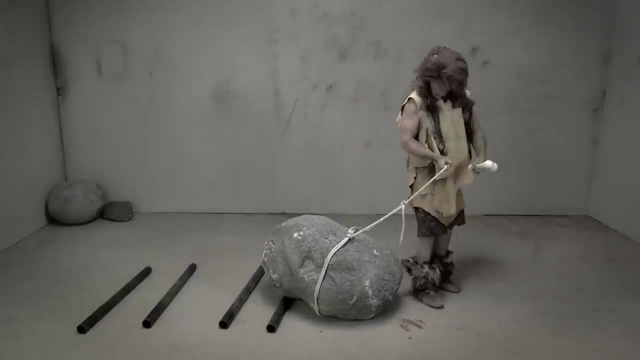 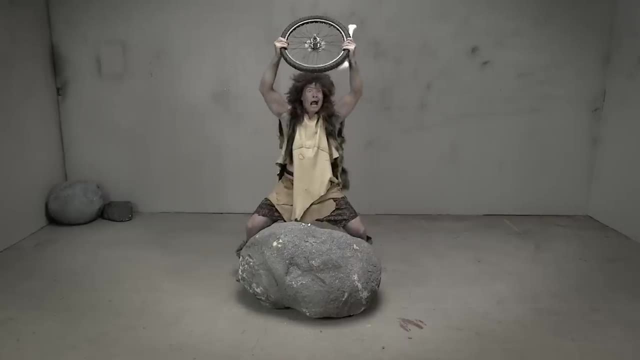 Oh, hahah, But they aren't perfect. So the wheel was invented. Yeah, The wheel is a simple machine and one of mankind's greatest invention. But no, that's not how it works. No, wheels go on axles which go under a platform. 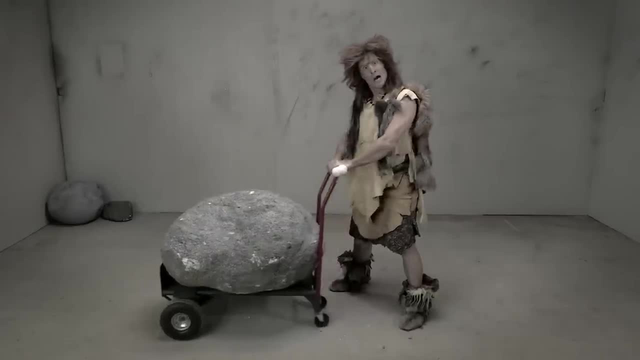 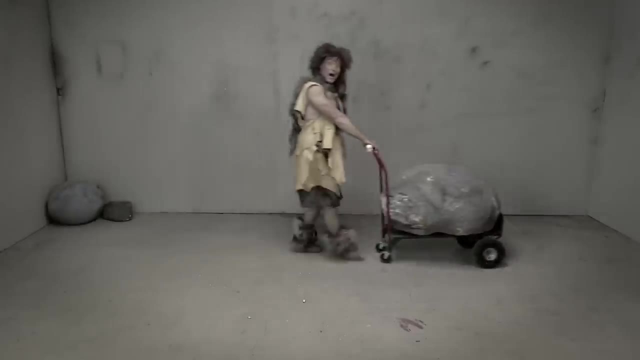 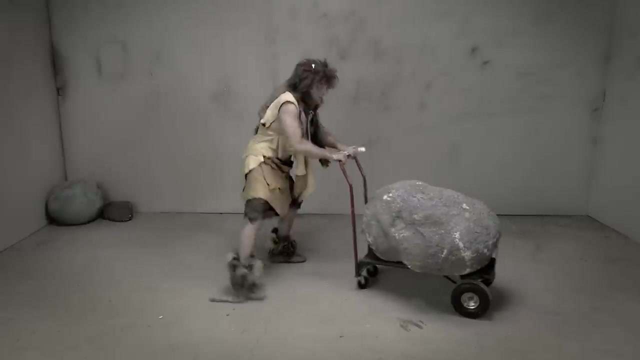 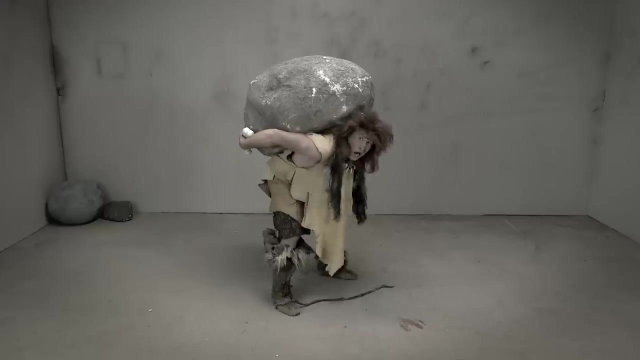 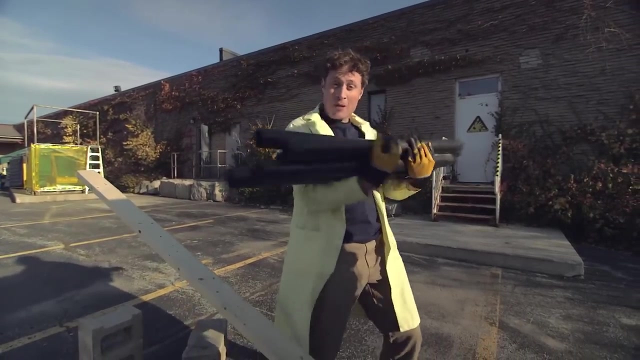 Now you have something to place that heavy rock on to move it around. But All these great inventions came after the time of the caveman. caveman had to do everything the hard way. Join us next time for more science. Okay, I've got rollers. they're just plastic pipes, but they'll work perfectly. I put them. 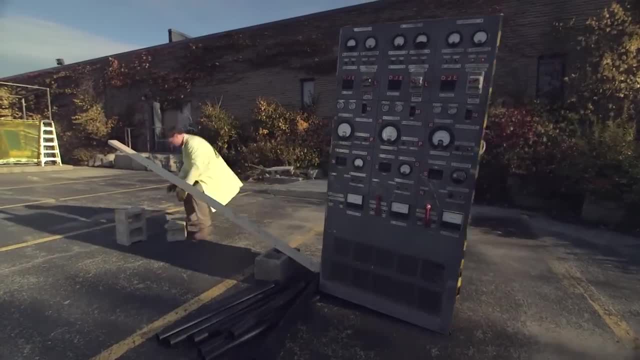 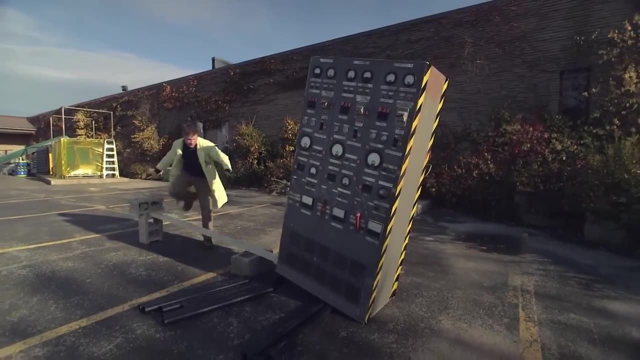 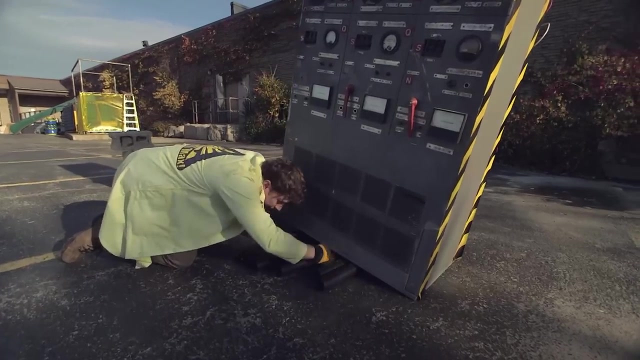 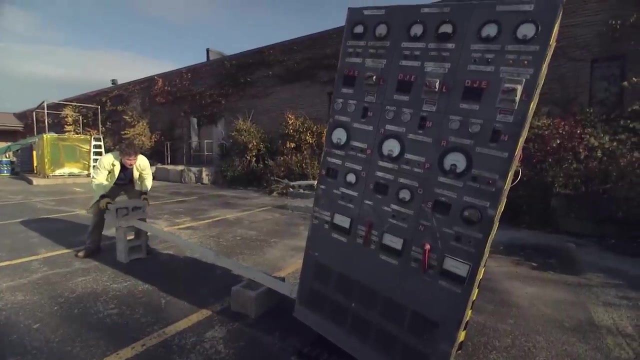 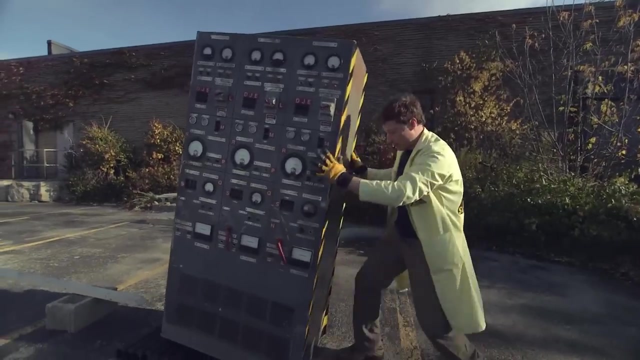 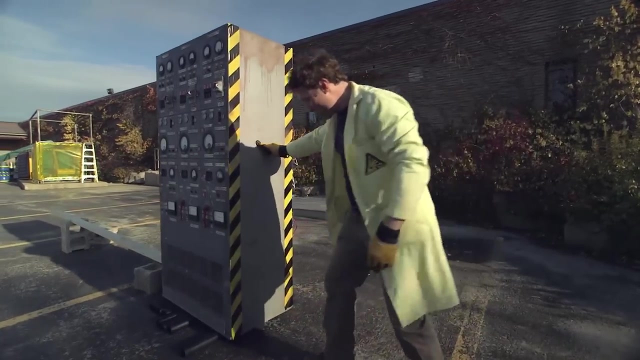 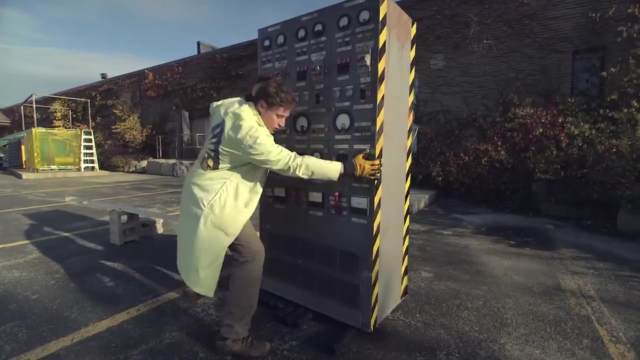 And now to lift up the machine. Perfect, and so the rollers. And then Whoa, whoa, careful, Uh-huh, Look at that, No problem, Wait, I gotta get rid of this Moving now. the trick with rollers is you have to keep taking them out of the back. 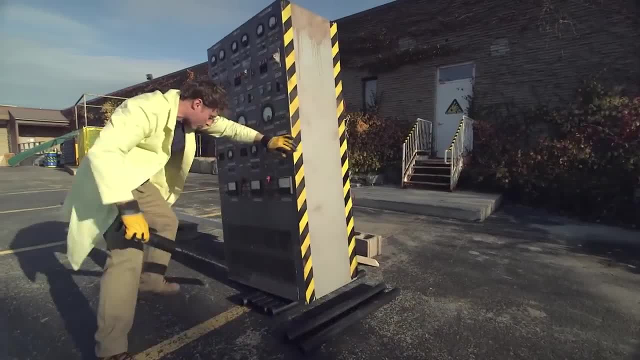 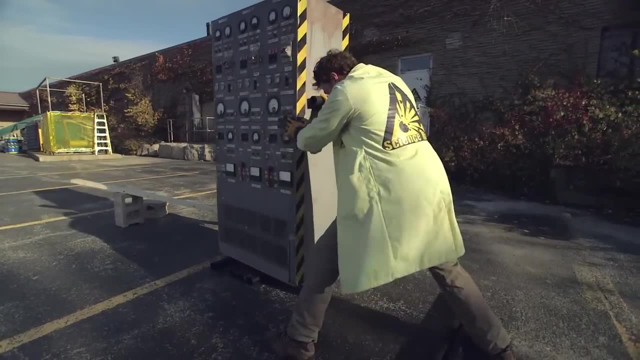 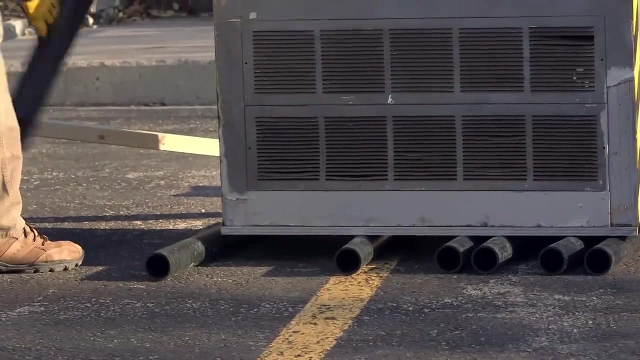 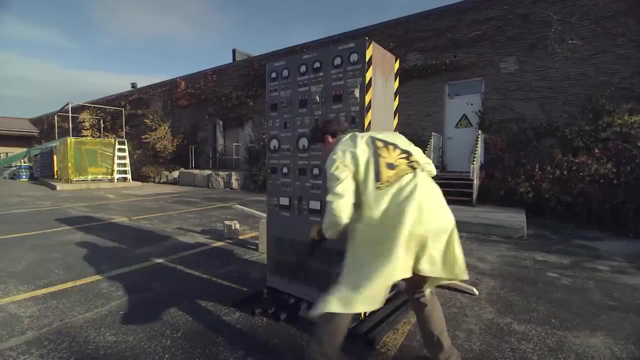 And putting them in the front. but whoa, Whoa, whoa, It's stop, rollers, stop. Oh no, Oh no, Okay, okay, Whoa, Rollers, easy, There we go in the front, roll it forward. Now I know what you're thinking. you're thinking this seems like a lot of work, and it's true, moving the rollers back and forth and back. 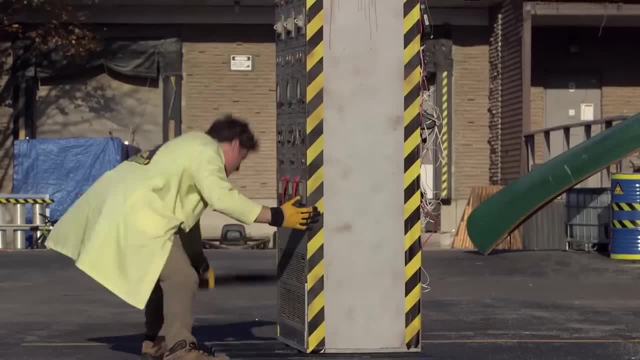 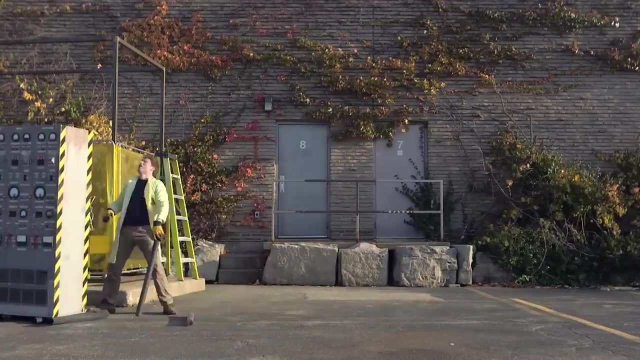 back and forth does take some time, But did you know? this was how the pyramids were built. It's true, giant stone blocks were moved on rollers, just like I'm doing here, And, as you can see, what worked for the ancient Egyptians. 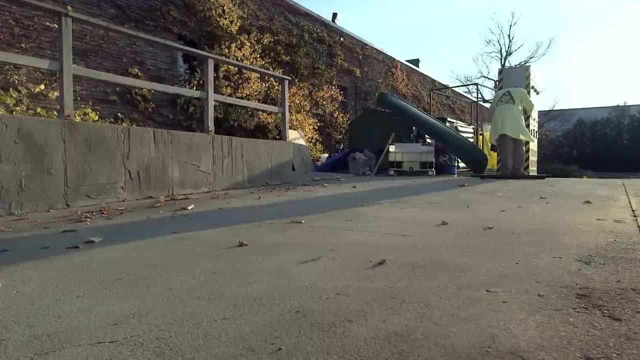 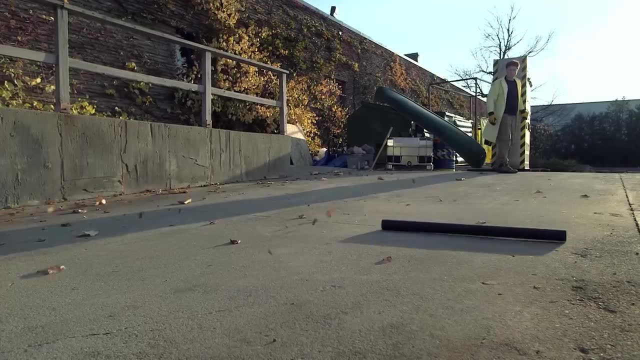 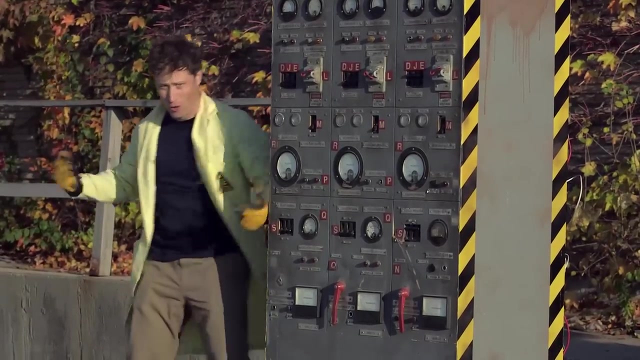 works for me too. Uh-oh Yeah, there's a hill here. If I go down the hill, it's going to start rolling faster than I can do the rollers. I'm going to need some help. Um, uh oh, I know. pulleys, pulleys, pulleys. 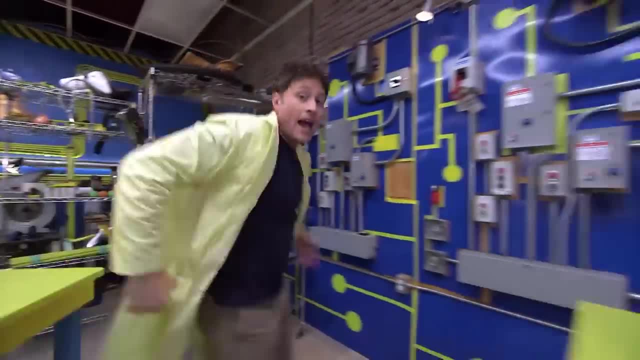 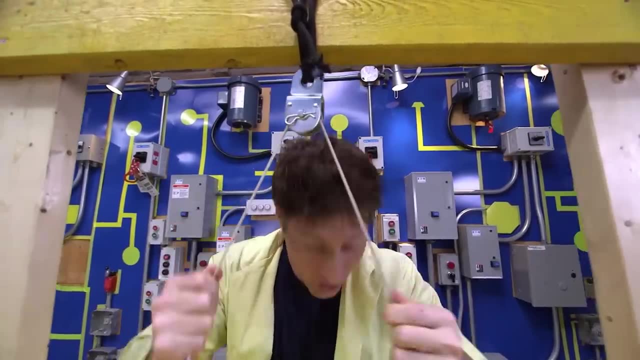 OK, pulleys. Pulleys are a great way to get your hands dirty. Pulleys are a great way to get your hands dirty. Pulleys are a great way to change the direction of force. I've got a rope going through this pulley and down to a book. 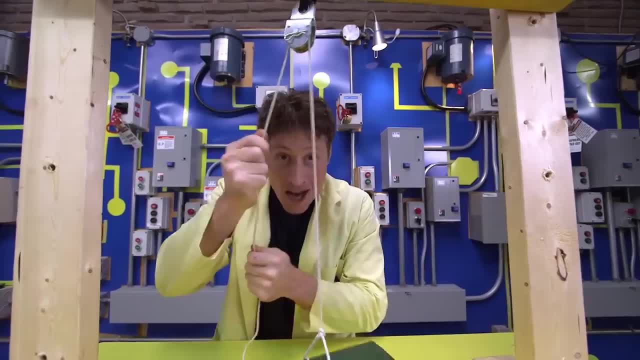 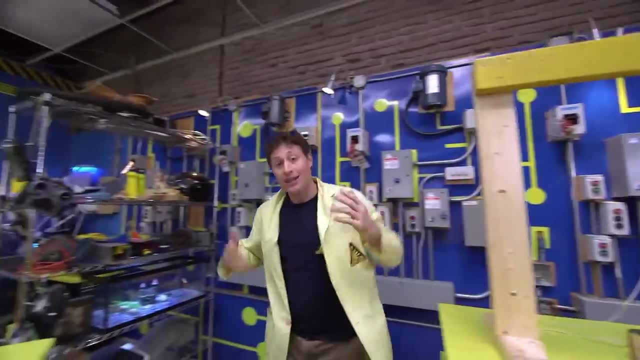 So when I pull the rope down, the book goes up. Changing the direction of force can be very helpful, But pulleys can be helpful in another way. Pulleys can let you lift something that you couldn't normally lift. Now the rope goes up and down, and up and down, and up and down. 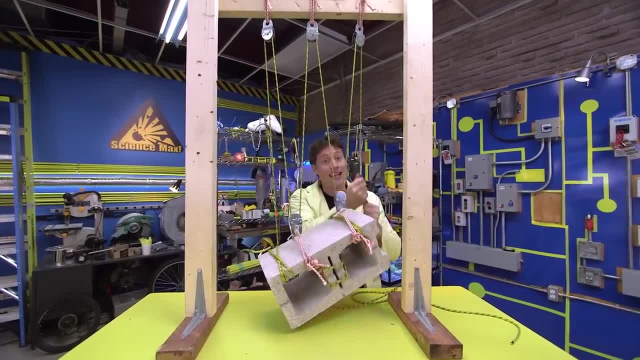 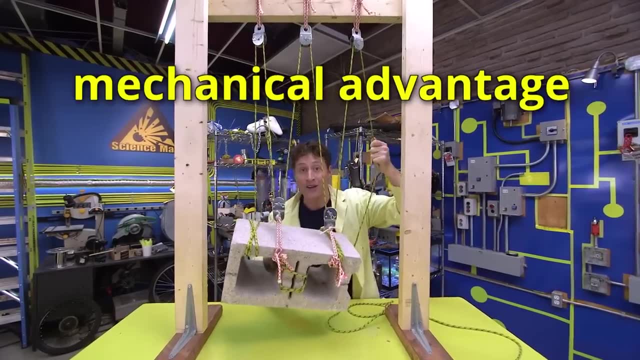 And the force I need to lift this cinder block is a lot less than if I was just lifting it by myself, But I've got to pull a lot more rope. That's called mechanical advantage: Spreading out the force over a longer pull. 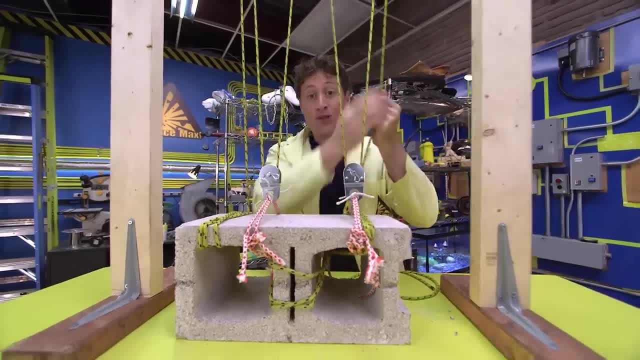 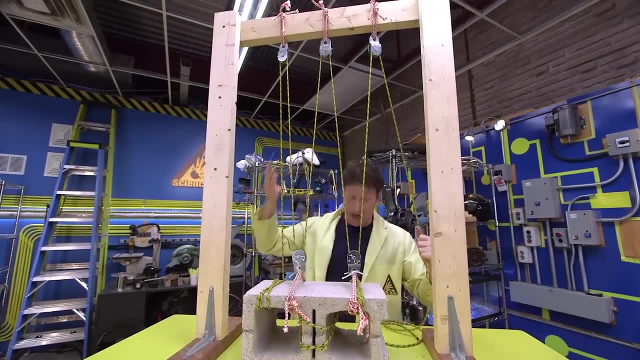 so you can lift a larger weight. If you use more pulleys, it reduces the amount of force. One pulley, same amount, Two pulleys half the force. Three pulleys, one third. So I've got five pulleys here. 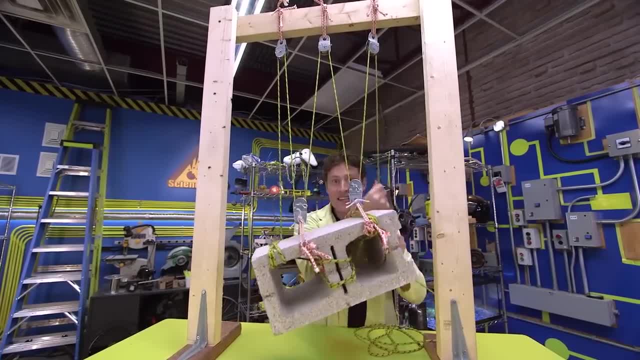 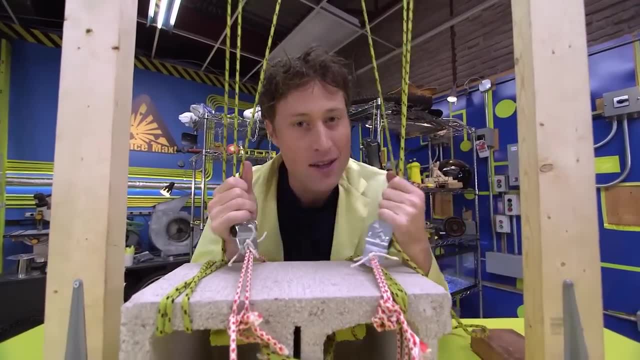 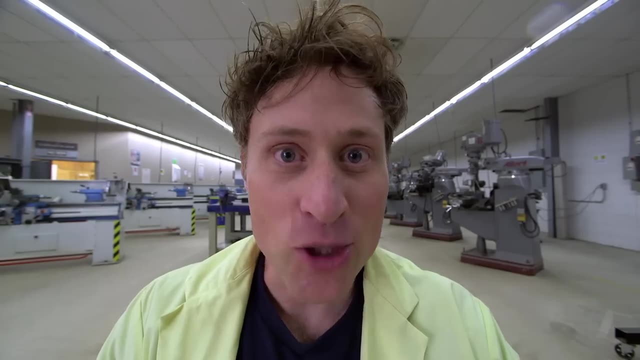 which means I only need one fifth the force to lift this cinder block. So there you go, pulleys. Now back to the Wait a minute, wait a minute. This calls for a mini-max- Mini-max. So how much weight can you lift with pulleys? 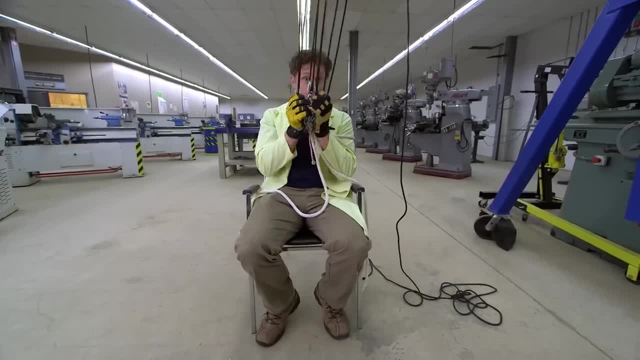 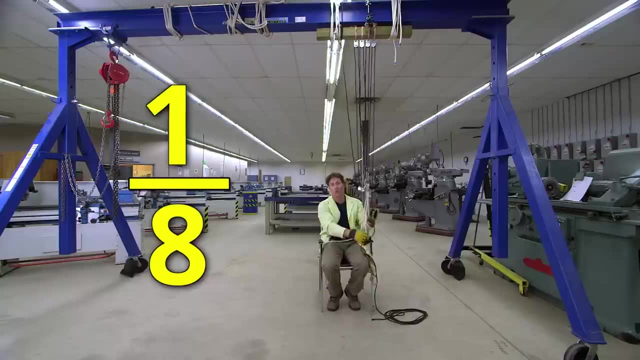 Well, as much as you want. really, I have four pulleys on the bottom and four pulleys at the top. That means with eight pulleys, I only have to lift one eighth of my weight plus the weight of the chair I'm sitting in. 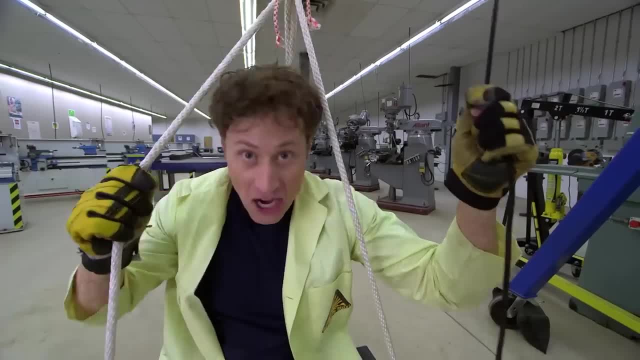 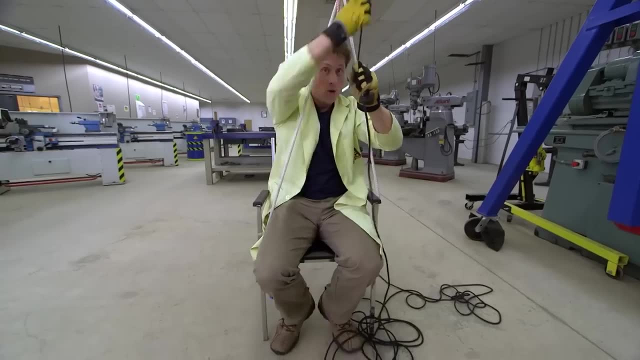 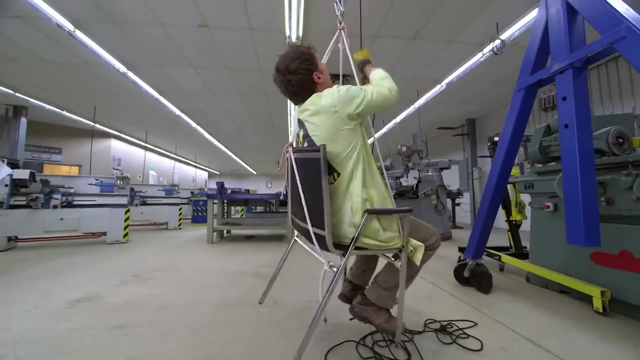 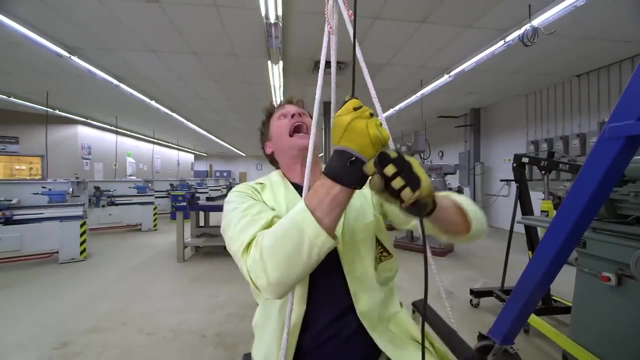 And if I keep pulling, you will see that the chair I'm sitting in is roped to the pulleys. So now we see if I can pull myself up with nothing but pulleys. Look at that, I'm totally lifting myself into the air. 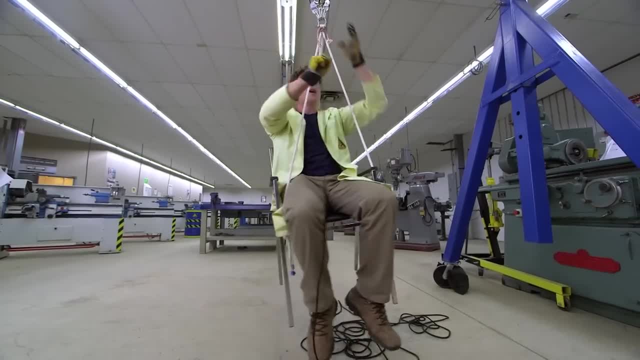 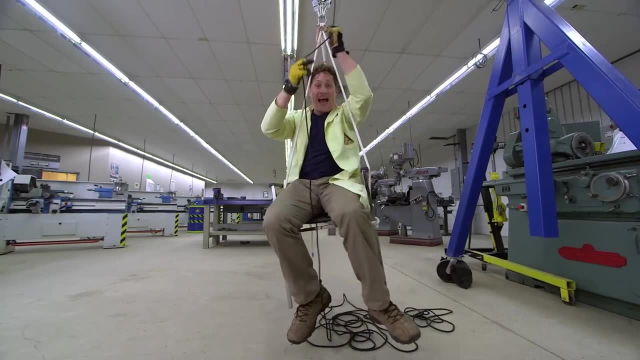 with the power of pulleys And I don't need to use two hands. In fact, I only need to use one finger to hold myself up And my thumb, obviously, to hold the rope. That is the power of pulleys. 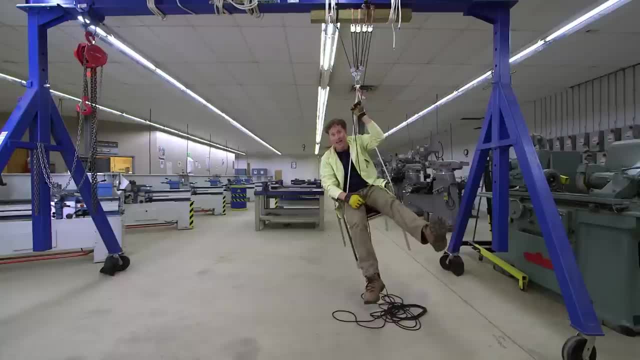 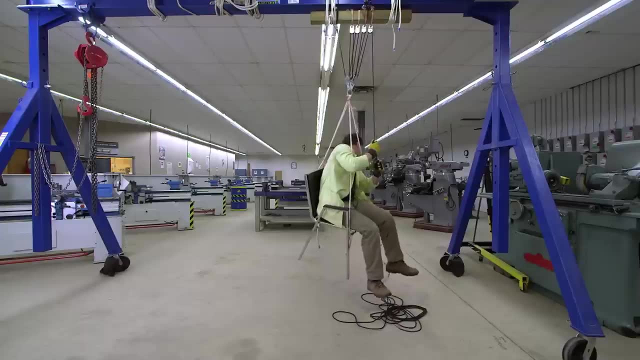 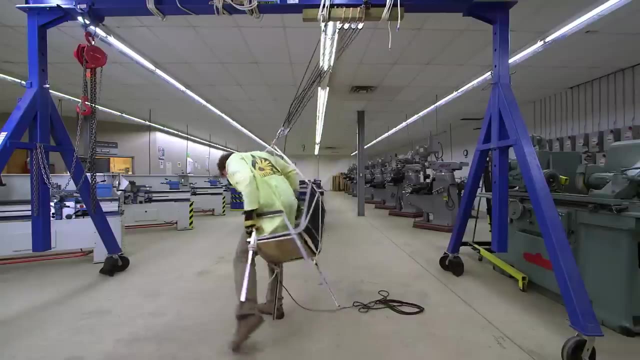 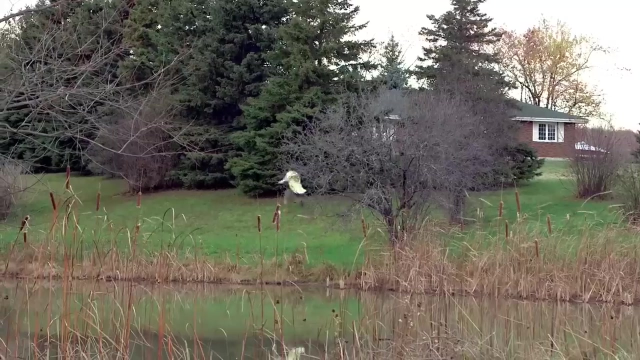 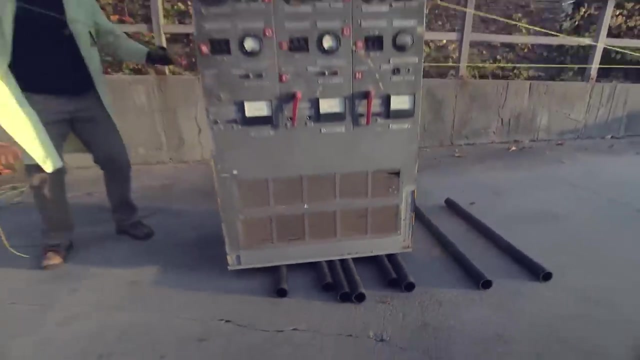 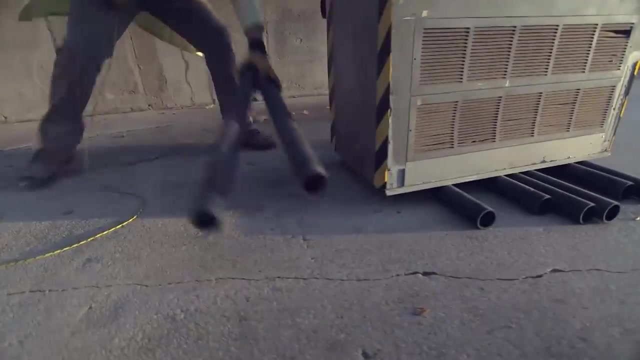 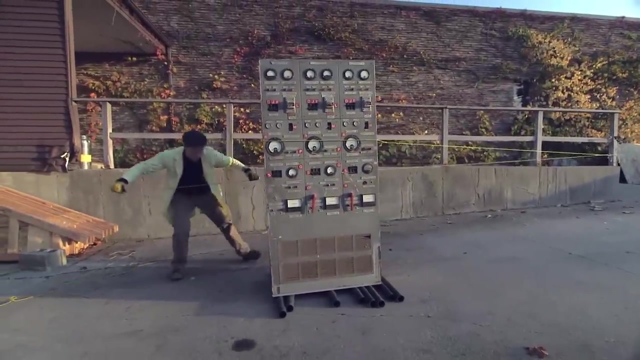 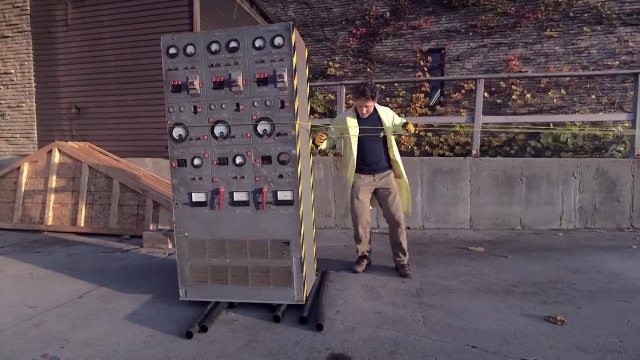 I can almost make myself fly. Well, almost. Now back to the particle impulse controller, Letting myself down. Particle impulse controller, Let's go Wait A All right, I've been able to use this pulley to lower it down the hill. 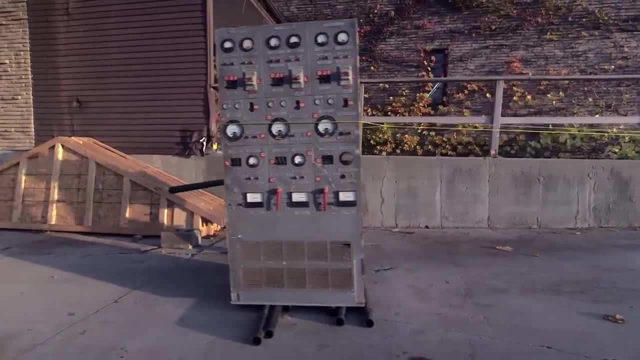 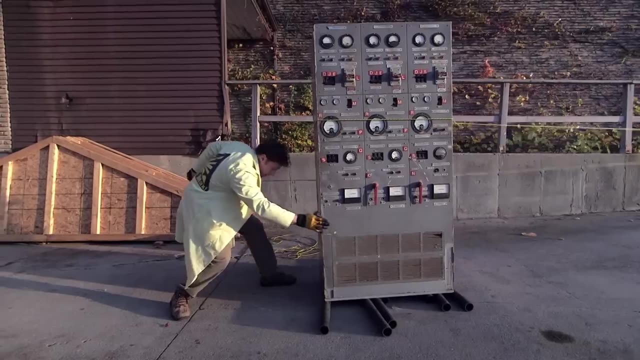 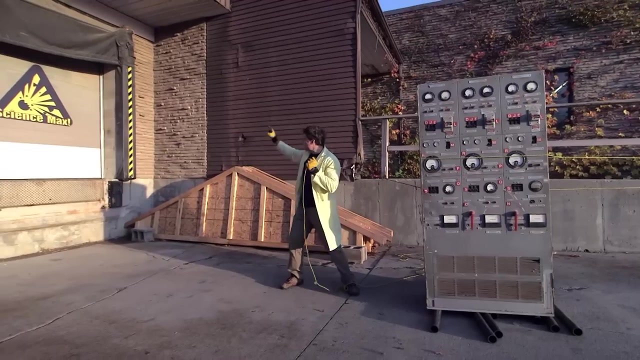 at the speed I want it at the speed I want to go. Interestingly, I'm using the pulley not to make it lighter, but to just change the direction of force, And I managed to get it right here at the bottom. Now I've got to get it up onto the loading dock. 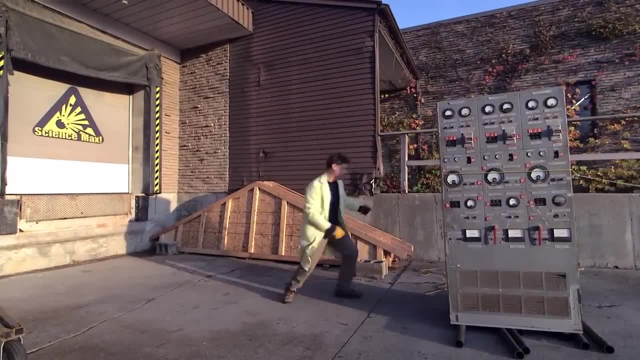 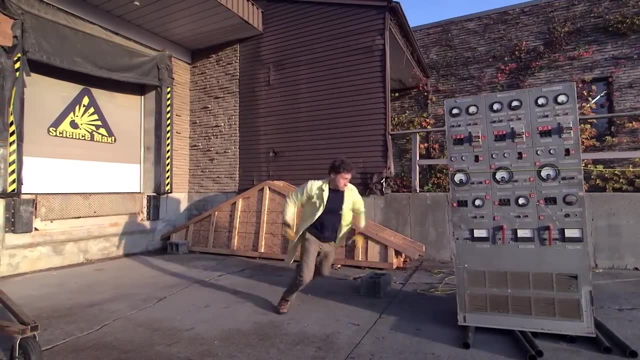 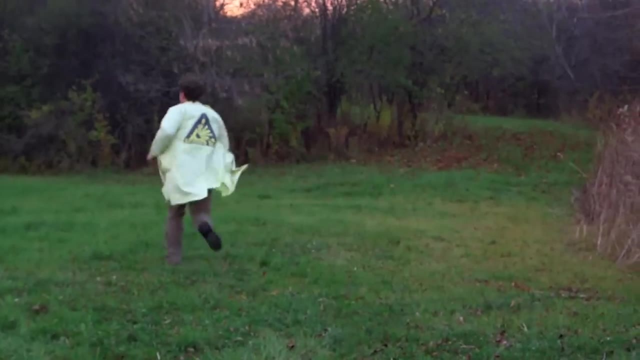 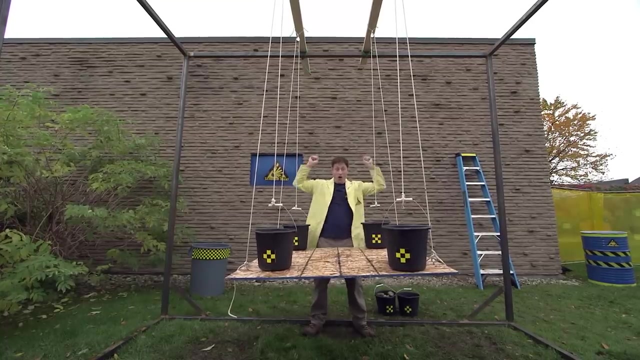 so I think this is where I need a ramp. Whoa, Whoa. Oh, Here is something mind-bending you can do with pulleys. These buckets are attached to the table through a pulley. There's nothing holding this table up. 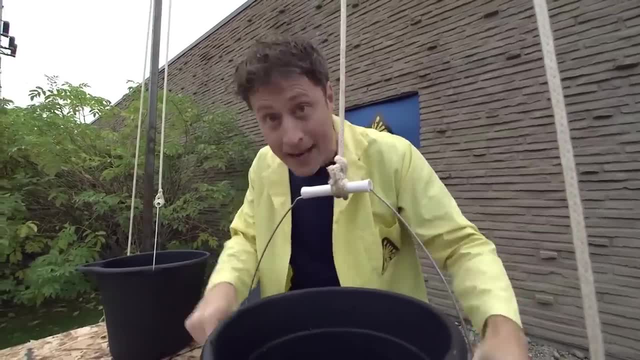 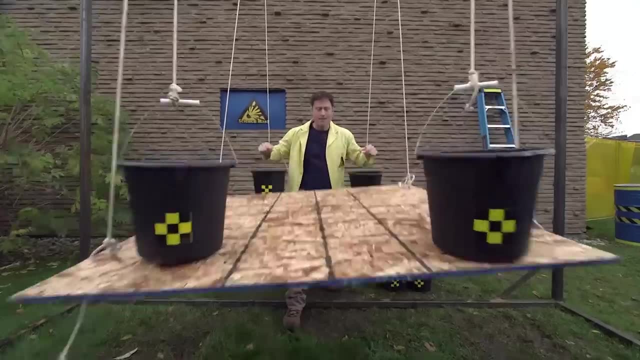 except for the weight of the buckets pushing down on the table. So if I took the buckets off the table, the weight of the buckets pulls the table up, But because of the bucket, The buckets are on the table. everything is in balance. 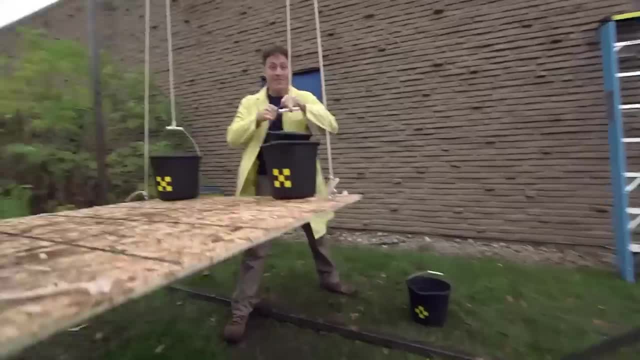 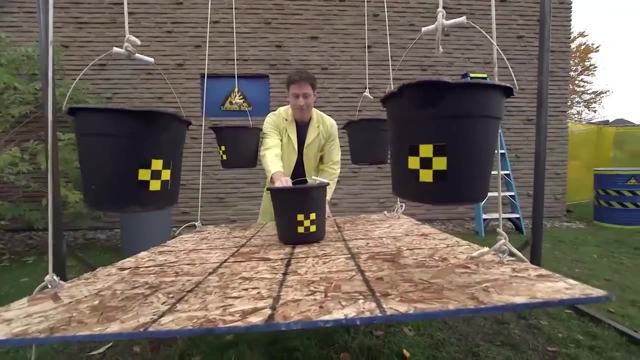 Mind-bending right. OK, wait, It gets better If I took a weight and I put it on the table. the weight of the buckets isn't enough to keep the table up, So I have to add more weight to the buckets. 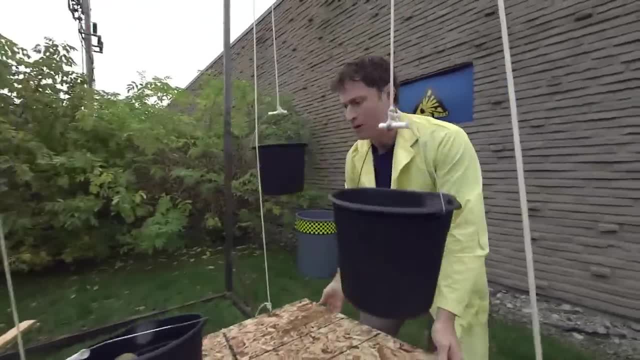 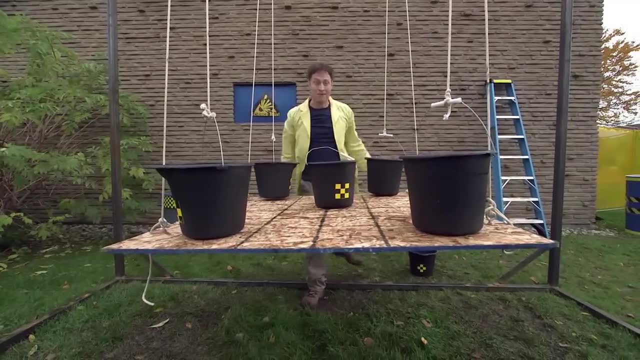 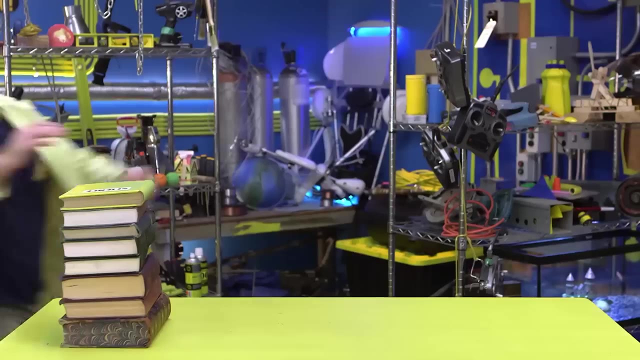 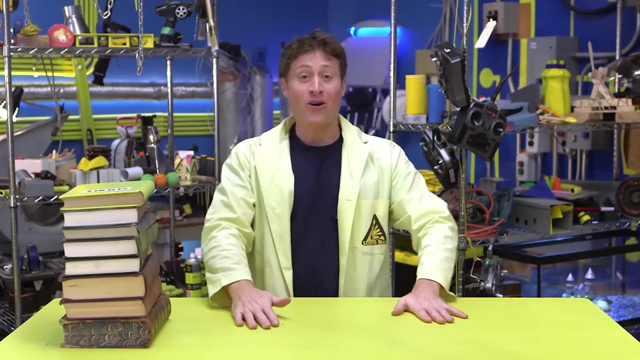 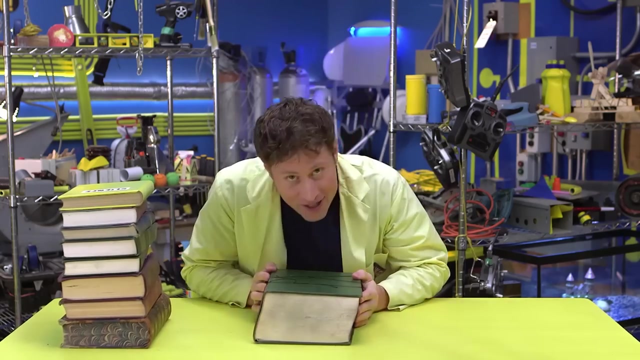 so the buckets pull the table up. Whoa, And there you have it. It's weird, It's mind-bending, It's science, OK, OK, Ramps. Ramps are a great way to move something up. I will demonstrate using- you guessed it? a book. 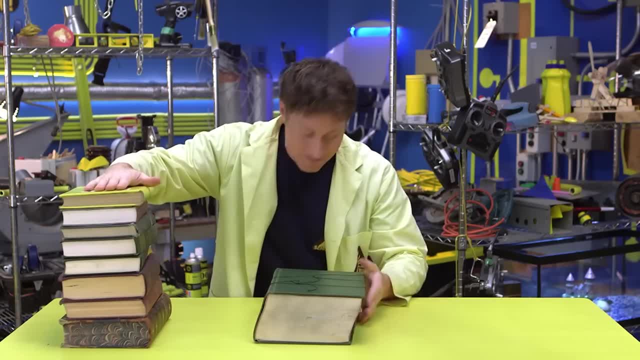 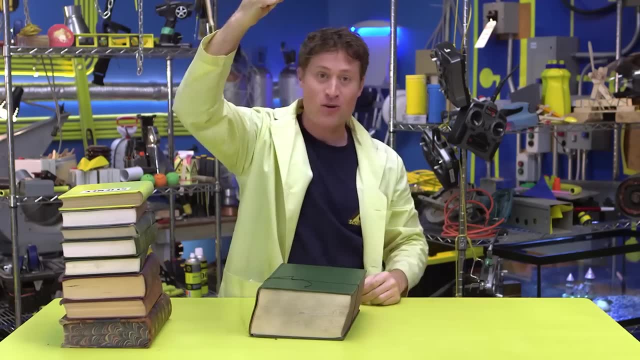 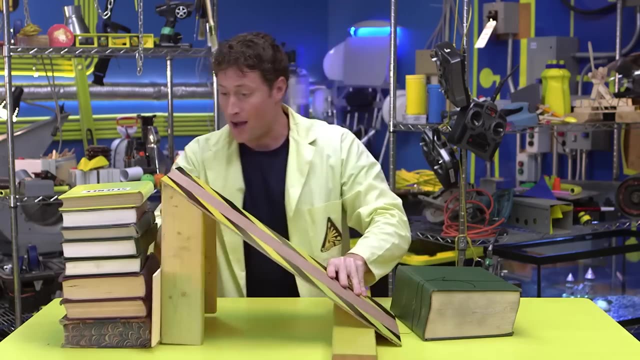 Let's say I wanted to move this heavy book on top of this stack of books using just this little string. Watch what happens: The string breaks. But if I built a ramp to get the book on top of this stack and I use the same kind of string, 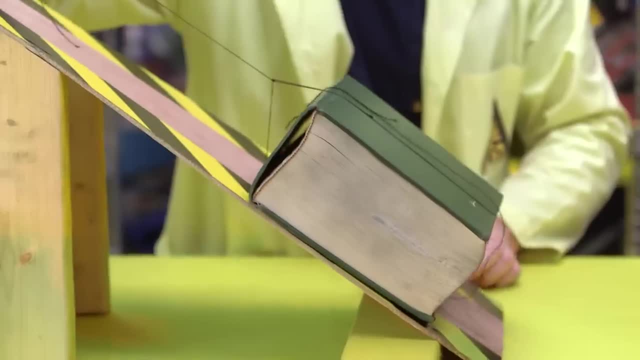 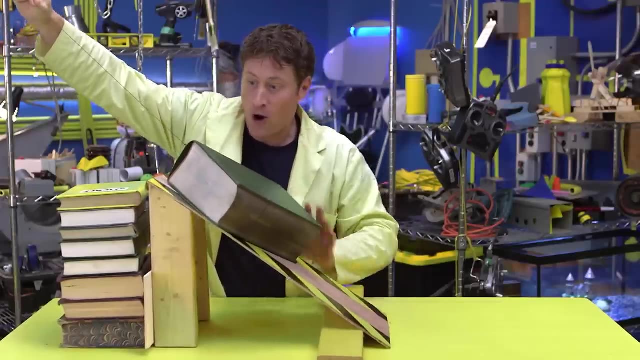 watch what happens this time. You see, the ramp distributes the force, So you use less force to pull the book over the same amount of distance and I can go, And I can get it up to the top of the stack of books. 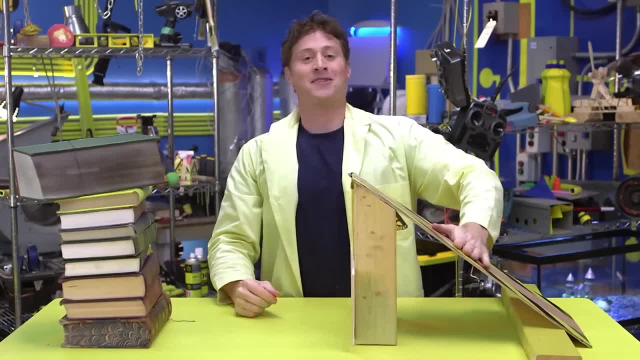 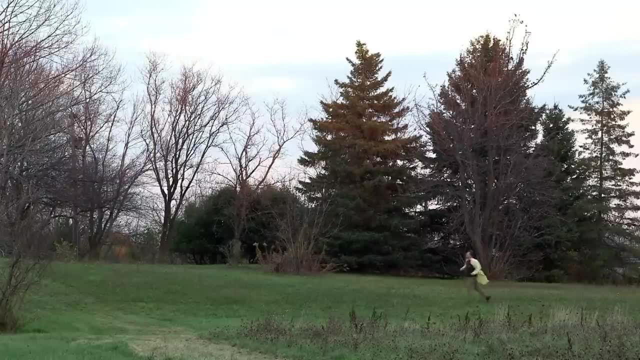 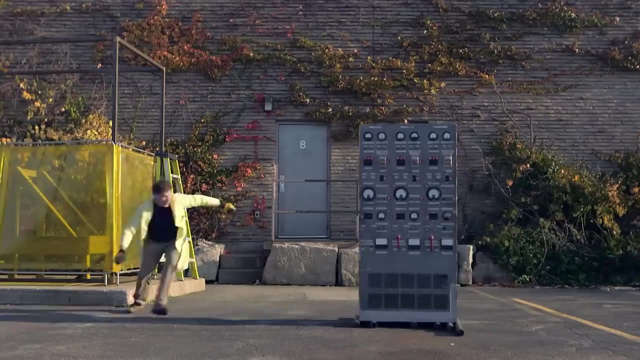 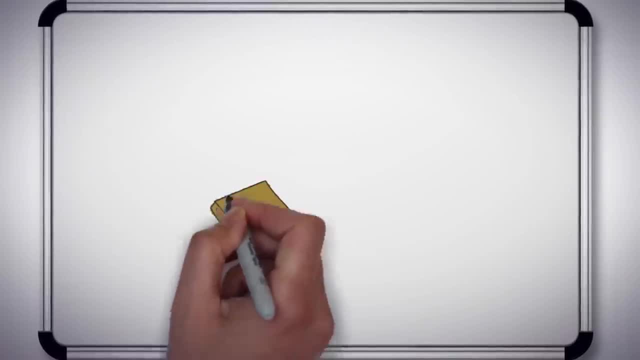 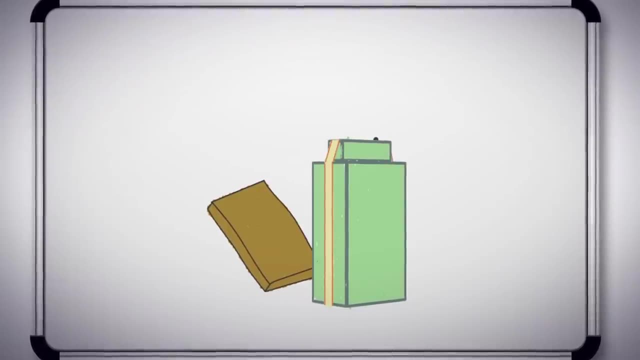 Oh, Oh, Oh Oh. Follow me guys. We're going to build a ramp that goes from the ground up to the loading dock. Then I need to pull the heavy impulse controller up the ramp. The best way to do that is to use a system of pulleys. 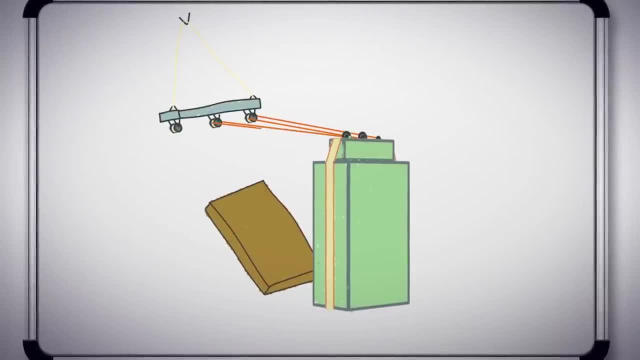 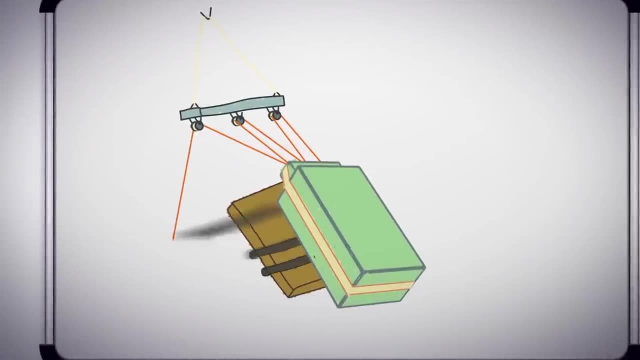 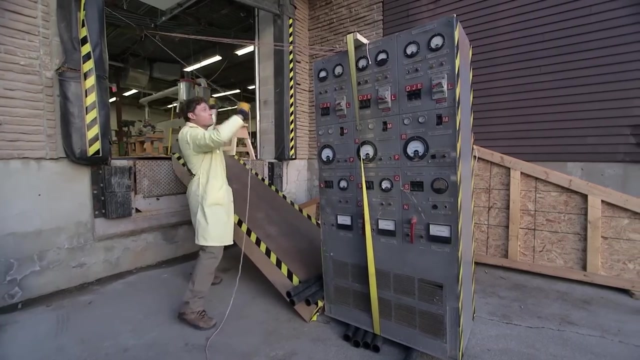 I have three pulleys on one end and two pulleys on the controller. Because I have five pulleys working together, I'll only have to lift 1 fifth of the weight. The plan is to get it tipped over onto the ramp, then use rollers to help it roll up as I pull on the rope. 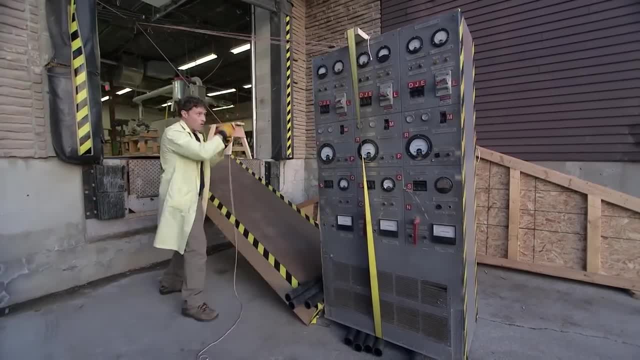 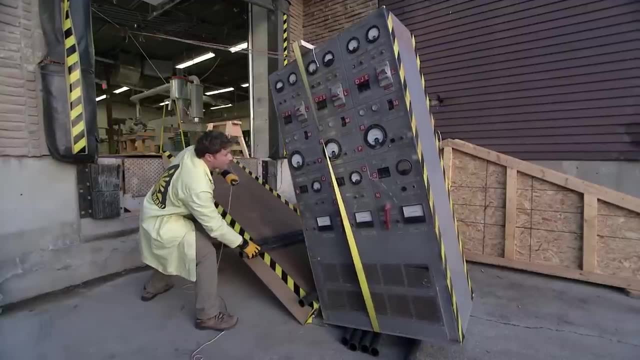 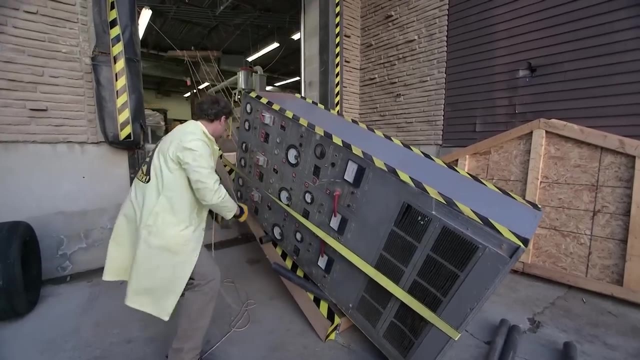 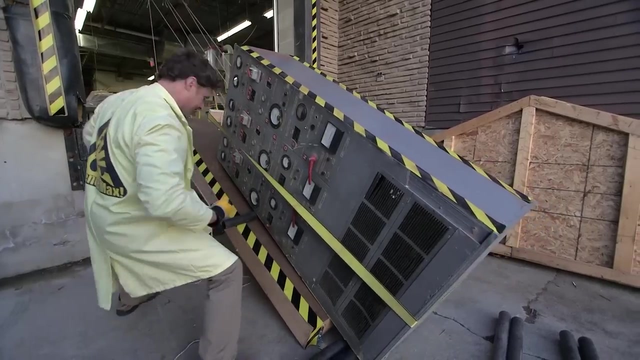 And I got two pulleys on this piece of wood here And now, if I pull and I carefully put the rollers underneath- careful, careful, Perfect, OK, now it's on the rollers And now I can pull it up the ramp.